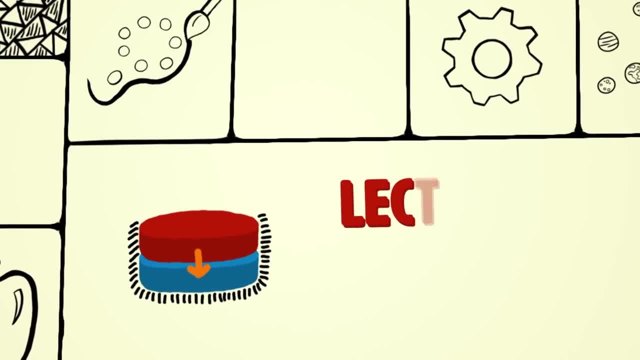 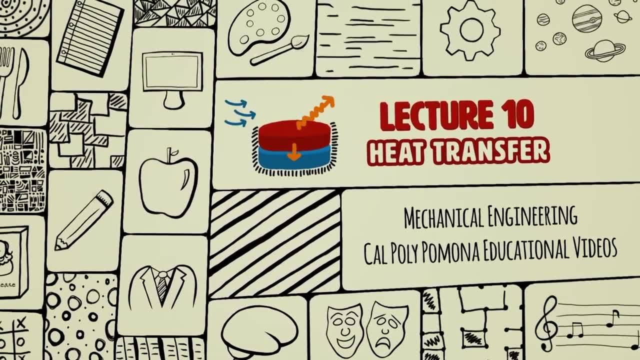 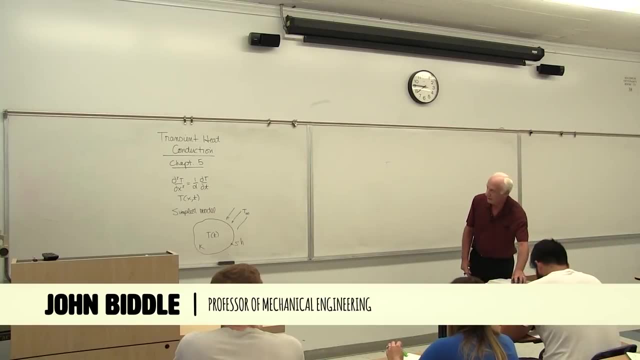 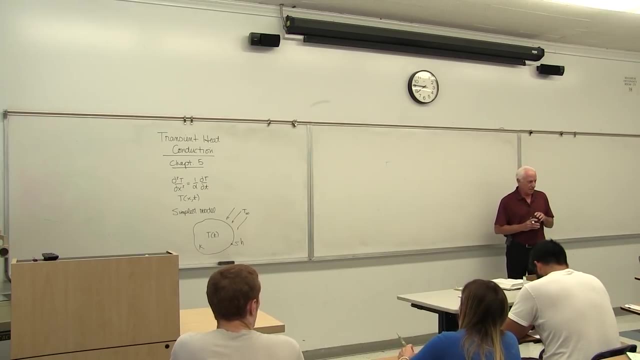 Okay, we are starting the last chapter in conduction: heat transfer. We'll be starting, probably we'll finish up Friday. We'll probably start radiation heat transfer on Monday of next week, chapter 12.. Now chapter 5, everything we've had so far, pretty much, except for some graphing we did, pretty much was steady state. Well, chapter 5 says: all right, now let's let things vary with time. 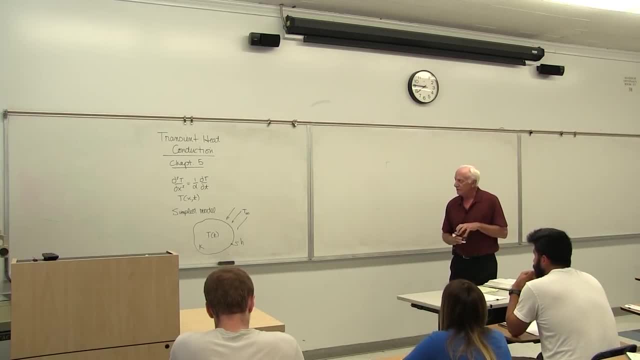 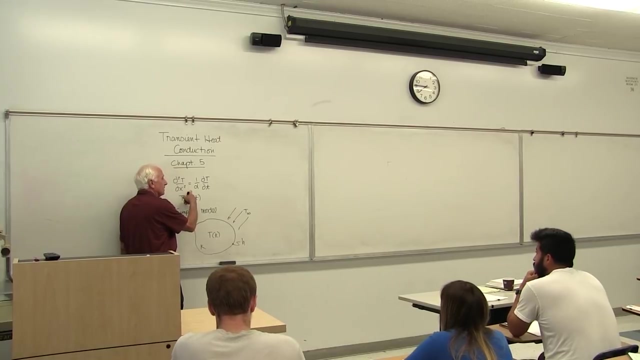 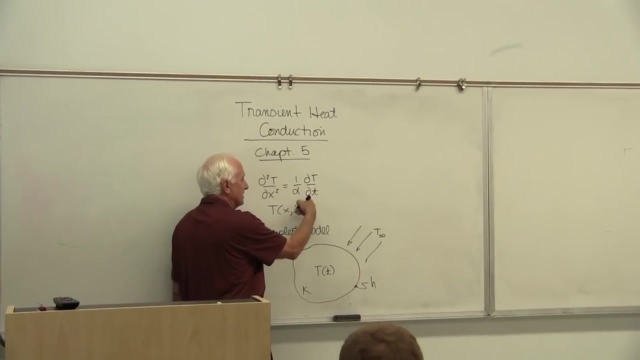 And you can see the differential equation there, the general one for 1D: transient conduction, no generation, constant properties. This one 1D piece of punctuation: no generation, The constant properties. the k comes outside the second partial divided through by k, usually alpha, But it's not steady state, it's transient. 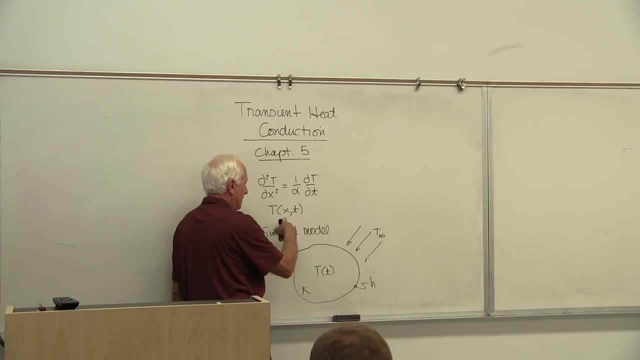 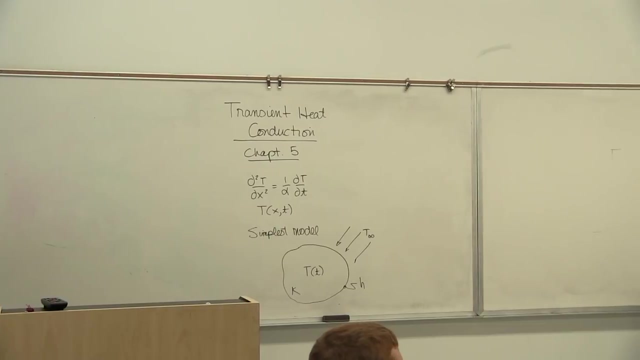 Temperature in general is a function of a coordinate like x or maybe the radius r and time t. There's a couple ways to solve these problems. If you're lucky, there's an easy way, and then, if you're not, you have to do it the harder way. 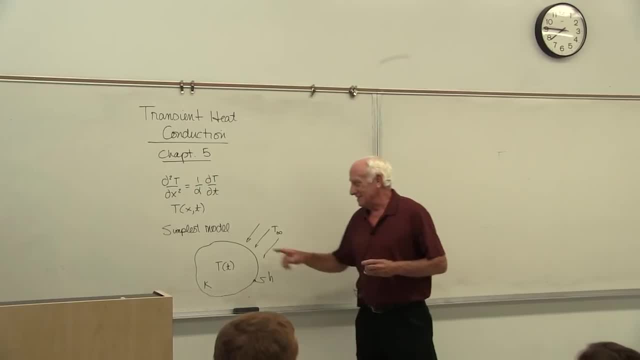 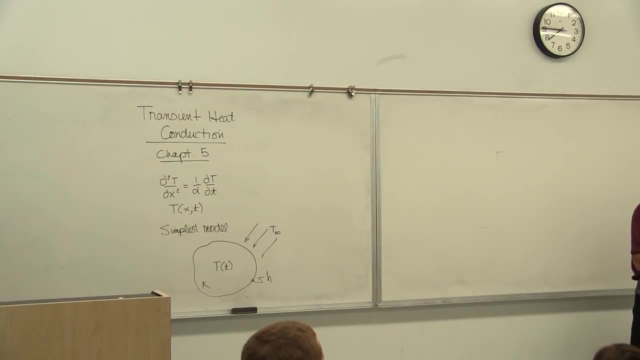 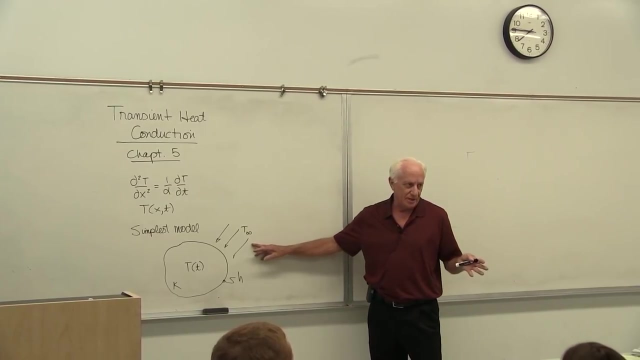 Okay, the easy way. The easy way is a simple model. Here's what we're doing. We're taking some object at a certain temperature. let's say it starts out hot. This is for It starts out hot, We blow a cold fluid over it. maybe it's air. let's just say air, We blow air over it. 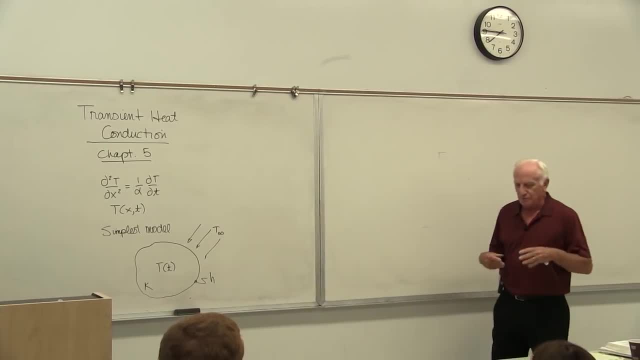 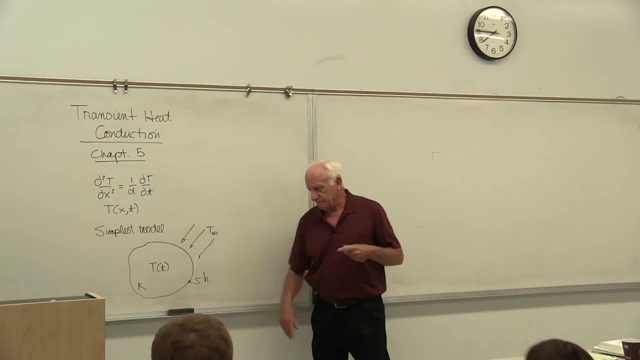 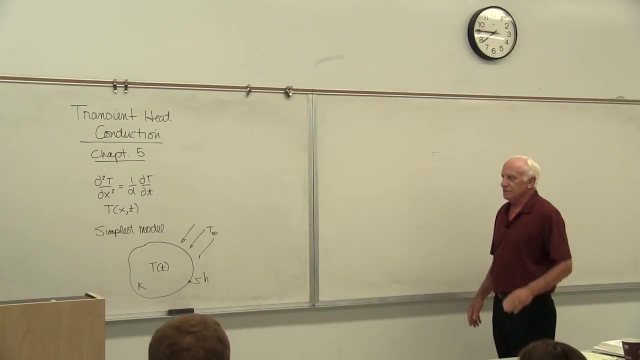 There's a convection coefficient on the outside surface. The object starts to cool. It starts to cool and the longer you wait, the cooler this object gets. But the assumption we make is that temperature is not a function of x. on that picture it's. 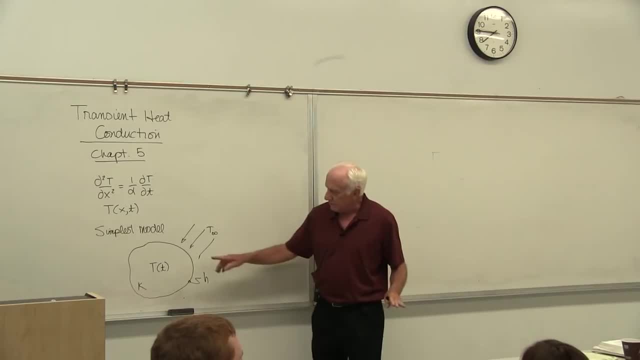 only a function of time. At any particular time, the temperature on the surface is the same as the temperature in the middle is the same as the temperature anywhere else in the body. Temperature is only a function of time, not of x. in this particular model. 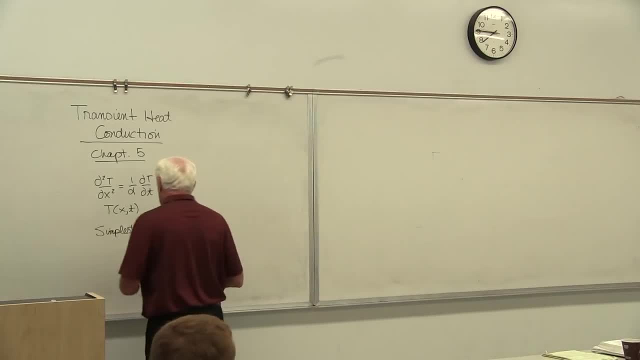 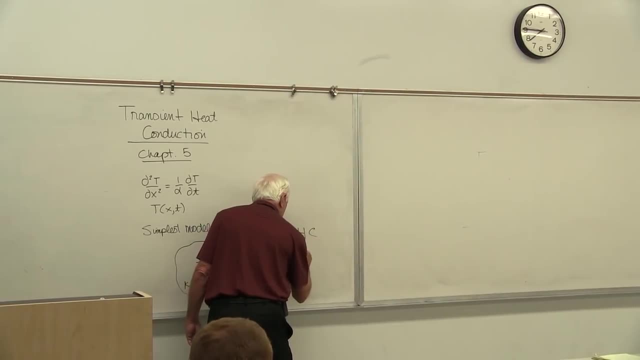 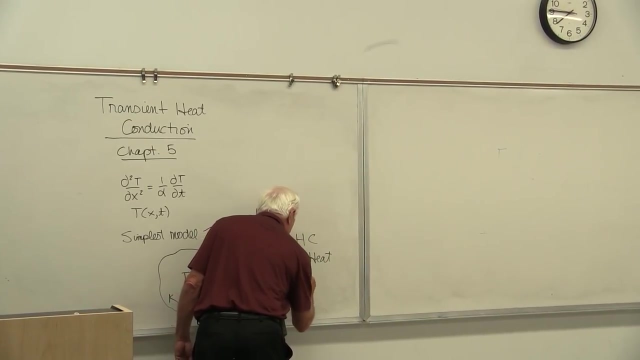 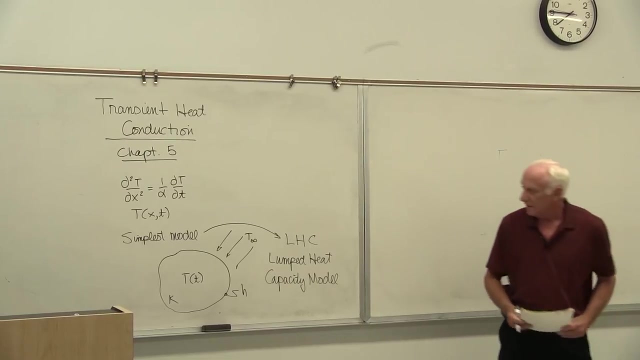 If that's the case, I'm going to tell you when it's appropriate to use it. if that's the case, this simple model is called the lumped heat capacity model, and that makes life a lot easier for us, that's true. 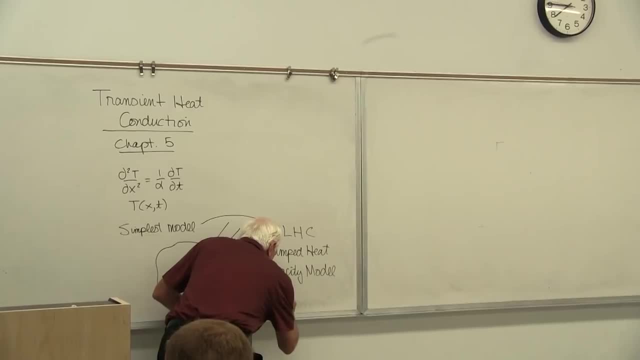 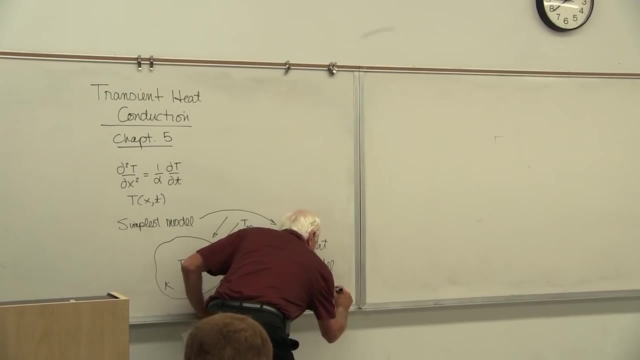 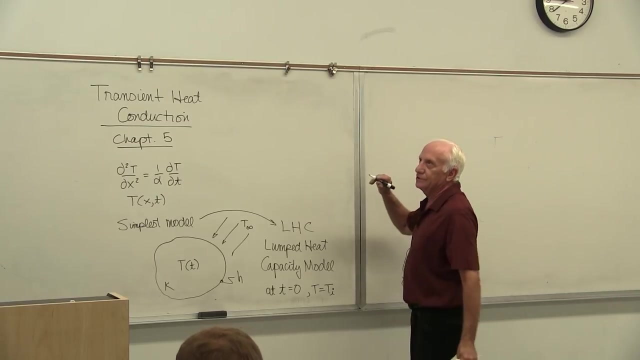 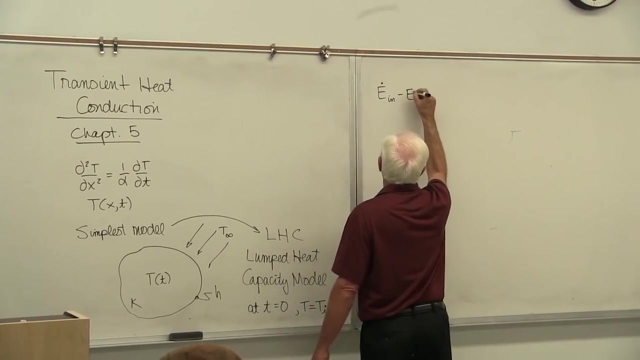 By the way, just so we know, at time equals zero, we're going to say the temperature is T-I, initial temperature. So that is our initial condition. at time equals zero, the temperature is T-I. We can go back to chapter one, control volume. around that we have E dot in minus E dot. 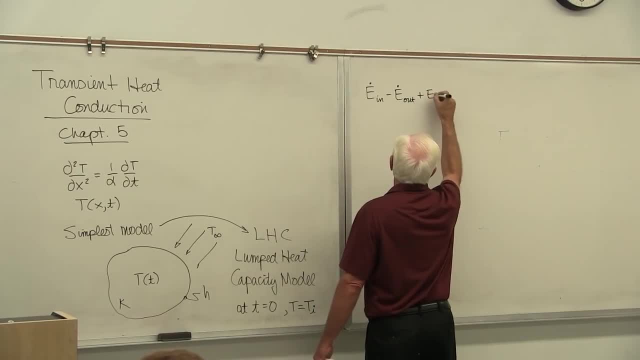 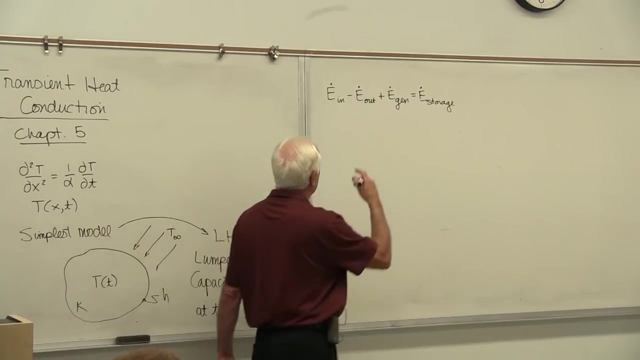 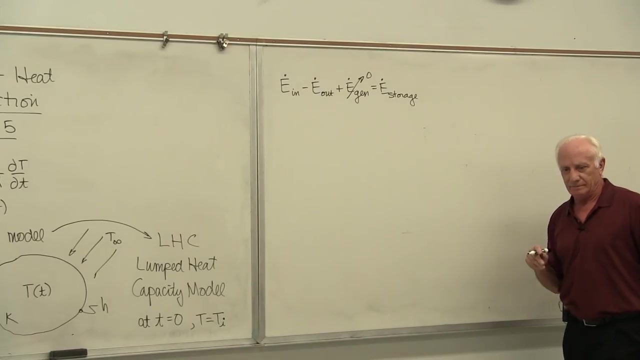 out plus E dot gen equals E dot storage, the change in storage. Okay, In this particular situation I said there's no generation. We're going to assume that the object starts out hot. T-I is a high number and T infinity. 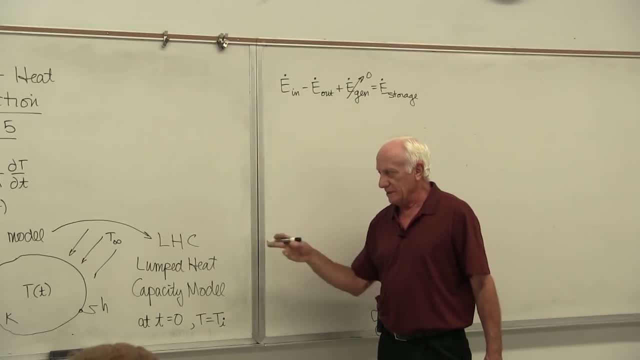 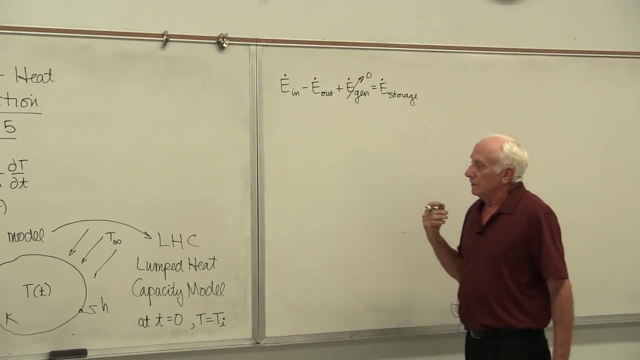 is cooler a lower temperature. So in this case it's going to be cooling with time. we could flip it around. we get the same derivation, it doesn't matter which way you build it. So heat, this is hot, Temperature is T-I. 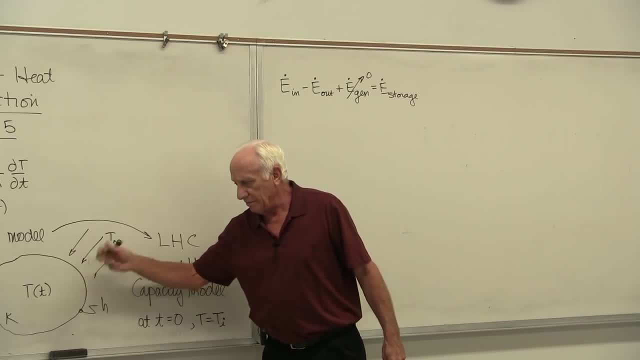 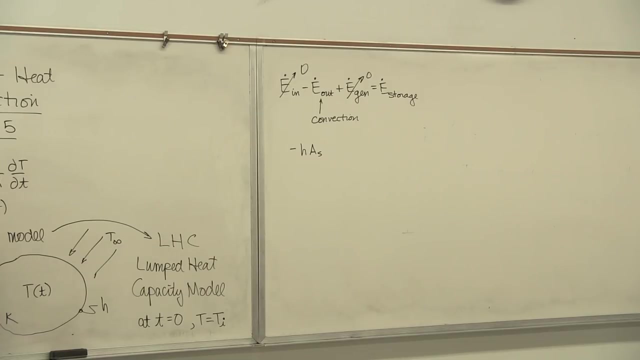 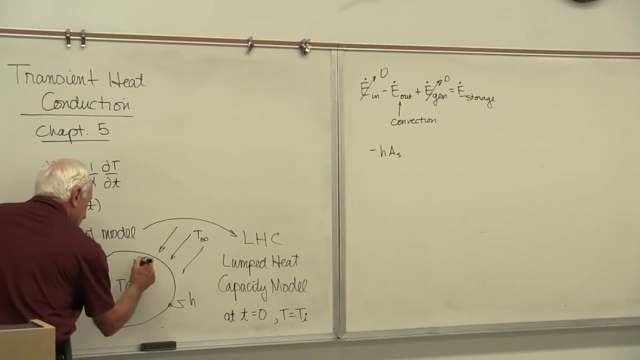 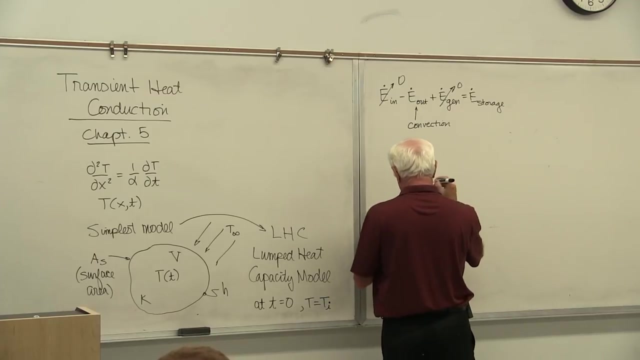 Heat. this is hot, that's cold. Heat's going out, heat's not coming in zero. This is by convection, minus H-A-S. A-S is the surface area, The volume of this is capital B, H A, S, and our temperature T minus T, infinity. 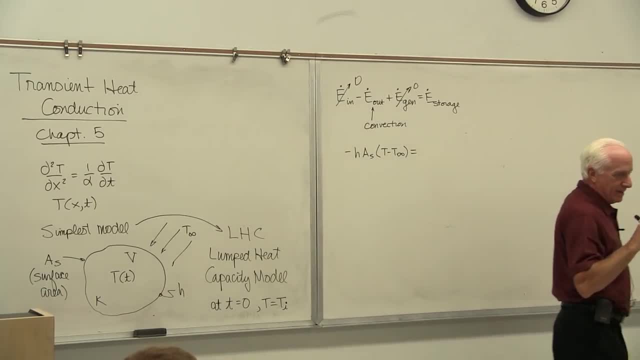 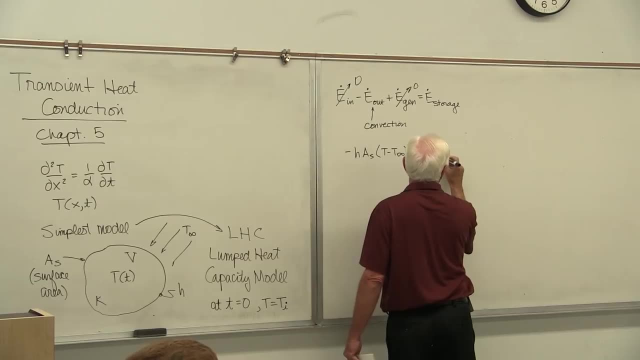 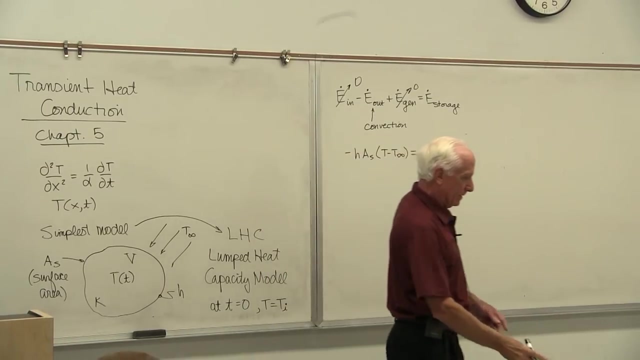 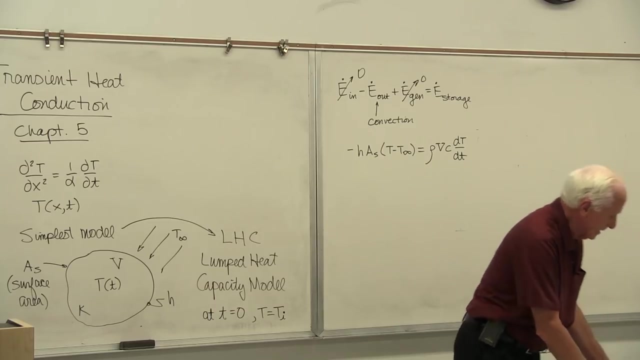 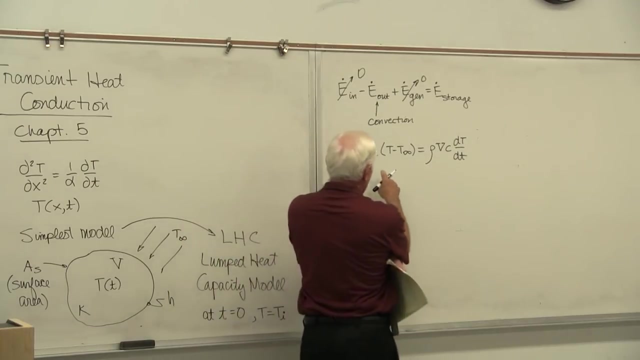 Equal storage atoms: C, sub P, delta T. The mass is the density times the volume. Specific heat: VT, V time. Okay, let's just check the units to see what comes out. We know this side is going to be in watts. 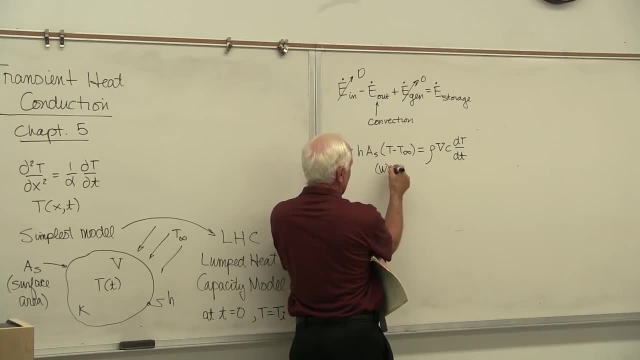 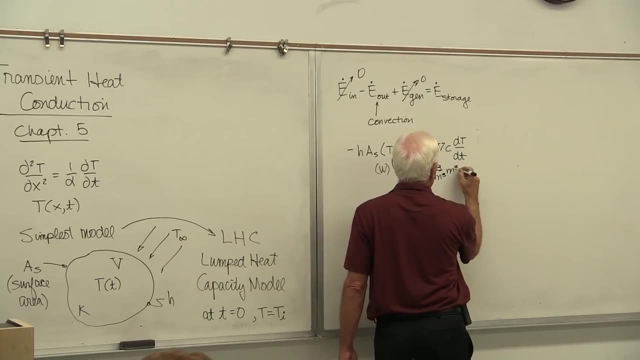 We've done that many, many times, So we know this side is in watts. Let's check this guy. Kilograms per cubic meter times cubic meter times joules per kilogram. Degree K times degree K per second. Cancel, cancel, cancel, cancel, cancel, cancel. 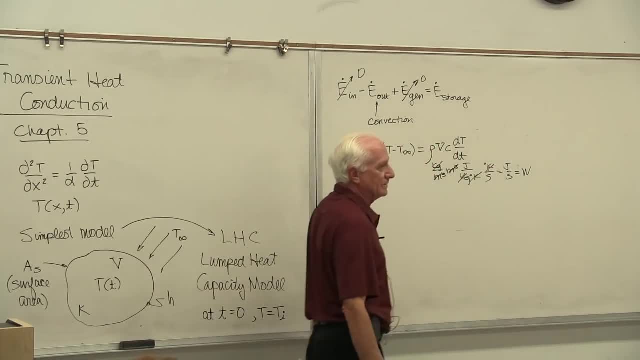 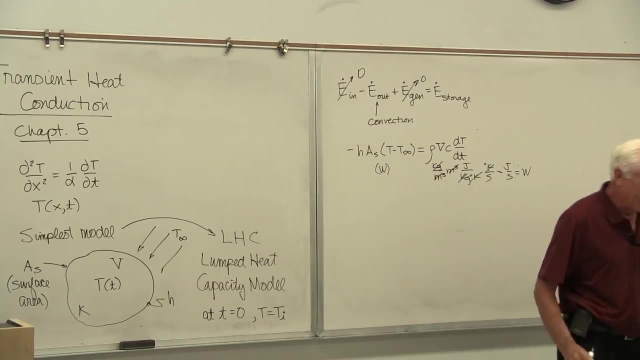 Yeah, joule per second. Yes, it is a watt, Left-hand side units equal right-hand side. But it's always a good thing to do to check it and make sure you've got it okay. Okay, so we know that equation makes dimensional sense. 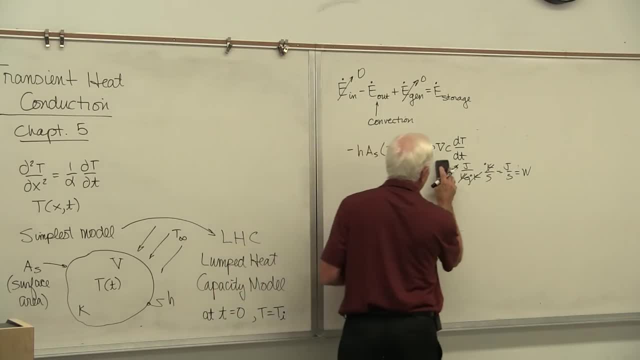 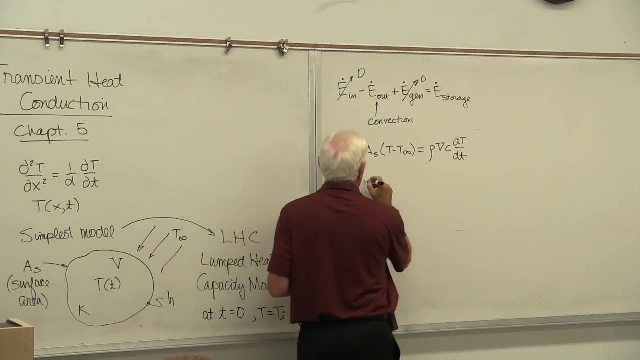 I'm going to erase that now. All right, Now we I'm going to clean the equation up as we talked about before step one: clean it up. To do that, I'm going to go through a change in variable, A new variable. theta is T minus T- infinity. 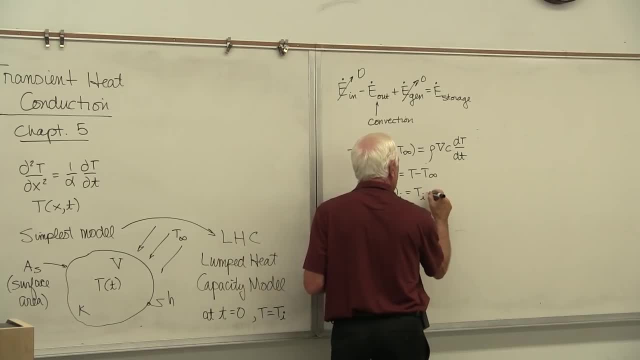 If you see the term theta I, it's TI minus T infinity. If you do this, it gives This guy over: here is theta. This is d theta dt, d, theta, dt And this is equal to minus. HAS rho, sub B times theta. 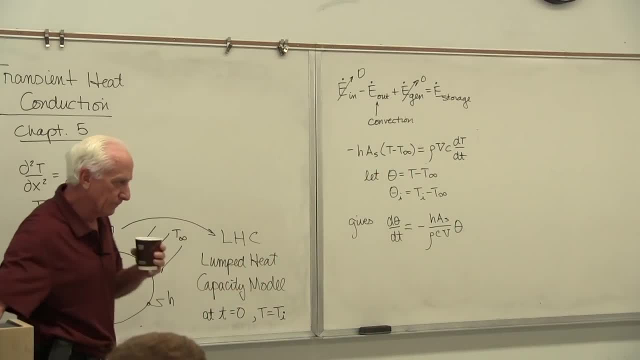 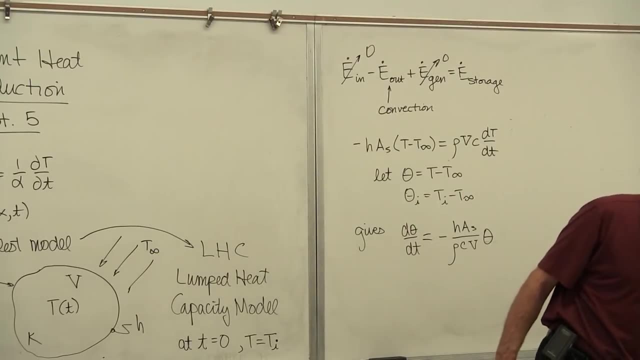 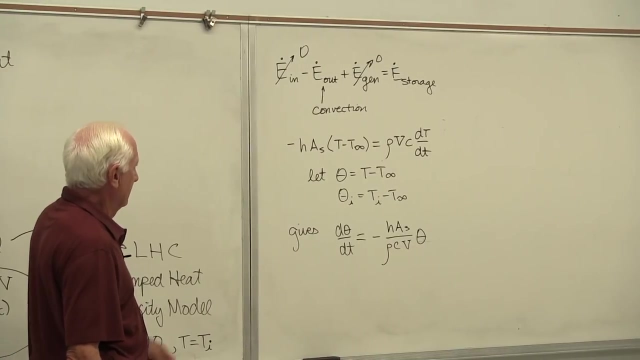 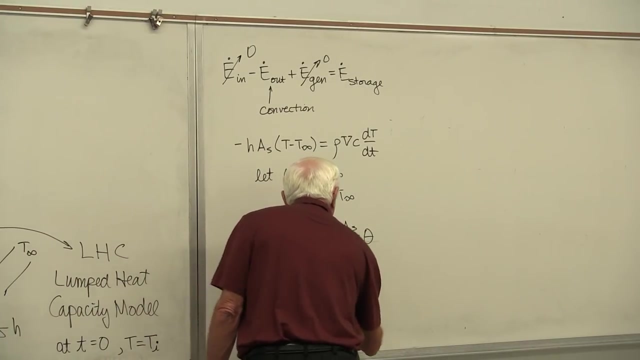 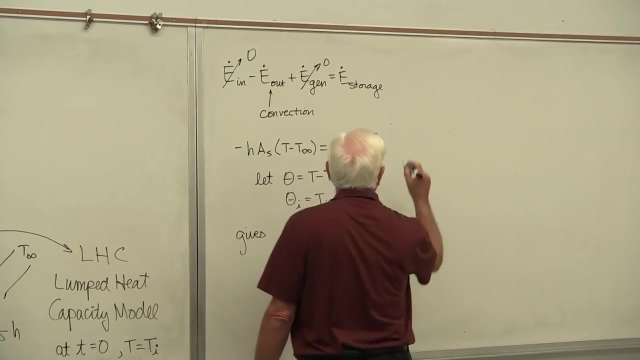 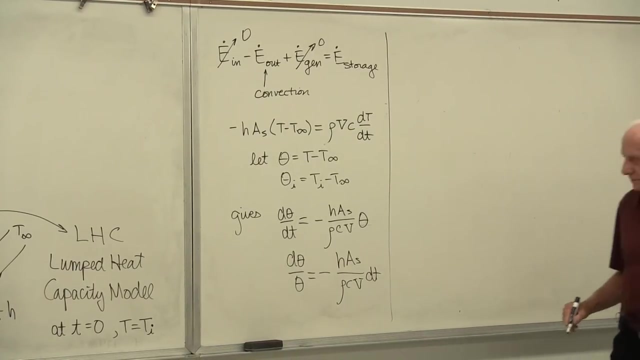 So there's the cleaned up differential equation. Okay, Separate variables d, theta over theta minus HAS, rho, sub B, dt. Integrate both sides. Integral dx over x is natural log of x, So it's a logarithmic function. And once you do that, 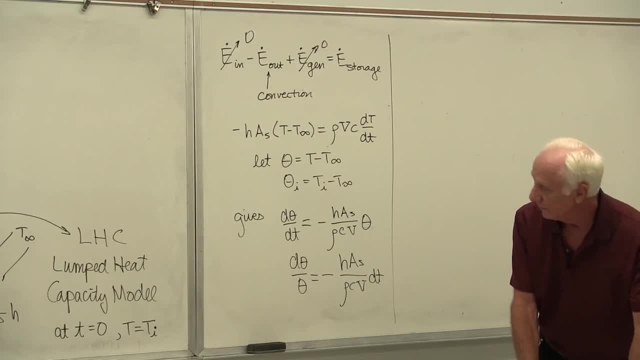 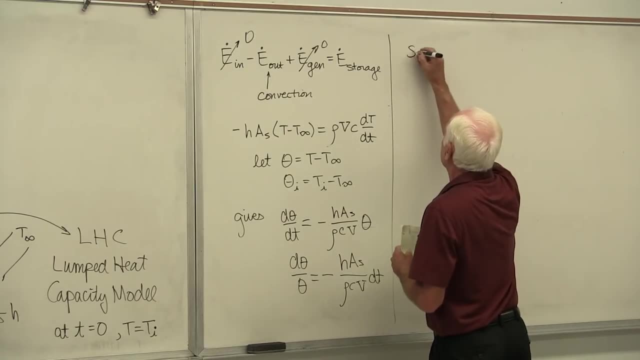 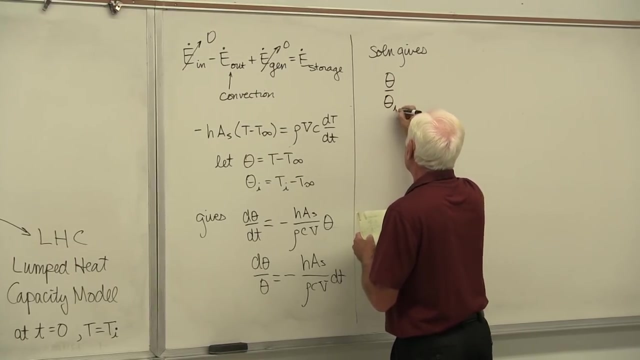 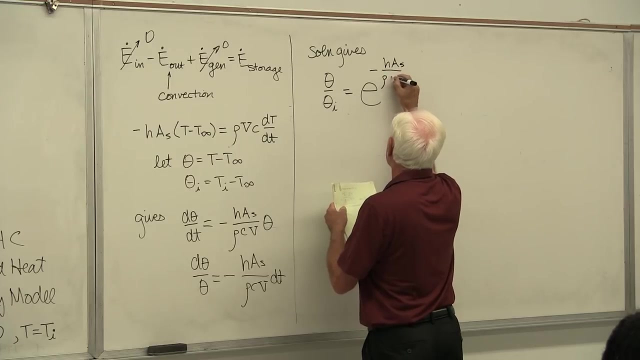 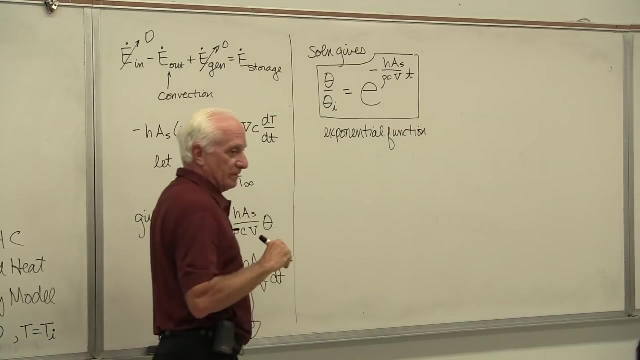 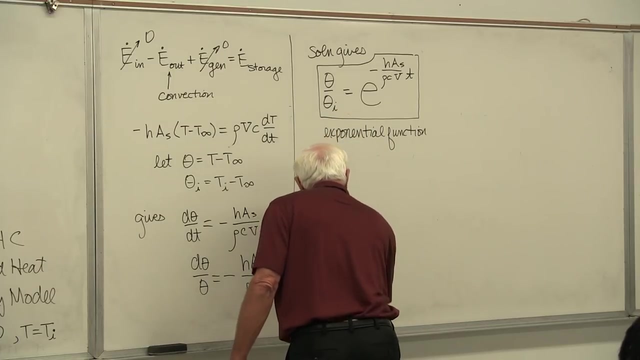 With the conditional condition: when time equals zero, theta equals theta i. Solution gives theta over theta i. This is exponential function. The left-hand side is dimensionless. Temperature over temperature difference, Temperature difference divided by temperature difference. We can then plot this where we'll plot time on the x-axis. 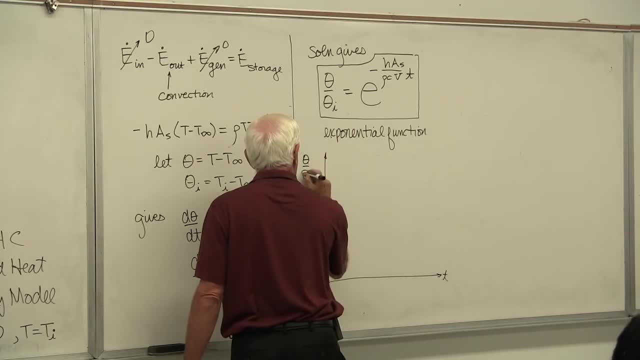 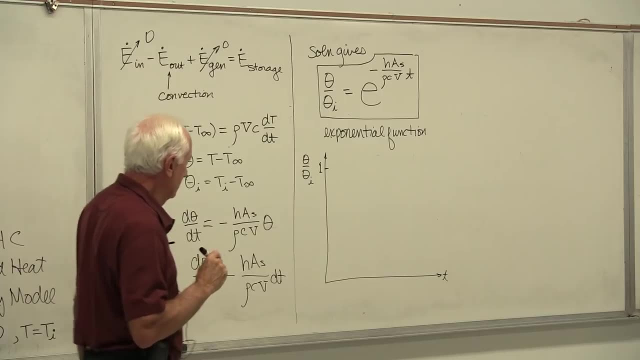 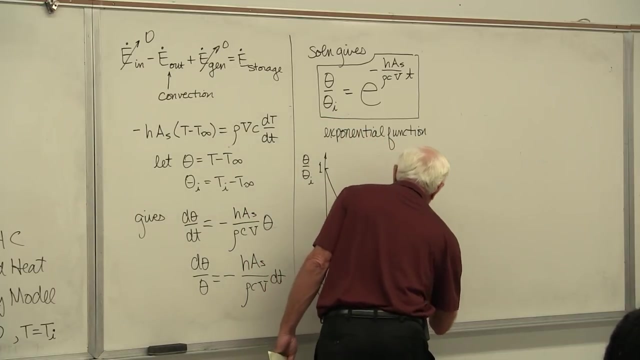 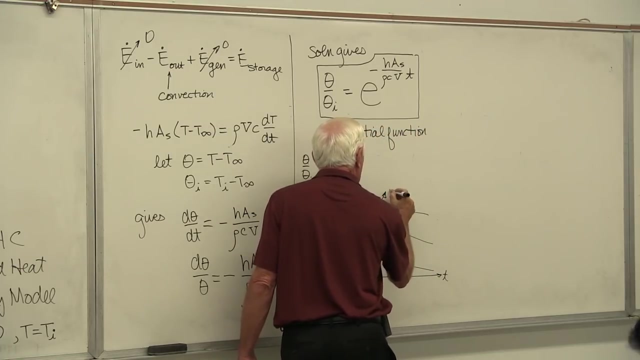 and plot theta over theta i on the y-axis. When time equals zero, theta over theta i is one. It's exponential. so it looks something like this For different values. it looks like this, And these values are something we call the time constant tau. 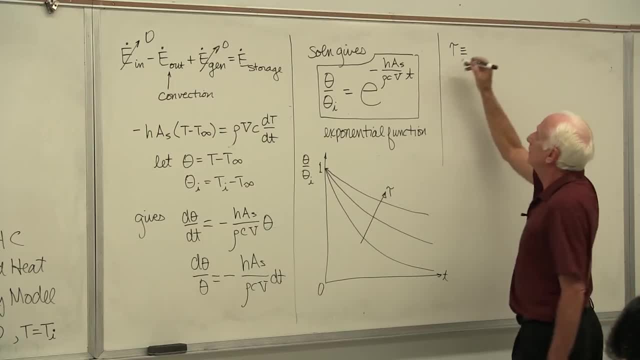 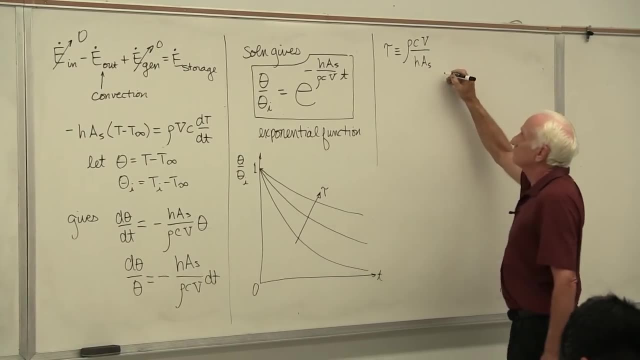 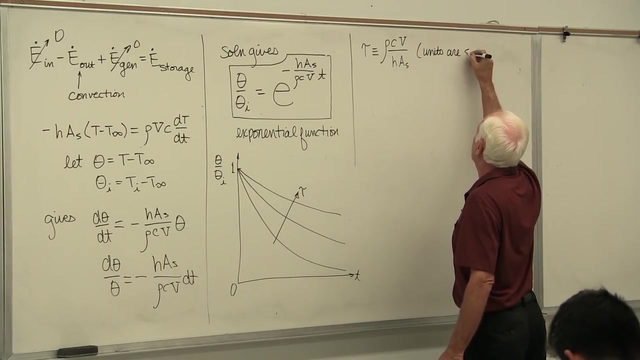 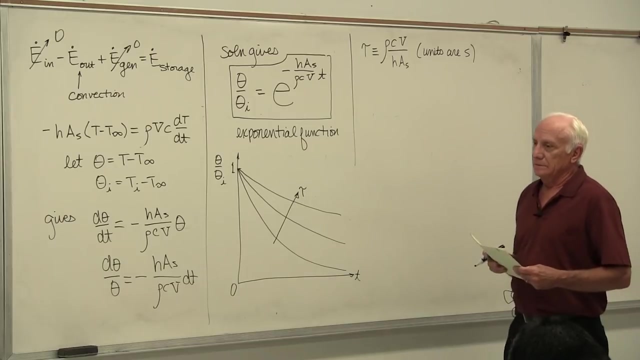 Time constant. tau is here. Rho cv, divided by has. The units are going to be in seconds or hours, Minutes, seconds or hours. I'll put down here seconds in si. They're pretty much always in seconds. That's why it's called the time constant. 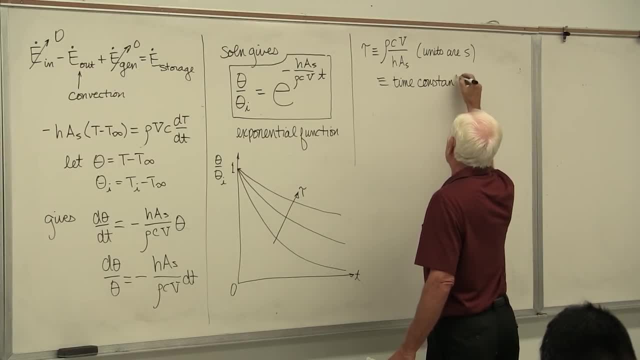 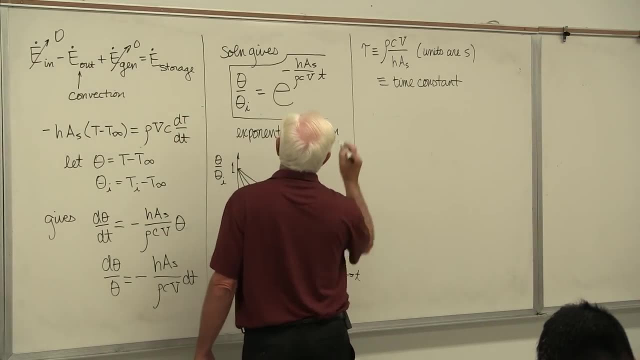 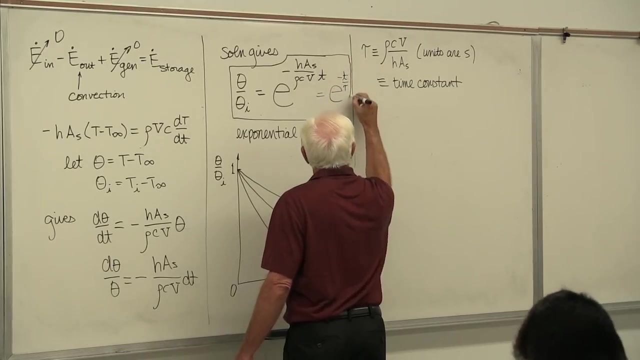 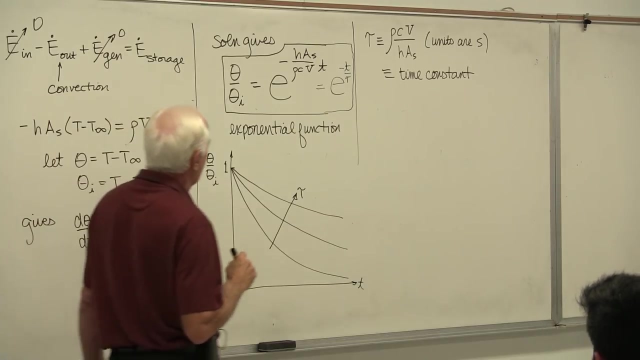 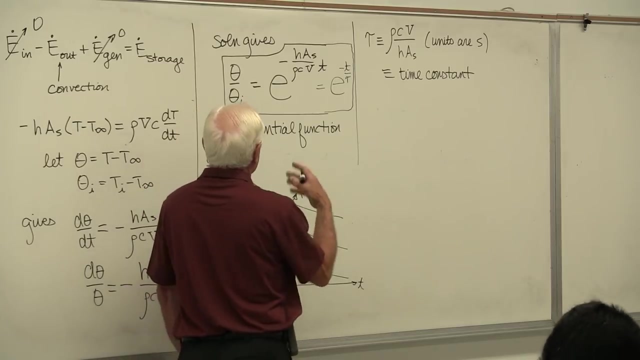 So, if you would rather, you could also express this in totally dimensionless form. That's the dimensionless equation. now, Time divided by time. What does this graph tell us? The y-axis is just temperature. So it tells us if the object, let's just say, starts out hot. 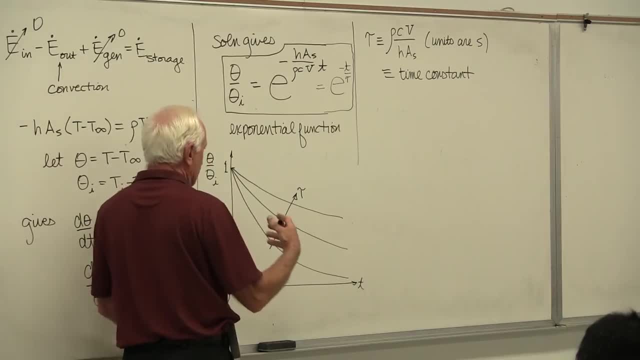 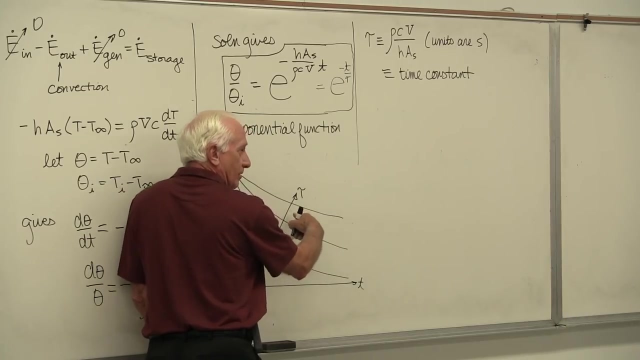 and we blow cold air over it. we know what's going to happen. The temperature's going to go down with time. But there are different curves. This is big values of time constant. This is small values of time constant. When an engineer puts that arrow on the parameter values. 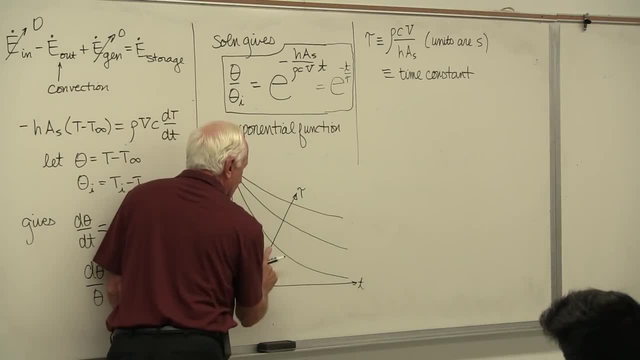 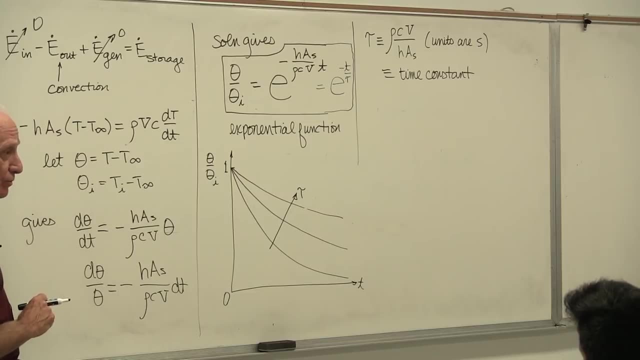 the engineer means tau is increasing as you go that way on the parametric value of the curves, Like the movie chart, Same thing We know relative roughness goes up as you go up on the movie chart. Okay, This is a low value of tau. 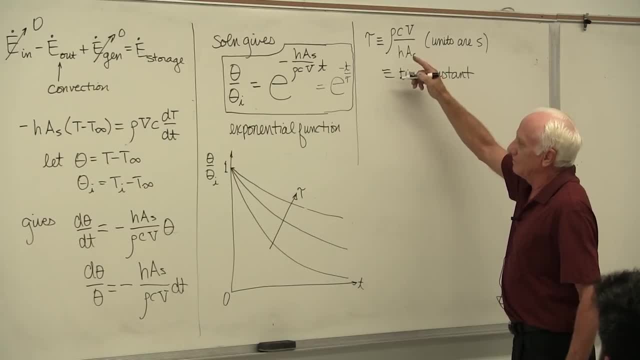 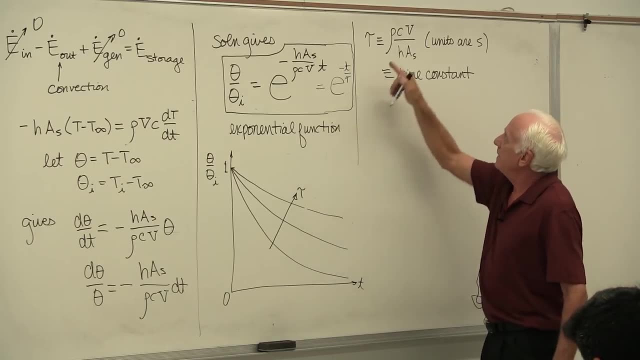 How do you get a low value of tau? Let's make a private question, Or common sense to take a high value. Take a high value of tau. How do you get a high value of that quotient? Well, one way is multiplying the density by the volume as the mass. 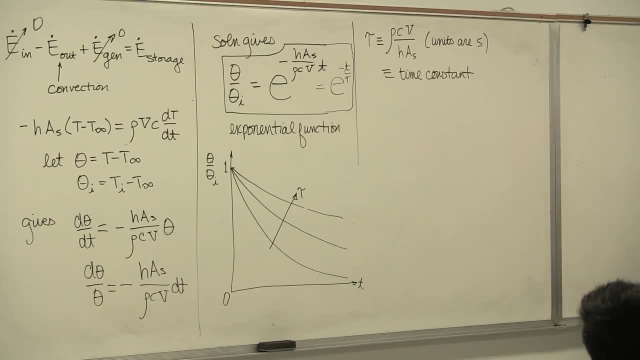 Okay, So the numerator has mass in it. If I've got a small copper sphere the size of a ping-pong ball and a big copper sphere the size of a basketball, which one do you think is going to cool faster? There's no doubt. 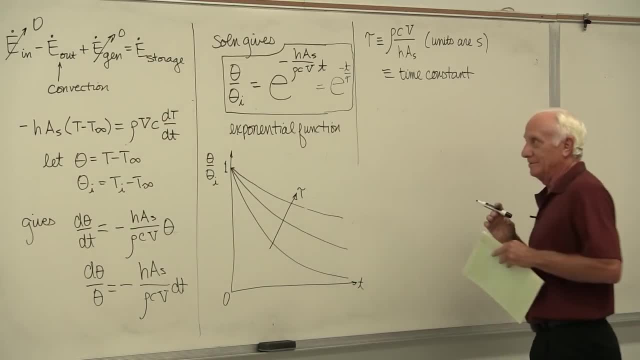 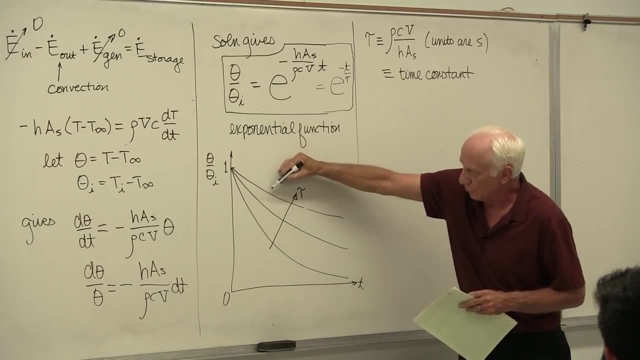 The small one. The big one cools slower, Sure, Sure. So the mass is up here. If it's more massive, tau is up here. If it's more massive, it cools at a slower rate. If the mass is small, tau is small. 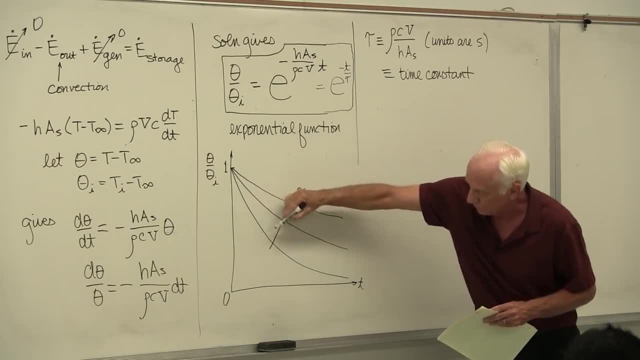 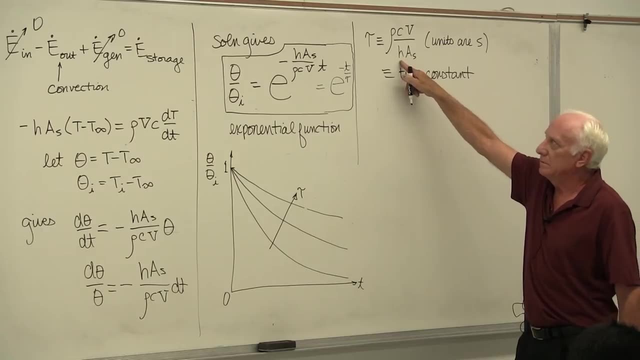 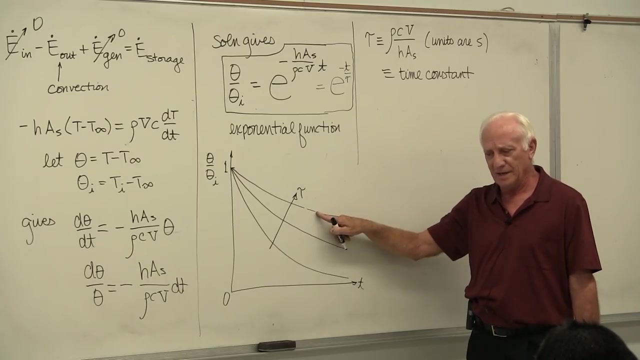 a ball bearing size copper sphere. oh yeah, it cools real fast in that air stream. How about H? If H is small? tau is big, This curve is H small. What does that mean? That means there's not much air blowing over it, and not very fast. 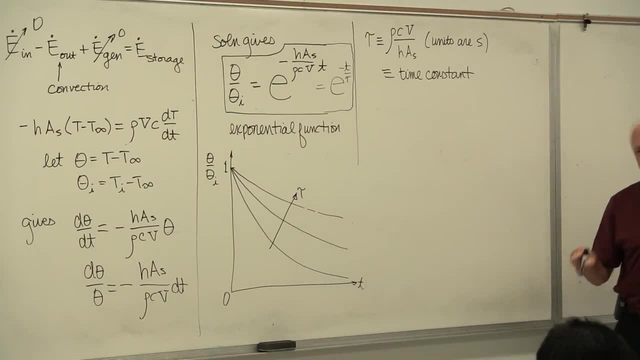 Oh yeah, It's going to cool slow. then You want it to cool faster? Put a fan on it. Oh yeah, H goes up big and now tau goes down. There's what the fan does to cool the copper sphere. So, yes, it does make common sense. 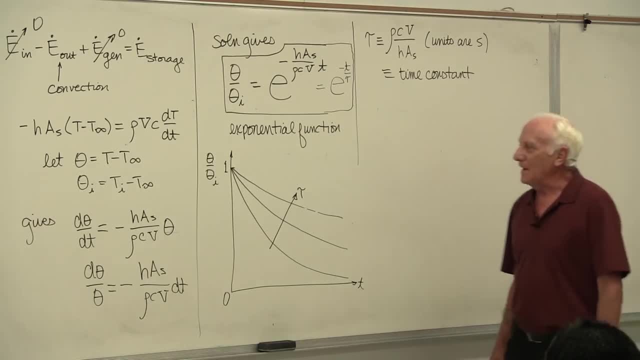 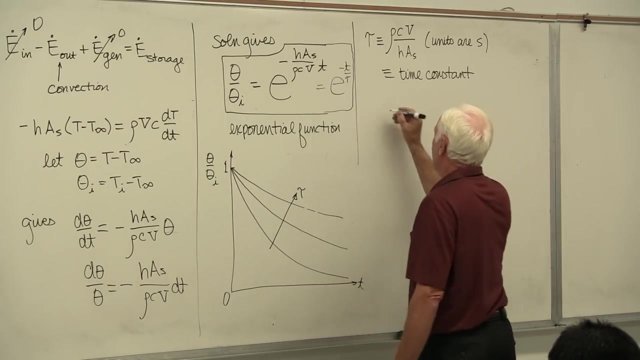 I'm saying it to you. Okay, So that's our equation. It's pretty straightforward. Now I know in some classes you've talked about time constants, but just so you know, the time constant can tell us several things. Number one: after, at a time t equal tau. 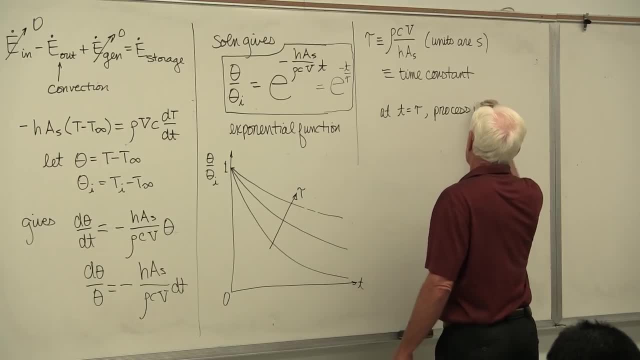 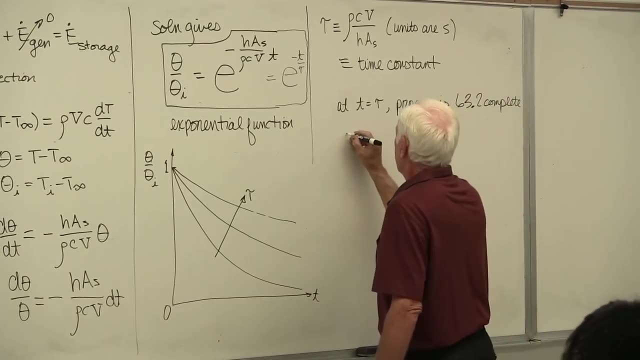 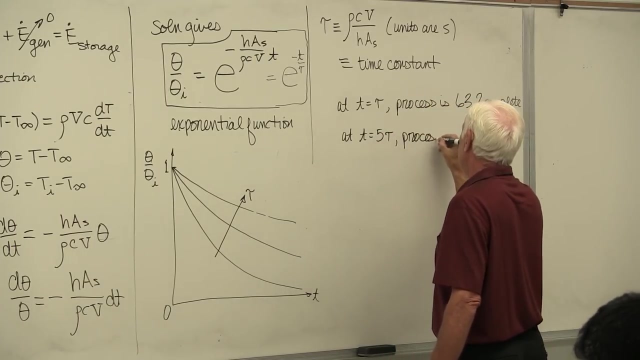 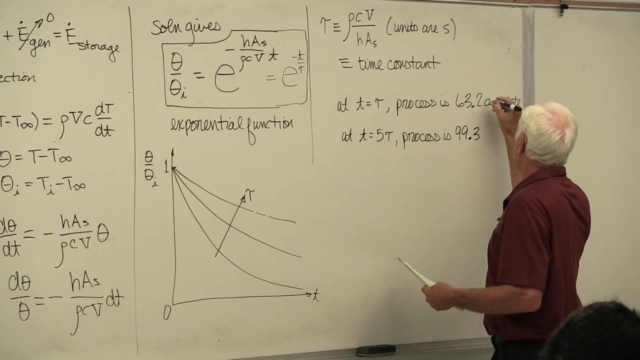 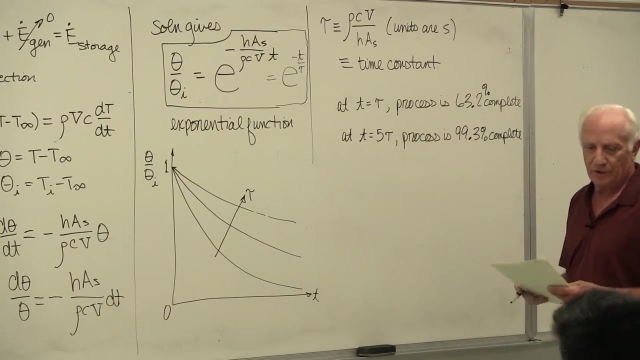 the process is 63.2% complete. At time equal five time constants, the process is 99.3% complete. One rule of thumb we engineers use. let's say you've got a thermocouple which can be modeled as a first order system like this: 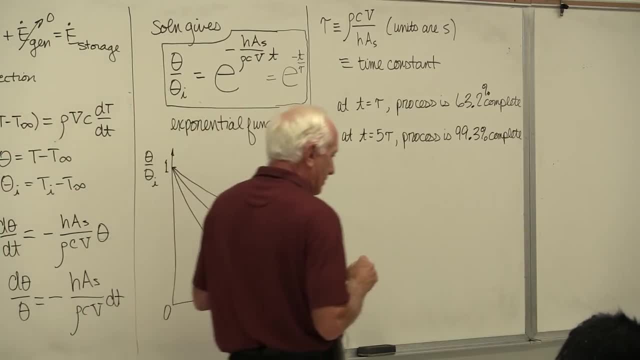 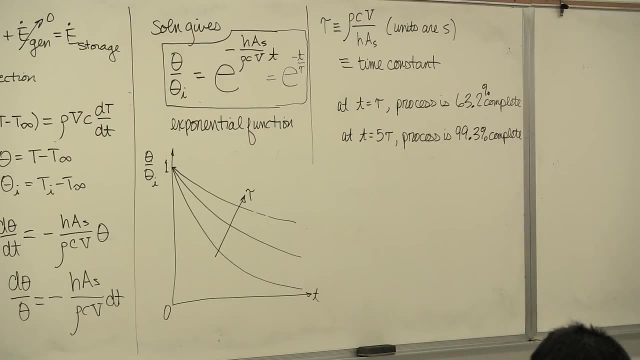 a thermocouple. If I put the thermocouple and I want to know the temperature of that wall If I put the thermocouple, if I put the thermocouple on that wall, how long should I wait before I read my digital output meter? 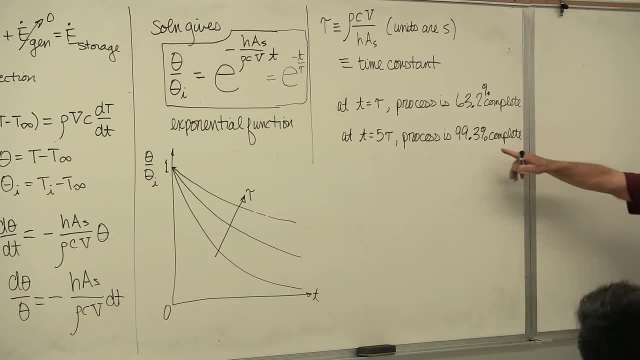 And the rule of thumb is: it's almost complete if you wait. how long? Five times a time, constant. I put a surface temperature sensor on my skin. How long should I wait to read the digital output? Well, the rule of thumb is: 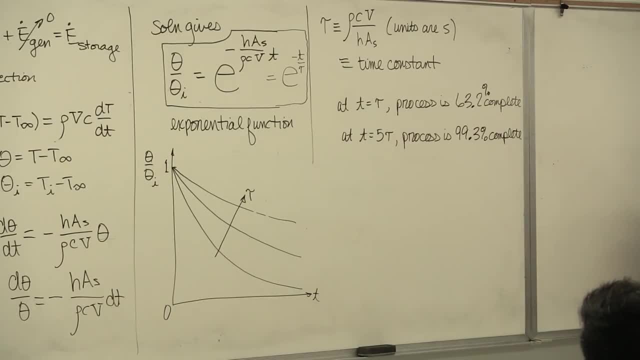 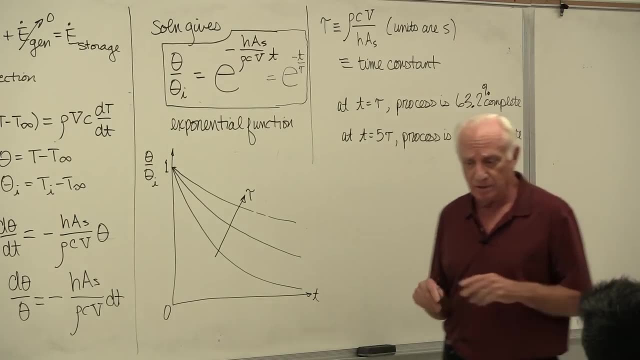 wait at least five time constants give me 99% of the way there's the true value of the temperature of my skin. So that's how we engineers use the time constant. sometimes We give this a ballpark figure: how long to wait to make or something. 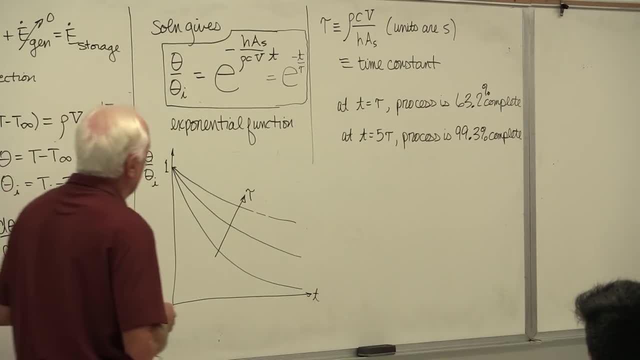 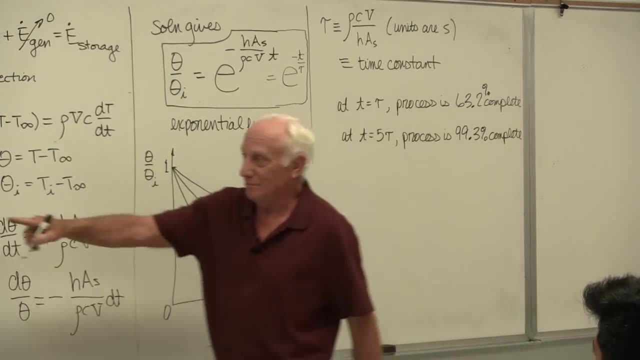 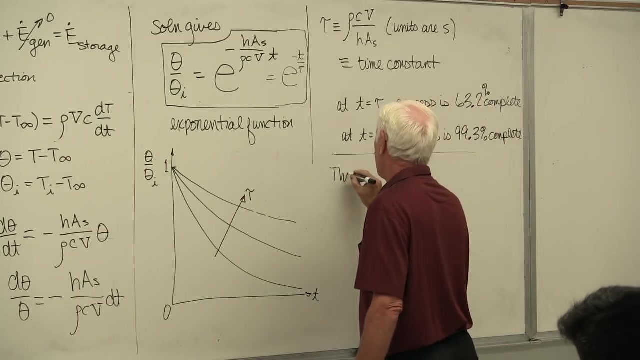 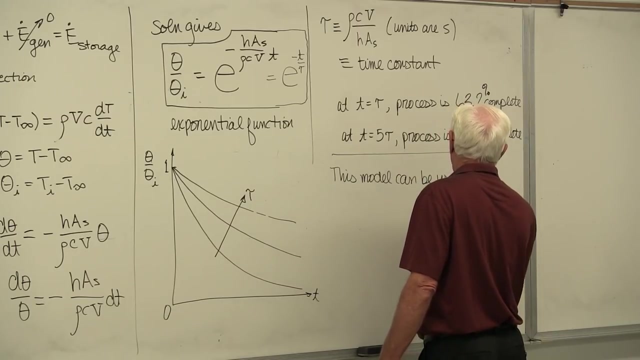 experimentally. Okay, so that's what that is. Now, of course, the question is: when can we use this simple model called the lumped heat capacity model? Okay, so this model can be used When v i the b? o number. 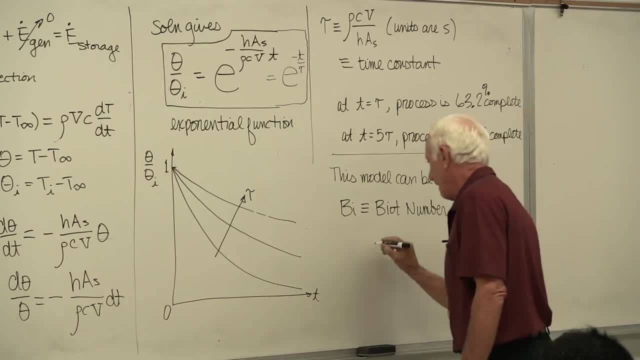 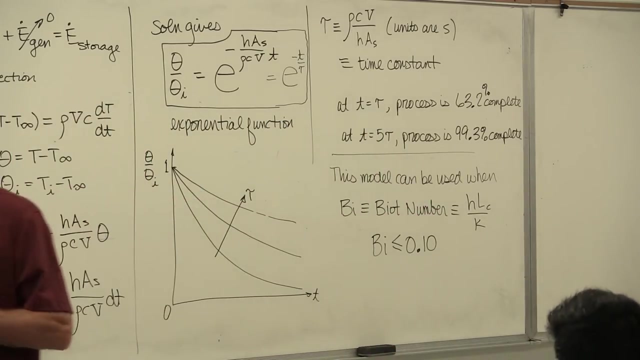 h, l, c over k one tenth. So first of all you calculate a dimensionless number. Call the b? o number. There's going to be a ton of dimensionless numbers in NE 415, wait until chapters 6, 7, and 8. 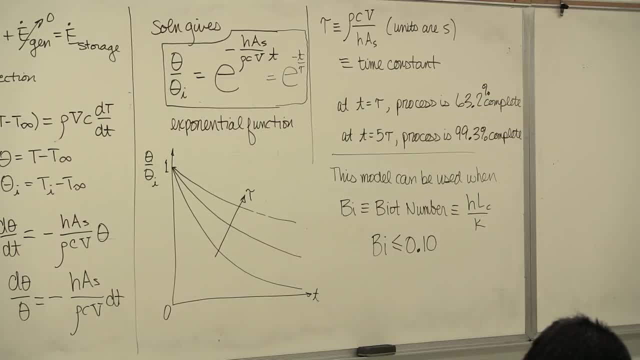 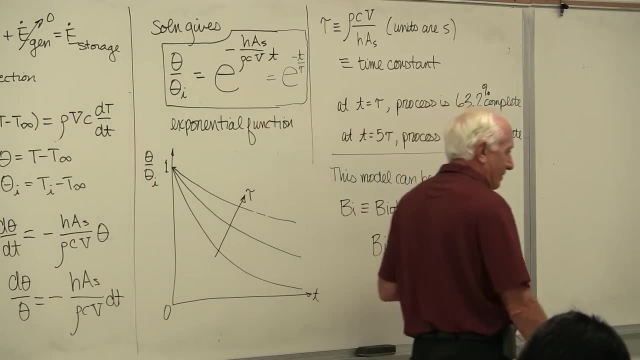 in convection, Probably 20 dimensionless numbers, at least In fluids. you had quite a few already. You know the Mach number, the Reynolds number, the Stuhl number, the Froude number, it goes on and on. 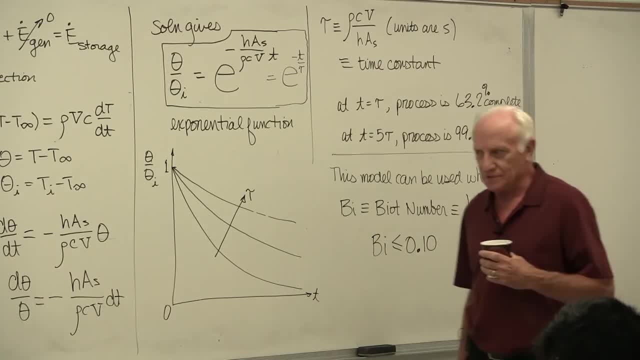 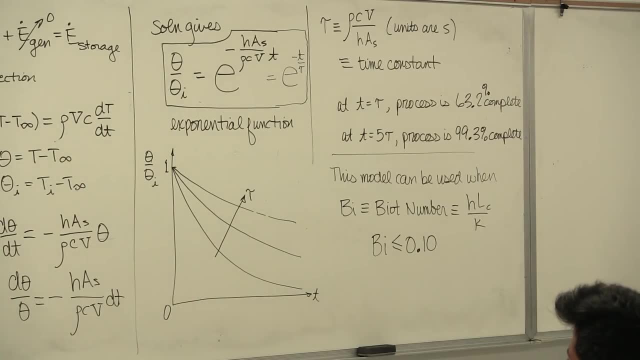 There's probably six or eight or ten. you get in fluids, In fluid mechanics, In heat transfer. there's more in heat transfer. We actually love dimensionless numbers. We're just in love with them. We try and do somewhat good with dimensionless numbers. 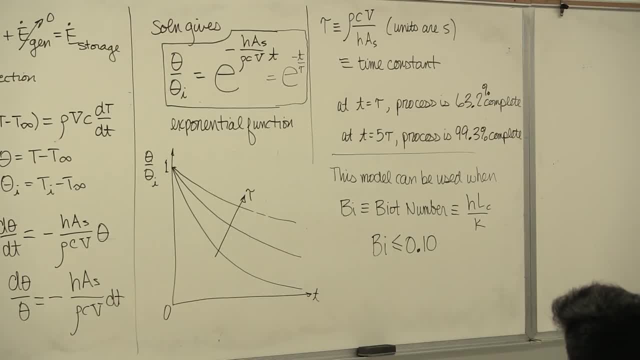 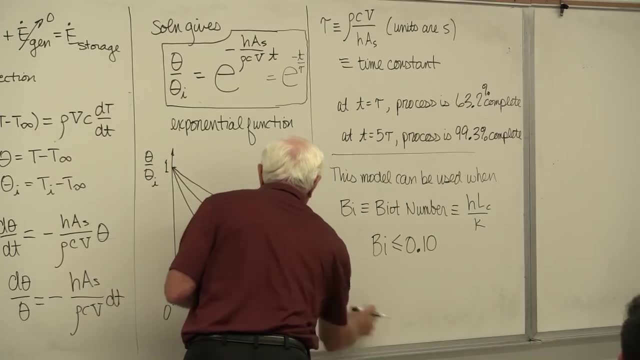 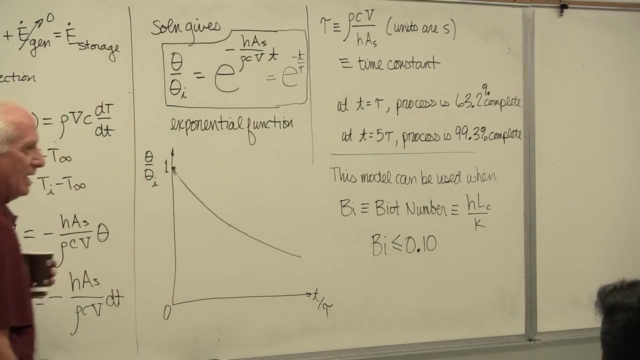 because they're so useful to us. Do you want to plot this guy versus t over tau? There it is. How many lines are there? One level Does it cover pretty much everything? All values of h, a, s, b, c row. 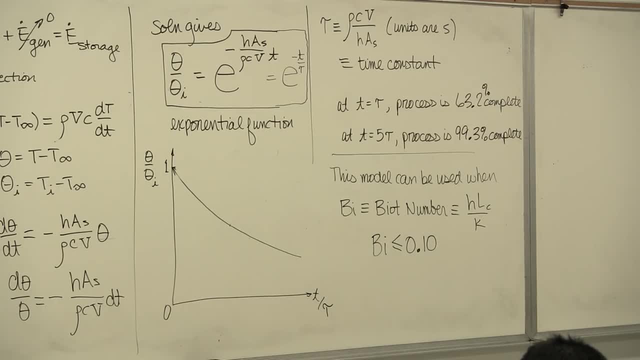 Yes, it does. That's why we love it. It correlates data. Is there a Moody graph for water: No. A Moody graph for a one-inch pipe: No. A Moody graph for a velocity of 15 feet per second: No. 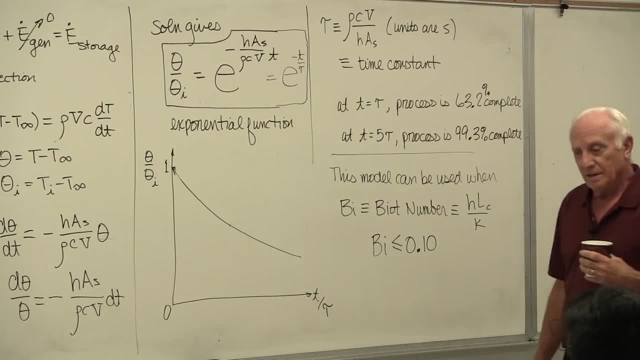 One graph covers everything. And why is that? Because we've plotted on dimensionless parameters: The friction vector f versus the Reynolds number r And the parametric value is epsilon over d, the relative roughness. That's a classic dimensionless graph like this. 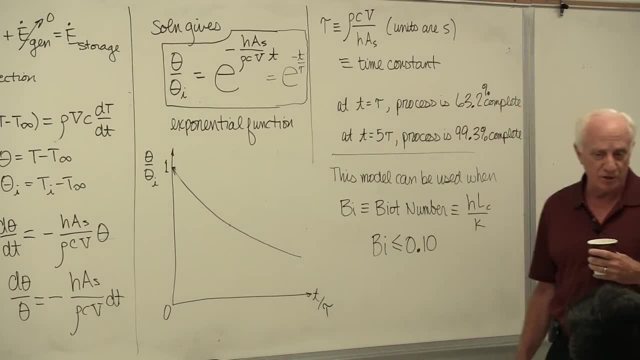 That's why we love it. I don't have five thousand pages of Moody graphs. One page, one sheet of paper covers every fluid, every pipe diameter, every velocity. Wow, Is that valuable? Yes, Thank you, Moody. Thank you very much. 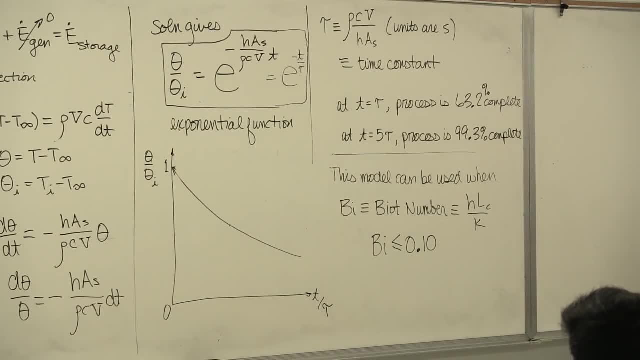 Same thing. We love these dimensionless numbers. Okay, Back to here. So that's the rule. now Let's see how we get this thing called L sub c. Now we have to shift gears. We're no longer in chapter three for fins. 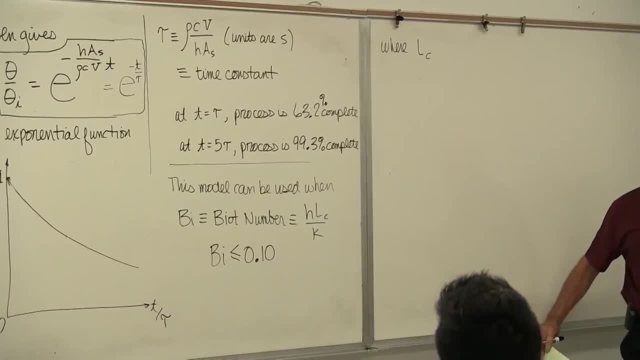 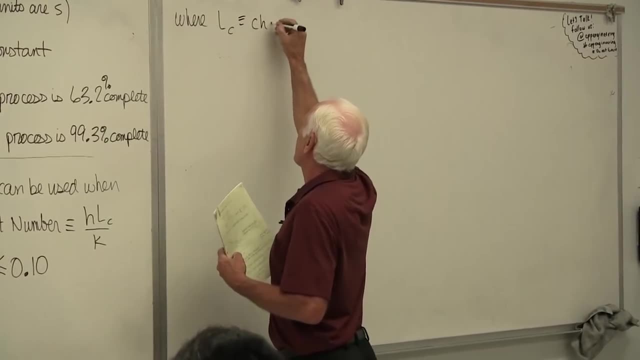 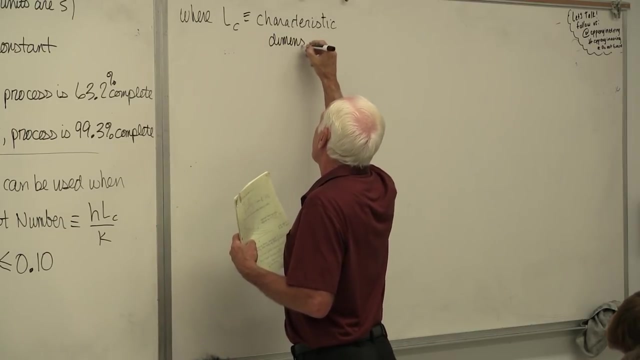 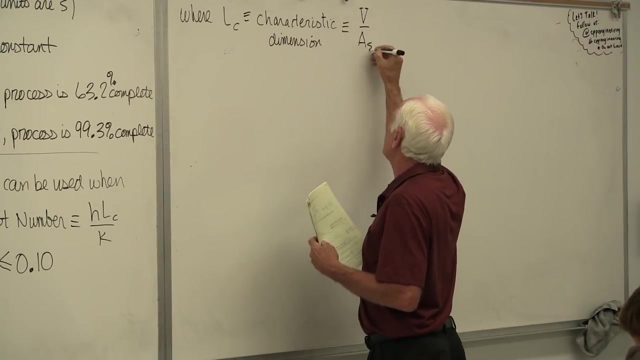 In chapter three for fins. L sub c stood for the corrected fin length. No, not this chapter five. Now, L sub c stands for a characteristic dimension. The characteristic dimension is the volume divided by the surface area. There's a table in the book. 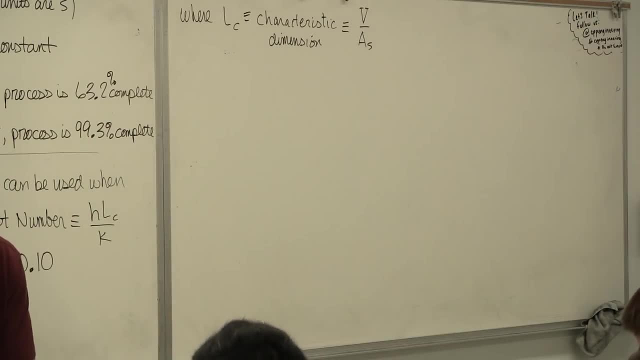 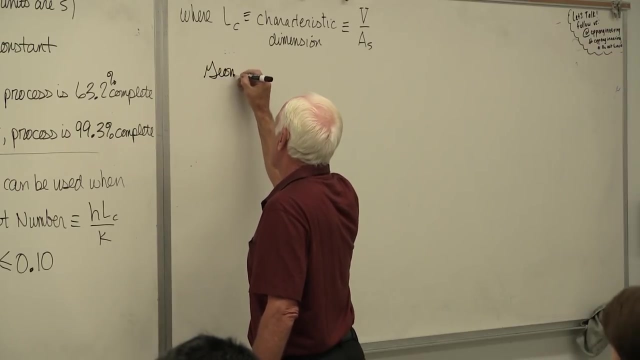 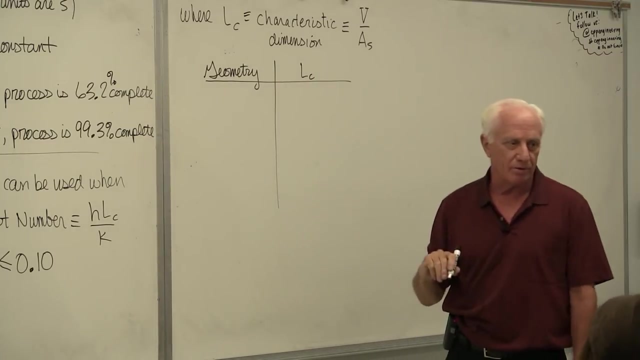 I'll just summarize it here- which gives different values for that. So if we have, let's put down the geometry L sub c. This is a table in the book. I forget what number it is: Five one probably. 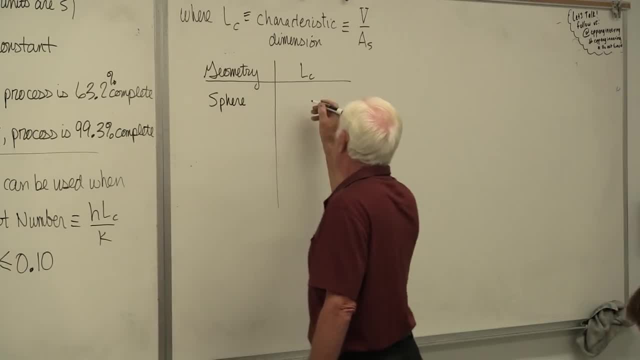 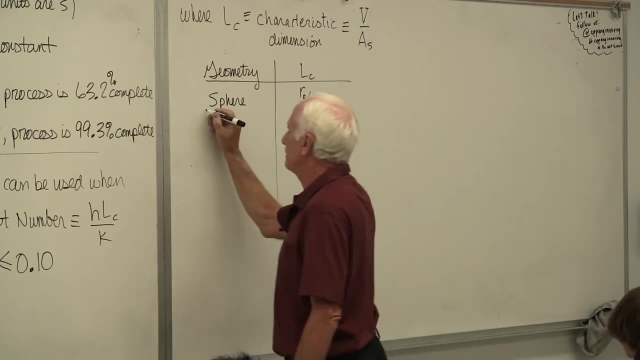 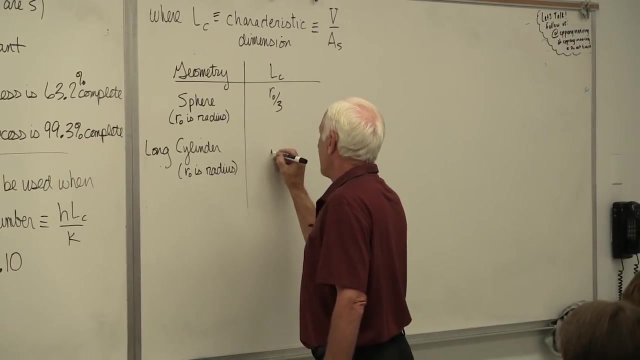 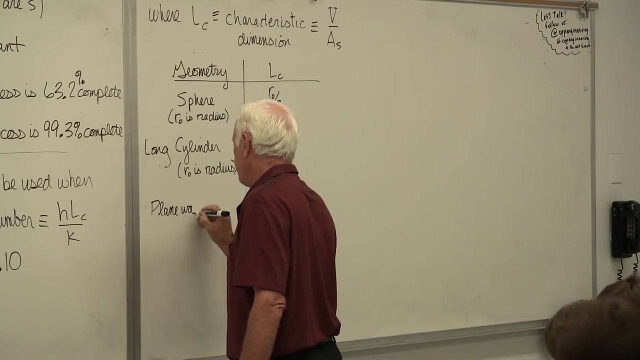 Geometry of sphere. This is d over six or r knot over three. R knot is the radius. If it's a cylinder, a long cylinder, r knot is the radius. R knot over two. If it's a plane wall, two L thick. 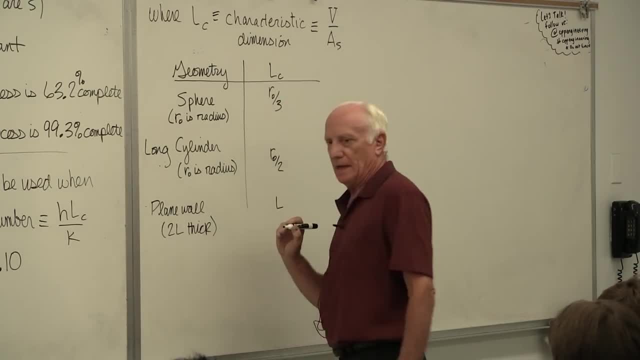 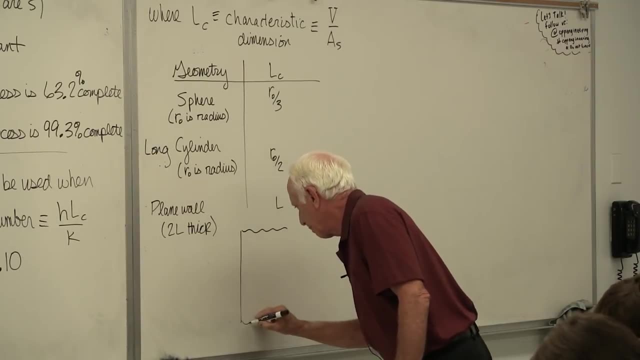 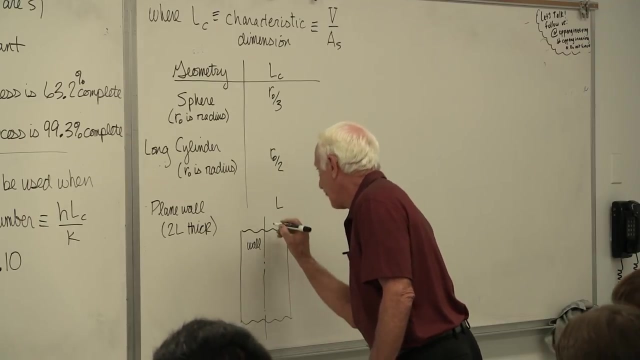 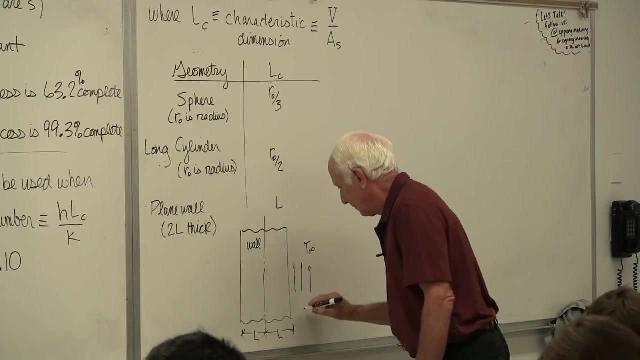 L sub c equal L, The half wall thickness. I'll draw a picture of the wall so you can look right here. So here's the thickness: L and L. There it is, The fluid blowing over here. T infinity with the convection coefficient H. 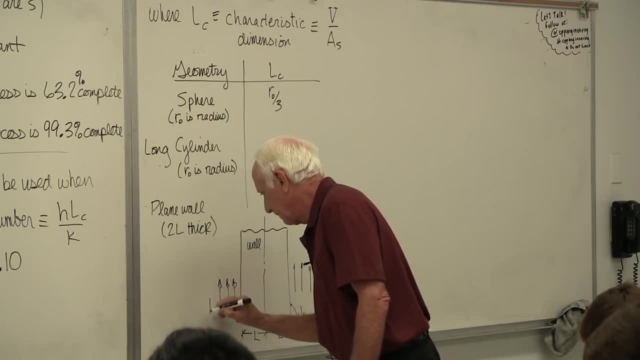 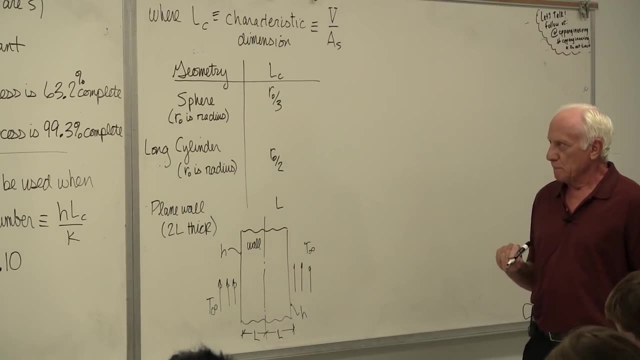 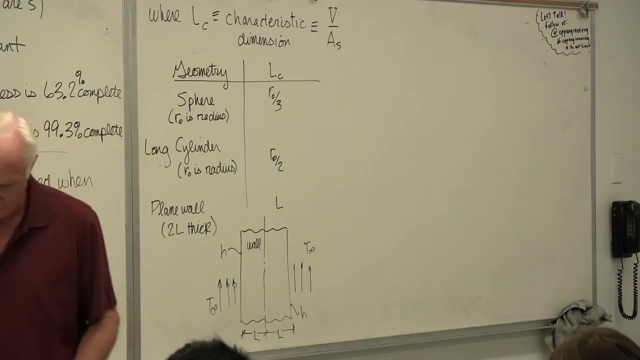 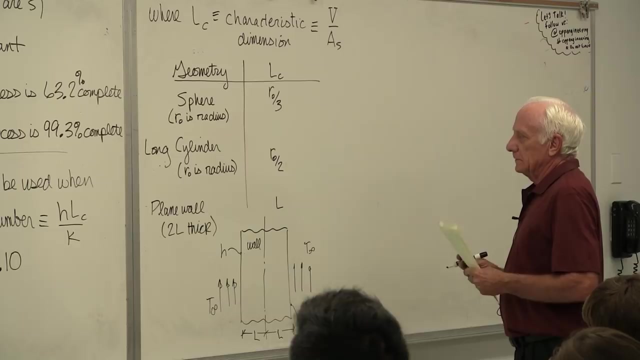 The fluid blowing over here with T infinity, with the convection coefficient H Identical on both sides of the wall, And when we do that, I'll just show you how to do this. Maybe I'll do the example problem and show you there. 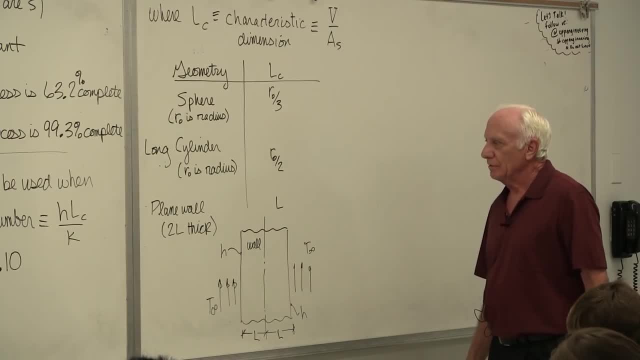 But I think I will. I'll come back to this in a minute then. Okay, So that goes up here in the BO number to check for that. Now you say: well, what if the BO number is greater than 0.1?? 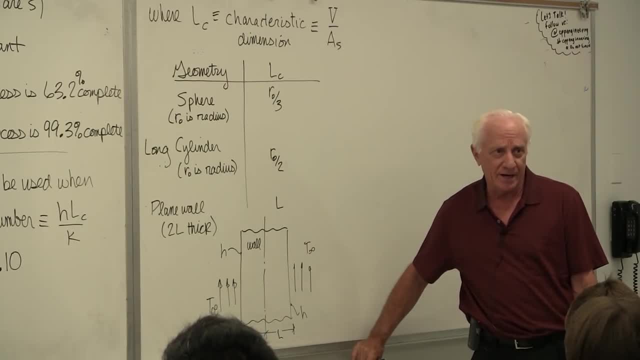 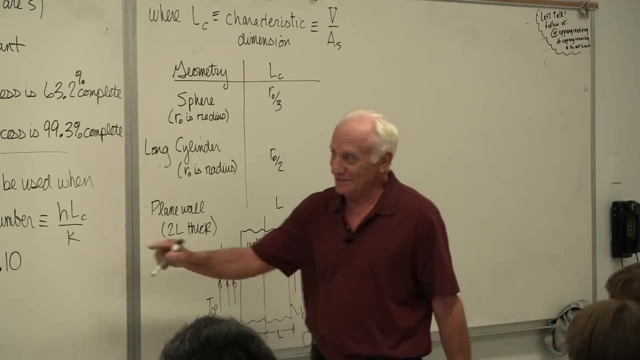 Well, I hope you can come back Friday because I'll tell you on Friday. Okay, It's the long, complicated way. This is the short, and easy way. If it's less than 110, then this method is pretty good. It gets us pretty close. 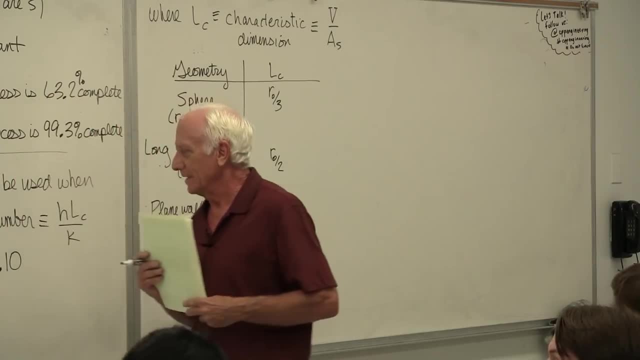 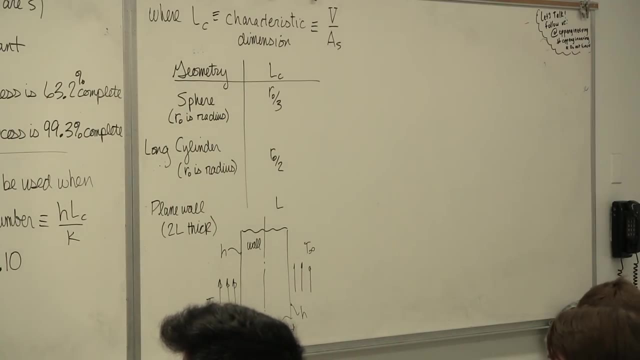 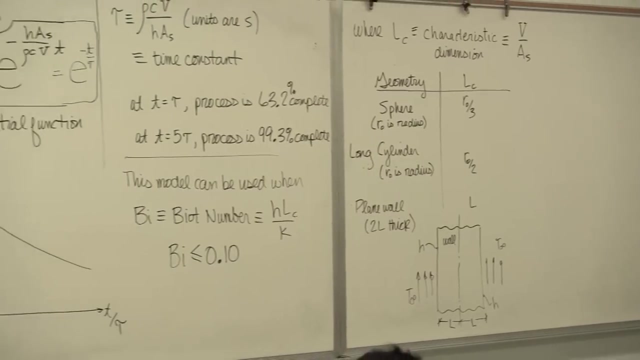 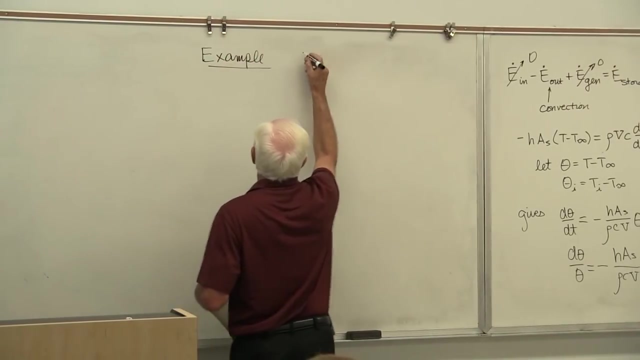 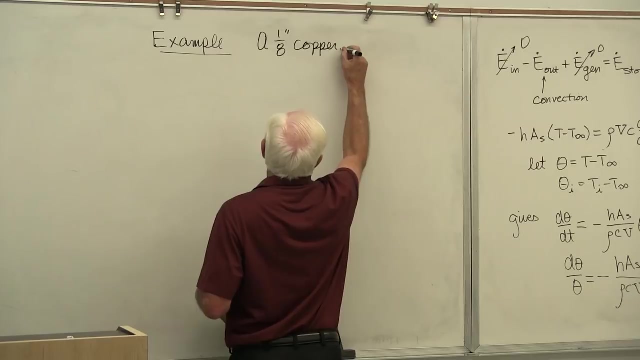 Not perfect, but close enough for most applications, All right. So we're going to use this now, this simple model for a problem of a small copper sphere. So this is an example: A 1 eighth inch copper sphere For copper. 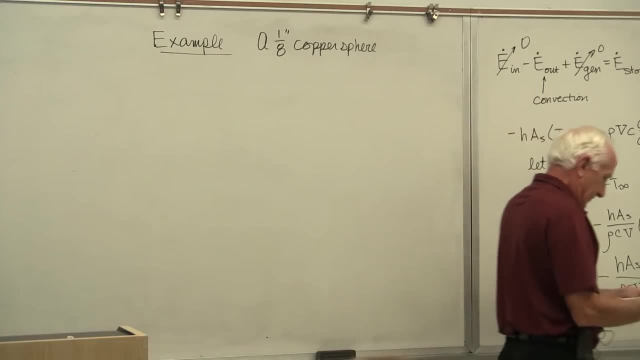 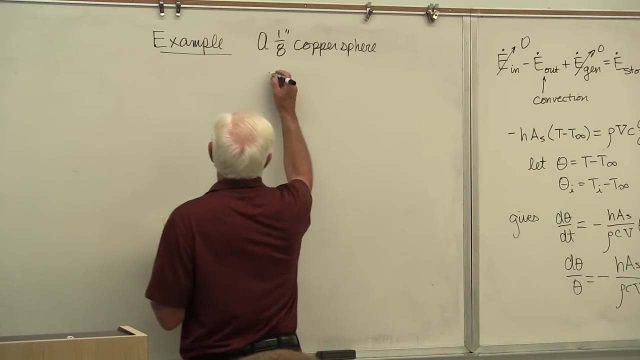 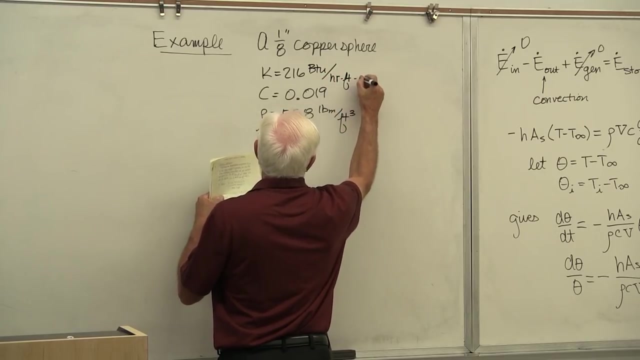 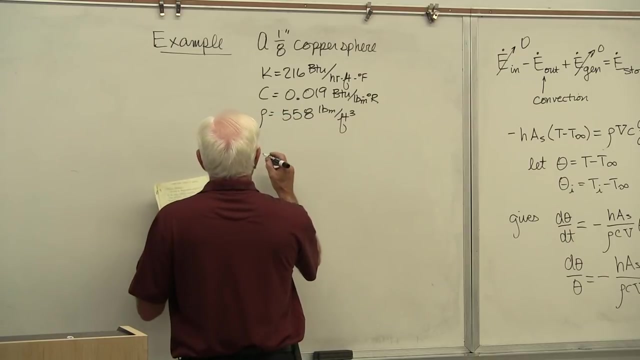 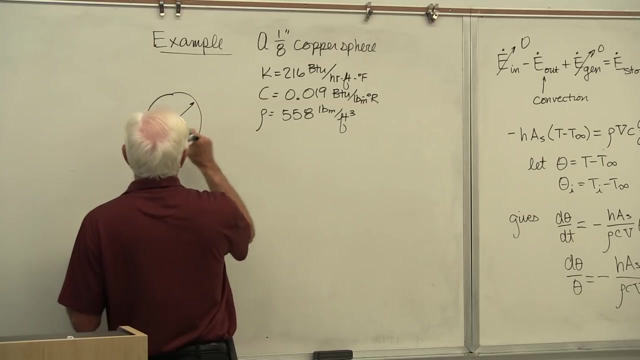 we have a density is 216.. C looks like a king Rho density: Specific heat. Let's see. Okay, Here's the sphere. This is the diameter. Okay, We have a fluid blowing over the sphere T- infinity. 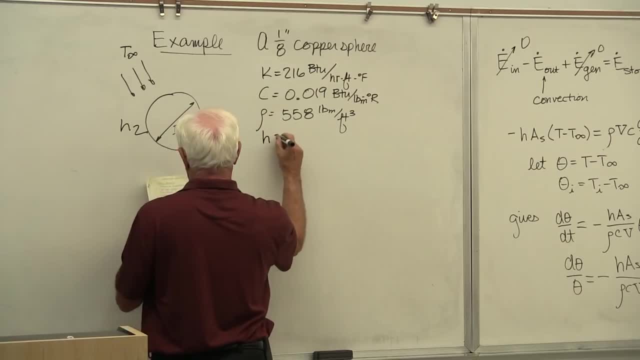 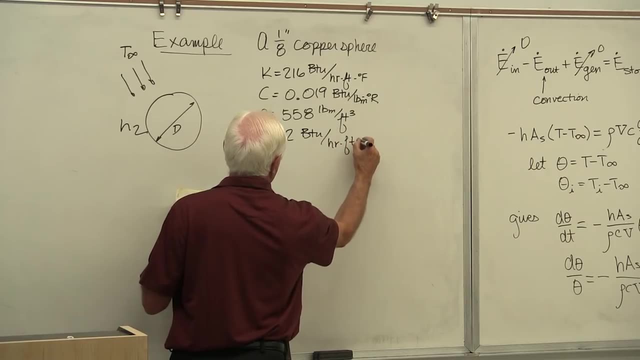 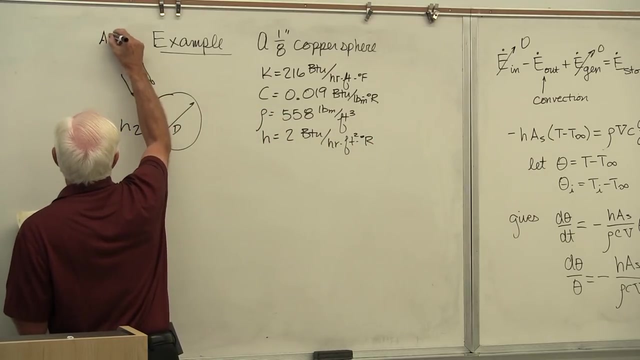 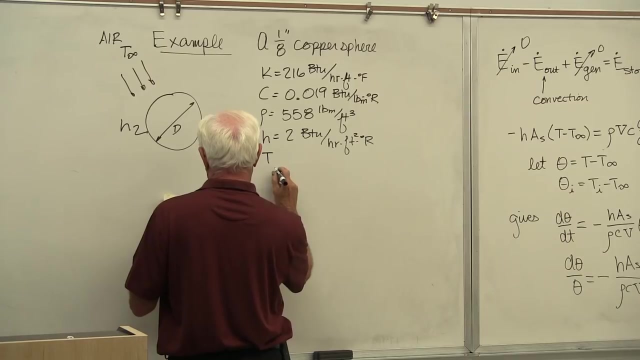 with H on the outside of the sphere, H is 2.. This is air flowing over the outside. T infinity is a zero is a T infinity is 100 degrees C. Initial temperature of the copper sphere is 300 degrees And we're asked to plot. 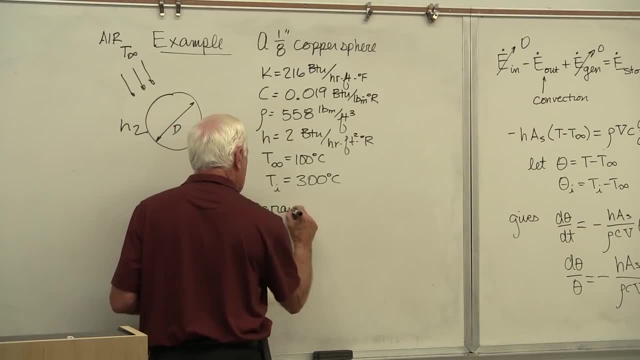 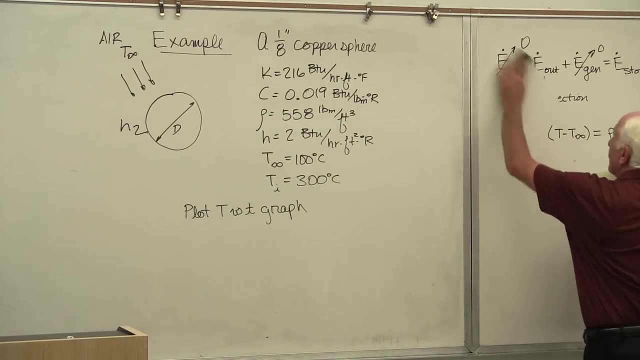 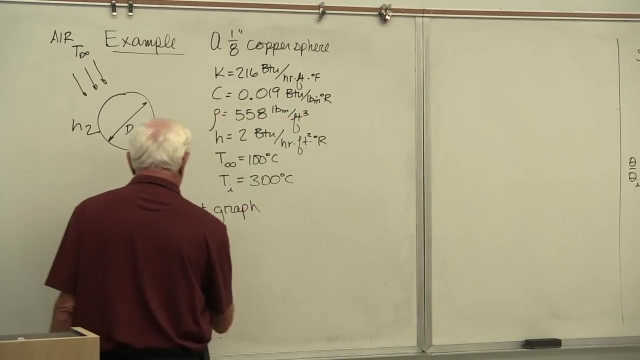 T versus time graph: Okay. T versus time graph: Okay. Obviously, first thing to do, we better see if we can use an easy way out, The field number. So field number I need LC. LC equals the volume of a sphere. 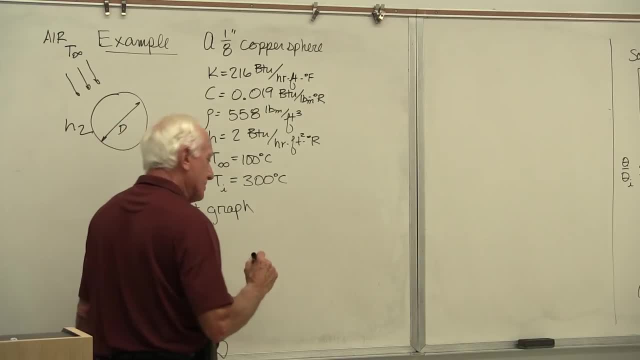 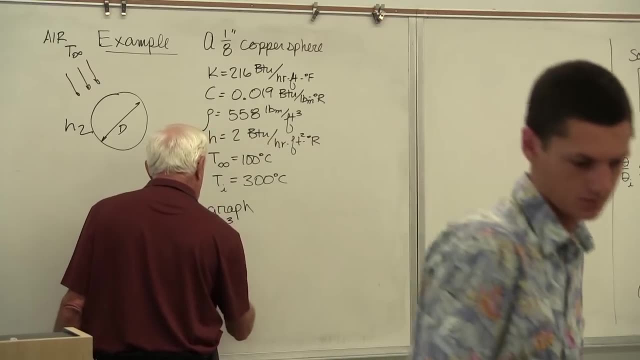 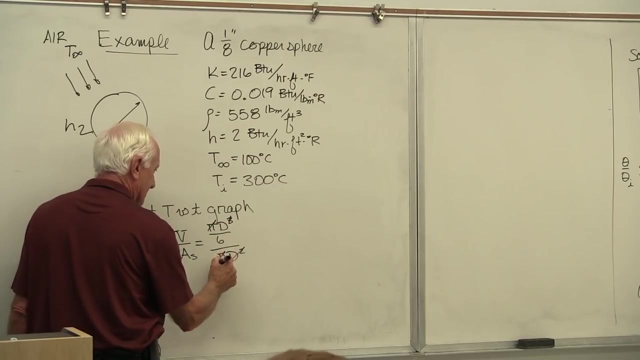 divided by its surface area. The volume pi D cube divided by 6.. The surface area, pi D squared I. I know you, you canceled stuff, but like didn't you just put the geometry up there for LC? I'm sorry. 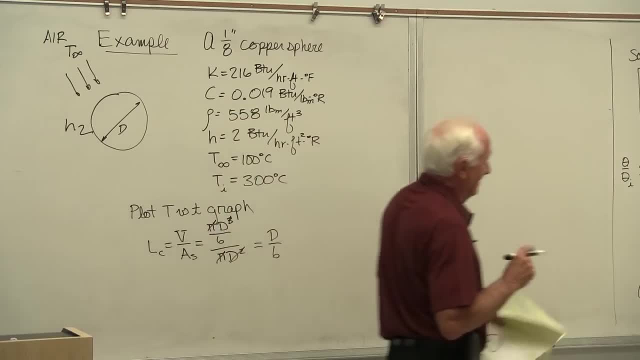 Sure, Sure, Okay, All right, You don't want to do that, Because the answer I get now better be that guy. You don't have to do it. If it's a sphere, you pick it off right here. L, sub C. 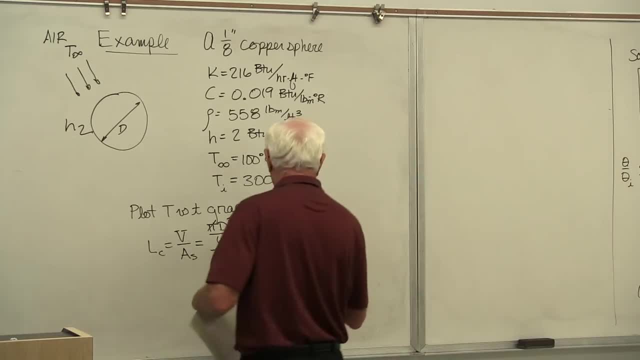 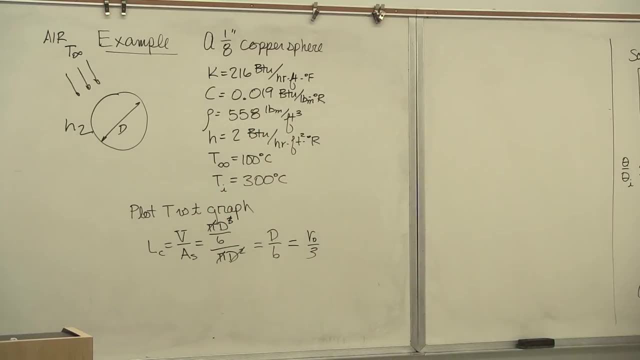 is R naught over 3, or D over 6.. D is 2 times R naught, So R naught over 3.. We've just proved that right there. There it is. There it is. You want to prove the other ones? 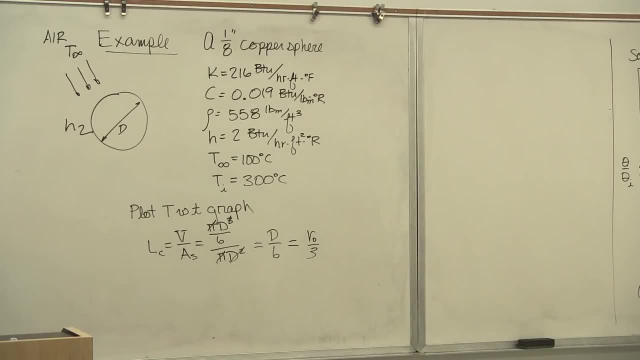 Okay, Let's do the long cylinder, Long cylinder D. Okay. L sub C equals volume over surface area, Volume: Pi D squared L. Pi D squared over 4.. L Divided by the surface area: Pi D. 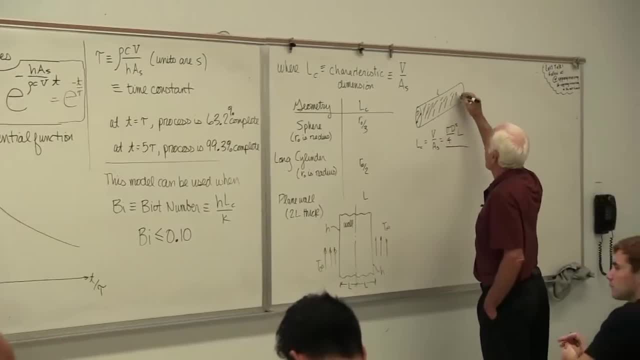 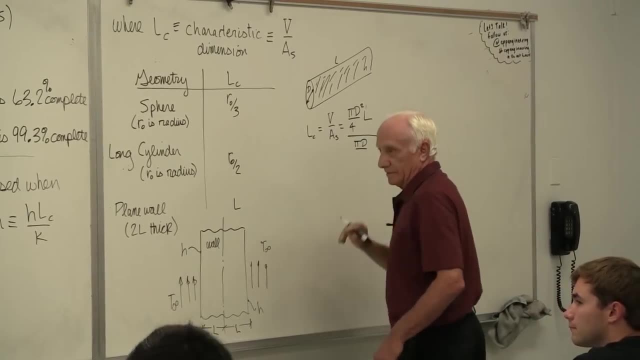 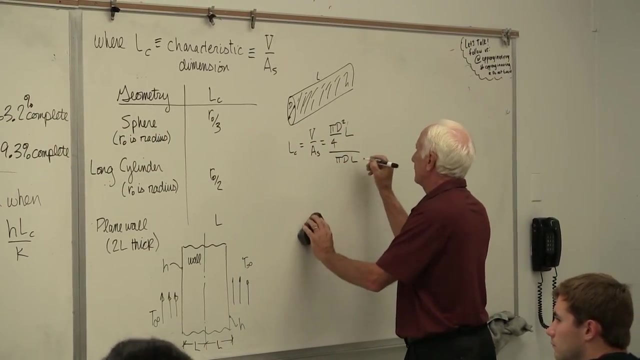 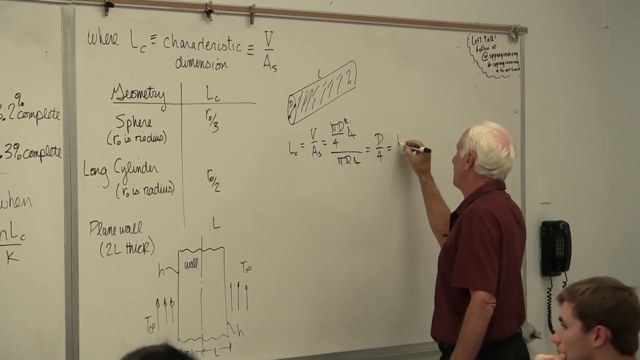 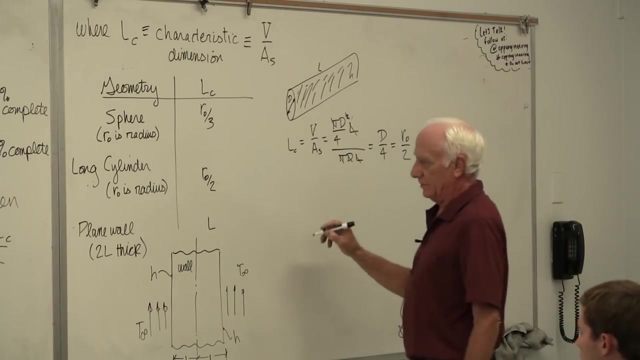 Here's the surface area: Pi D times L, Pi D. Cancel, cancel, cancel, cancel, Cancel, cancel. D over 4, which is R naught over 2.. Yeah, There it is Plane wall. You want to do that one? 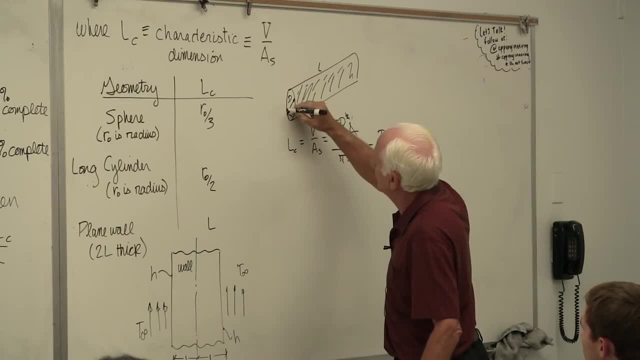 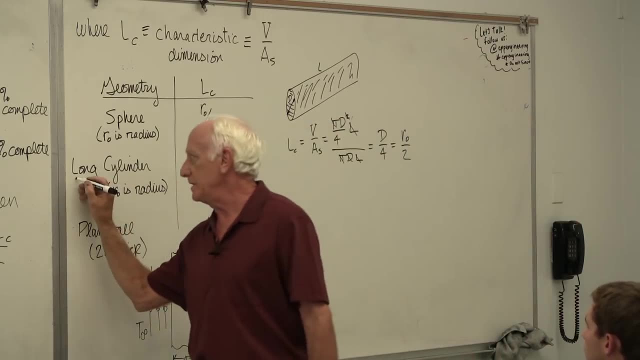 I don't know if you can do the plane wall. You say: well, wait a minute. You didn't include this area for convection, for surface area. No, I didn't, Because there's a magic word here. The magic word is: long, There are no ends. 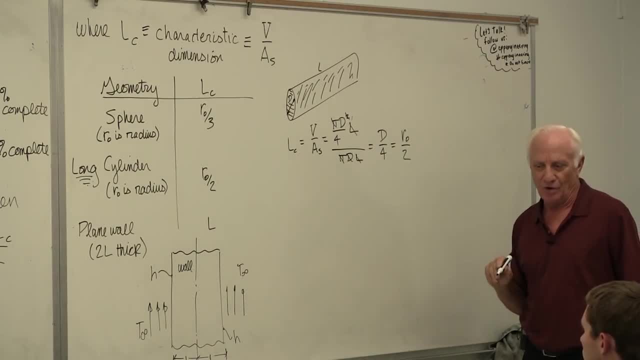 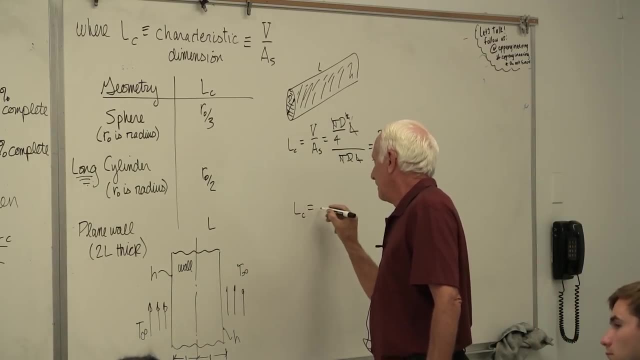 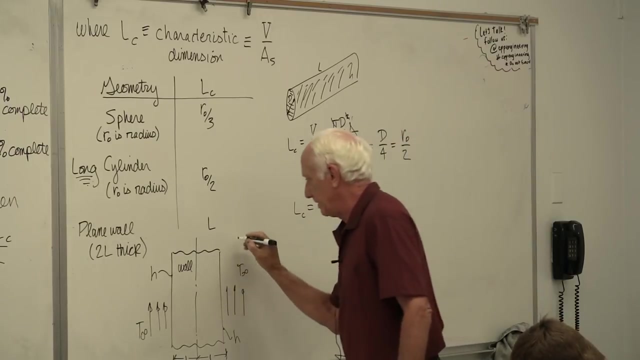 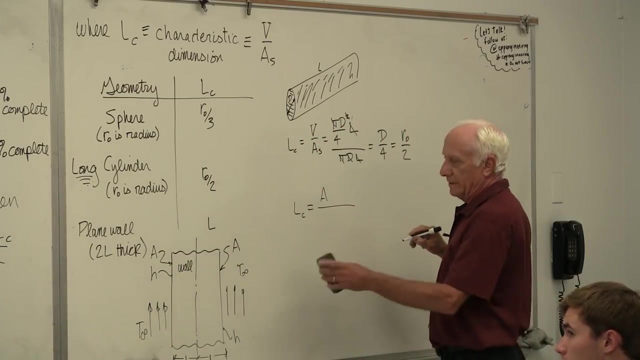 Long means ignore the ends. Ignore the ends, It's long. Plain wall Volume. Surface area times 2L. The area on the outside. Here's the area of A. Here's the area of A. 2 times A. Okay, so the volume is A times 2L. 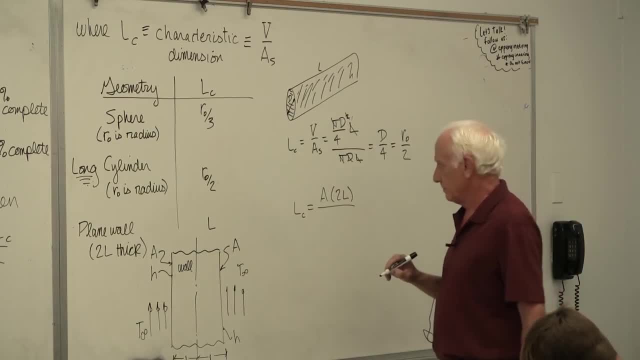 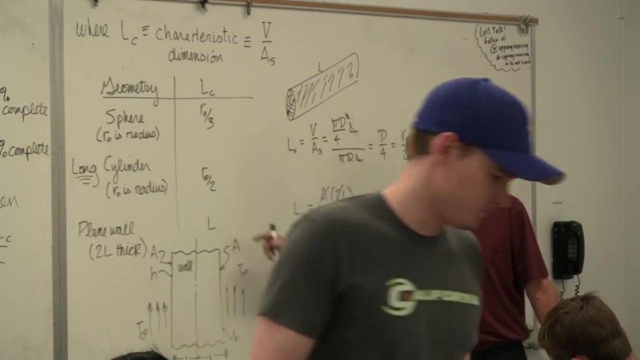 The surface area: Left hand side, right hand side. Each area is A Left hand side, right hand side, 2A. Cancel, cancel, cancel, cancel. Yep, It's just L, It's just L. So that's how you get those three things. 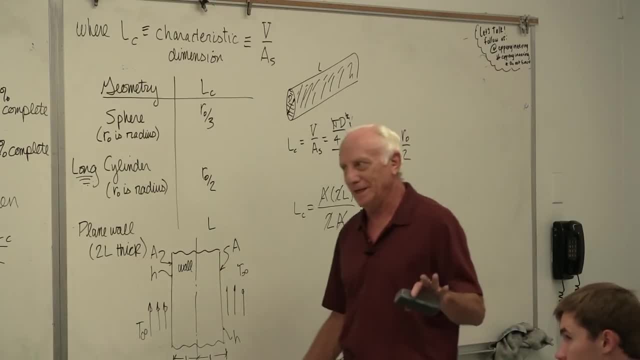 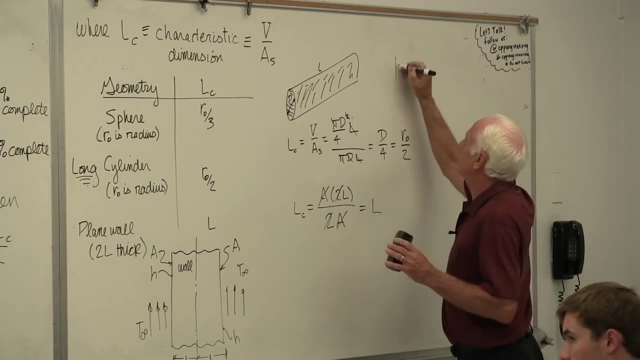 But the general rule is, if you want to find L sub C for any shape, here's what you do. Take the volume, divide it by the surface area. Just as another quick example, Let's say you've got a little cube of copper. 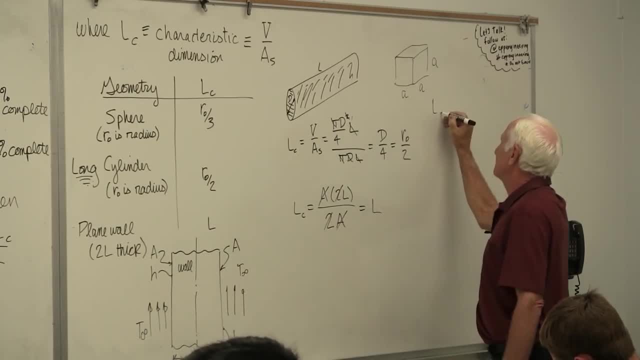 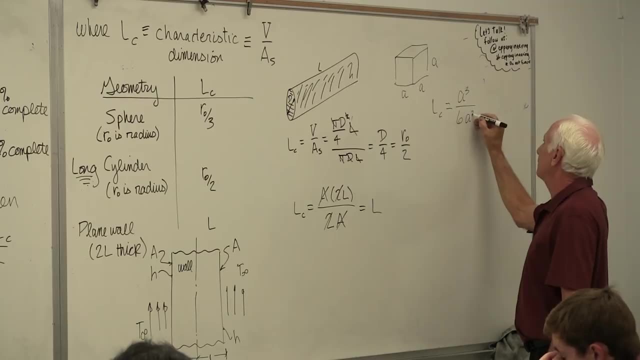 And it's A by A, by A. L sub C is the volume A cubed Divided by the surface area. 6A squared. Cancel, cancel A over 6.. No matter what it is, that's how you get L sub C. 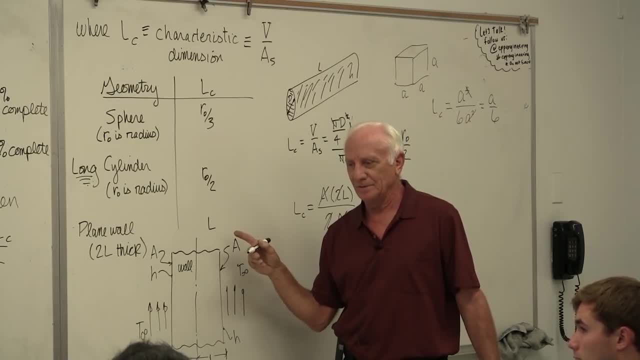 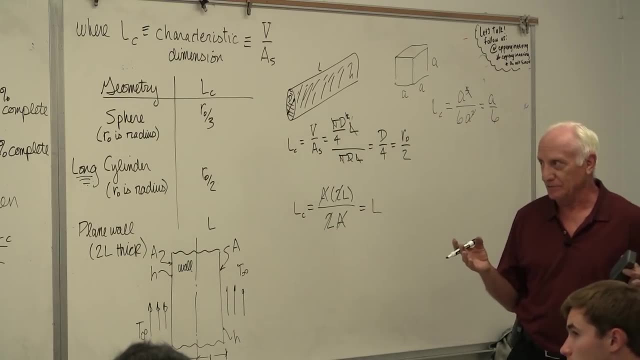 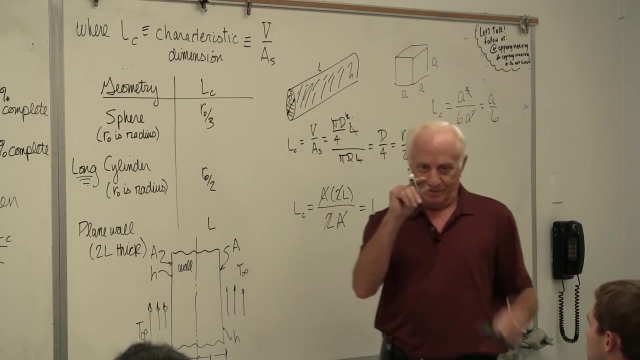 Why are these three things so important? Well, because the engineers use them a lot. If you want some examples, I'll give you three specific examples. If you're going to heat, treat ball bearings in a furnace, how long should they be in there? until the outside of the ball bearing is hardened? 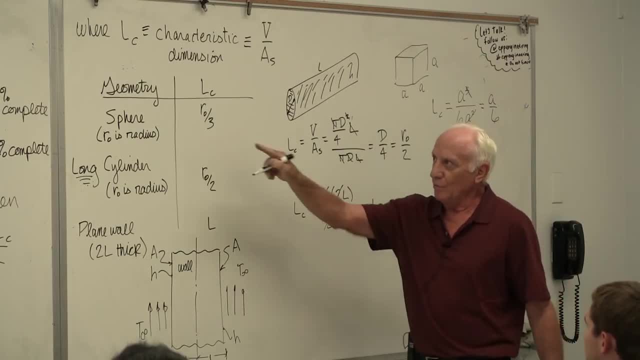 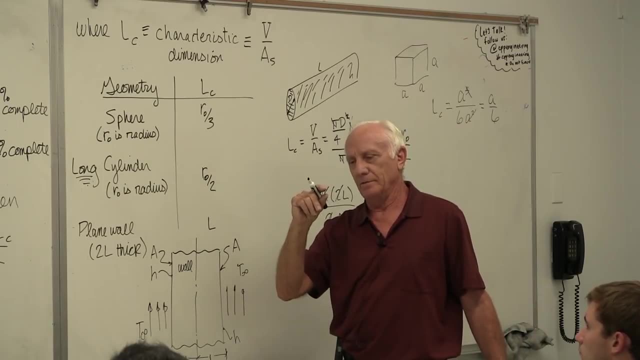 The ball bearing's hardened. How long should I keep that in there? We need, we need this guy. That's a ball bearing. If I have 3 16ths inch wire on a spool, how many feet are on that spool? 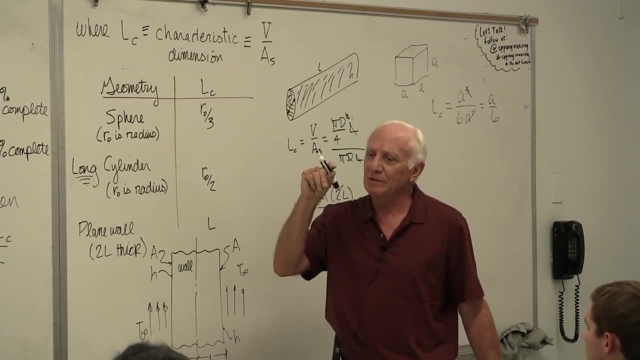 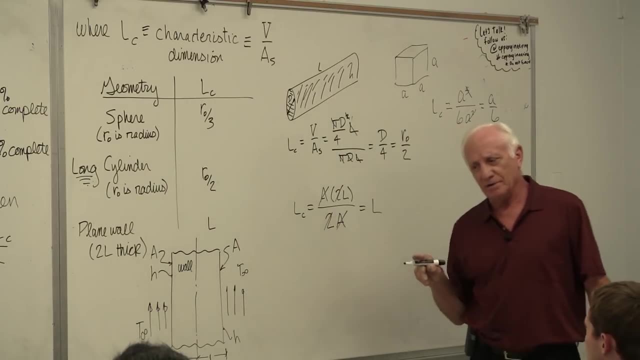 I don't know 200 feet. How big is the diameter? Oh, let's just say it'll be a quarter inch. Is that a long cylinder? Sure, a wire's a long cylinder. You put that wire through a furnace. how long should it be in there to heat? treat that. 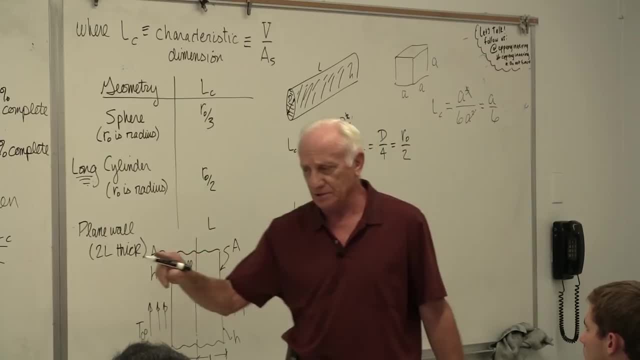 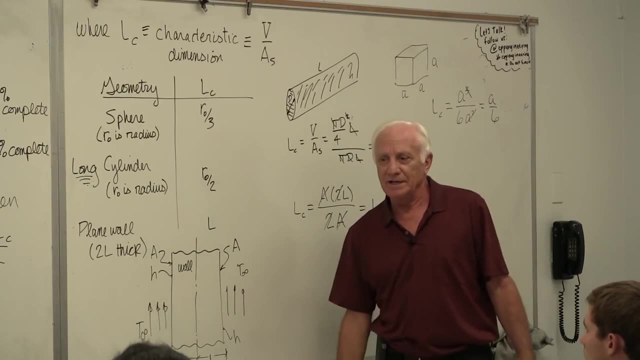 How long should it be in that furnace? How fast should that wire go through the furnace, The speed So when it comes out that end over there it's been heat treated. That's wire On a plain wall. you want to heat treat a slab of steel one inch thick in a furnace? 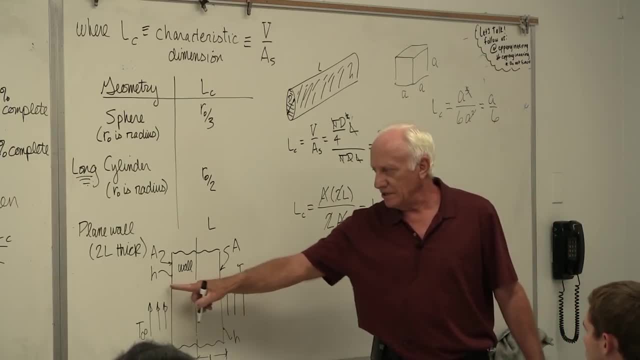 Yeah, there it is, Slab of steel. Convection on both sides Comes in hot, Gets hotter as it's heat treated. These are common things that occur in engineering, Whether they're ball bearing wire or maybe a slab of steel being heat treated. 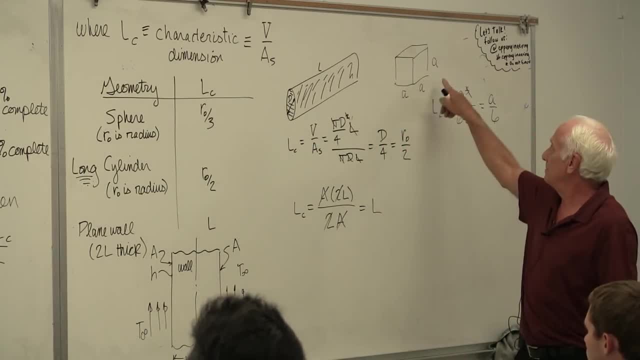 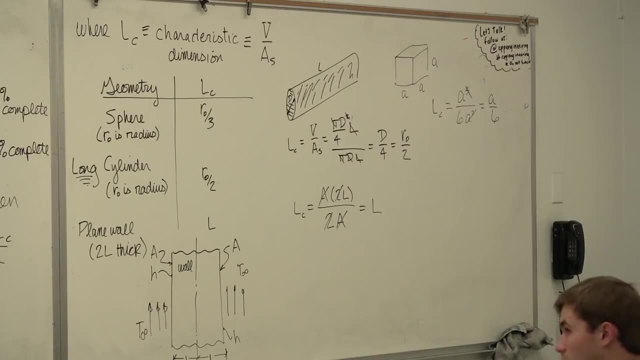 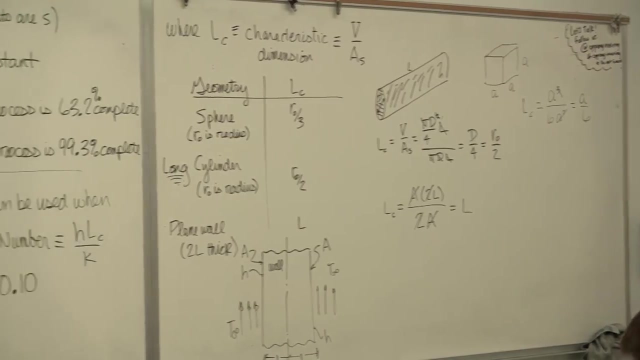 That's why they're listed in this table. But the other ones you can get them yourself. I had it over here, Okay, so back over here. We got this guy. Let's get the VO number now. VO number is equal to HLC over K. 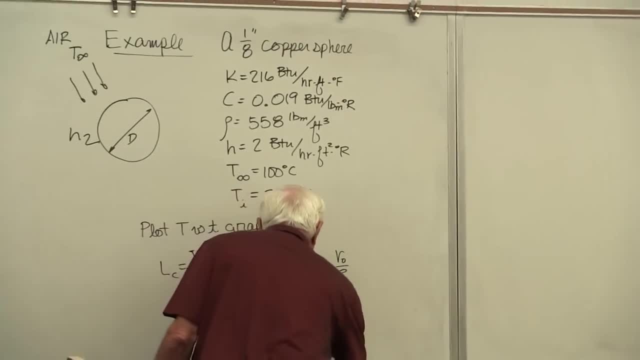 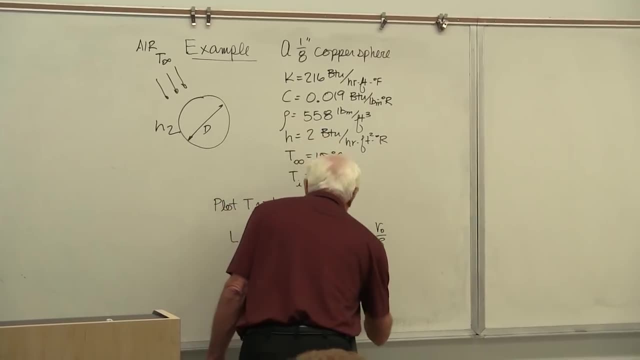 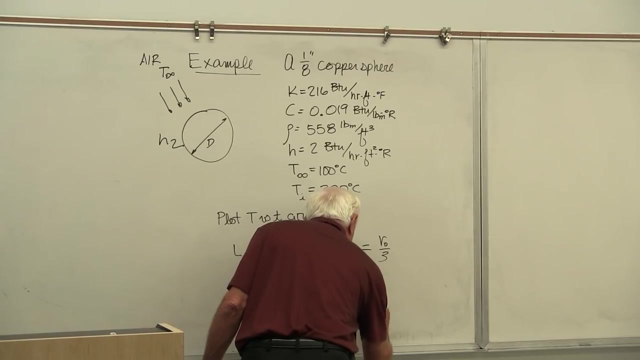 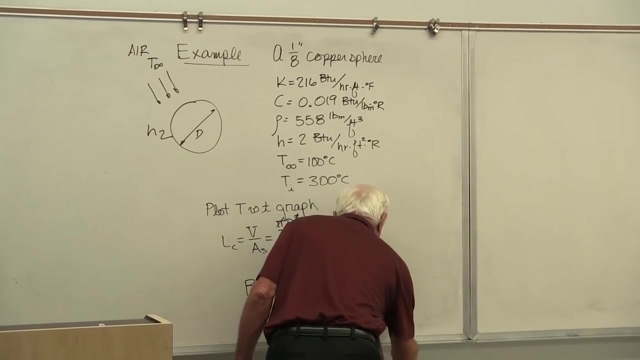 HLC over K. H is 2.. L is R0 is a diameter over 6.. The diameter is 1 eighth inch Divided by 12.. Divided by 6.. Okay, divided by K for copper 216.. 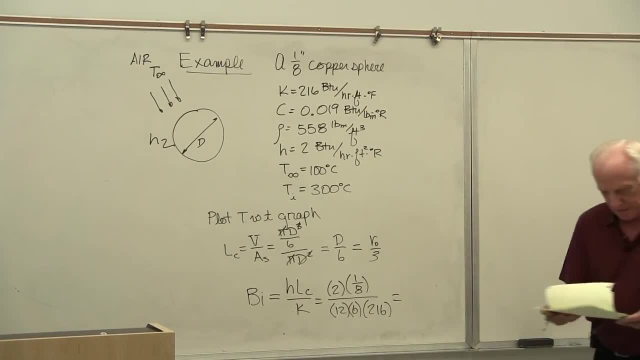 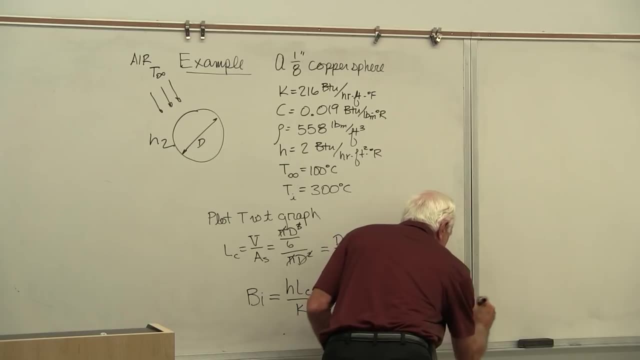 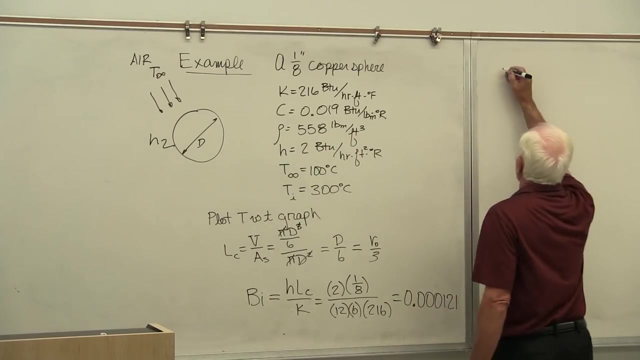 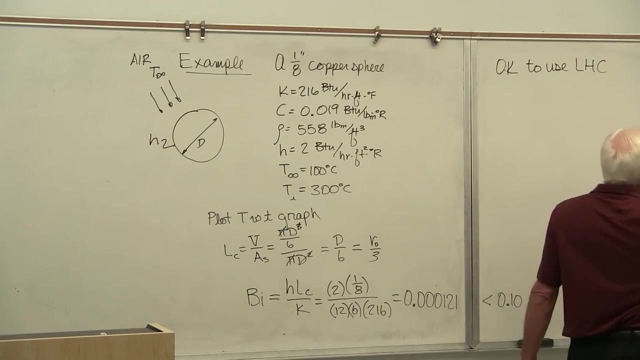 So if I do that, I end up with the VO number of 3 zeros 1, 2, 1.. That's a lot less than 1 tenth, So it's okay to use counting capacity. Alright, so here we go. 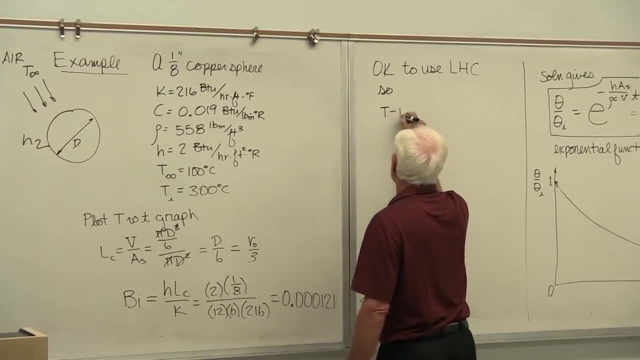 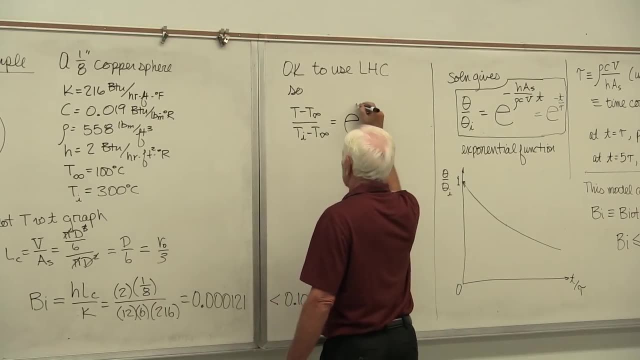 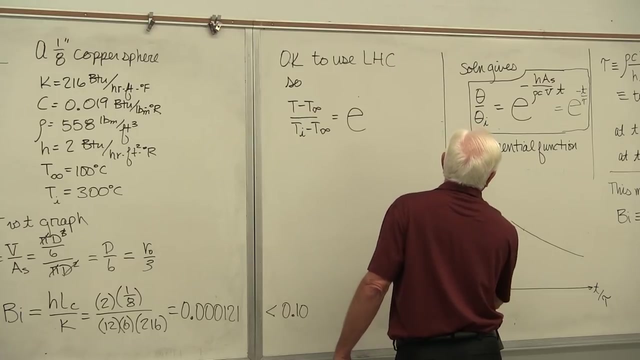 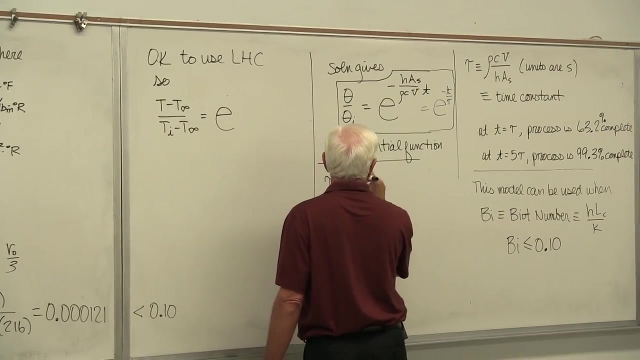 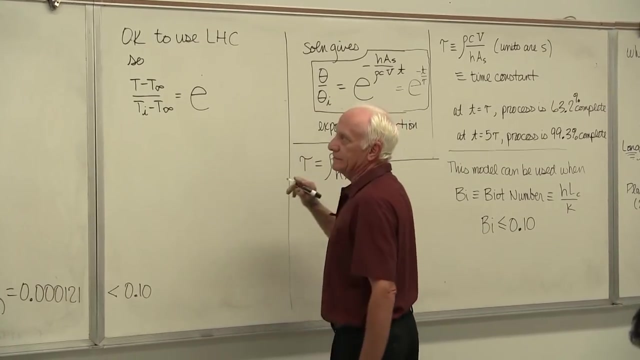 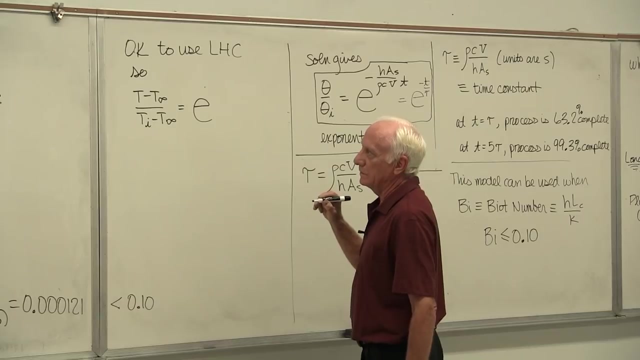 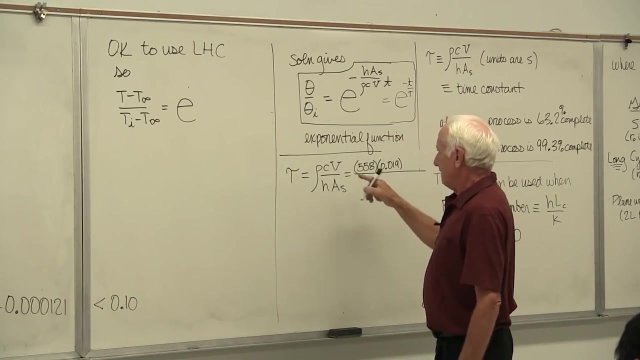 There's the equation. Let's get- we have to get our H data. Let's just calculate that. Rho CV time count. Okay, the density of copper: 558.. Okay, Specific heat: 0.019.. V over, As is L sub C. 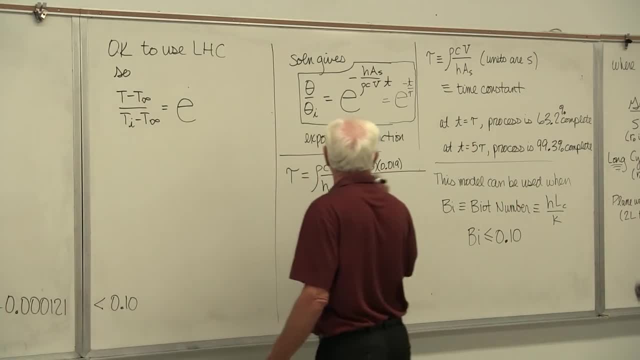 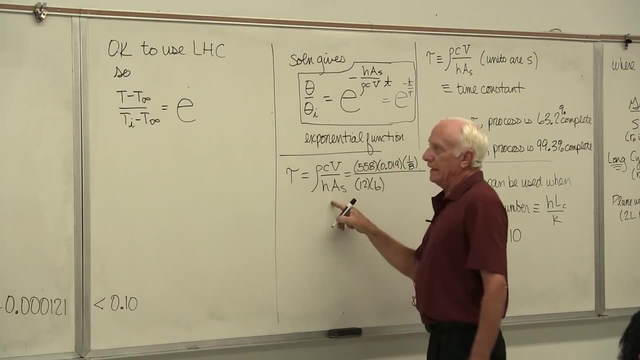 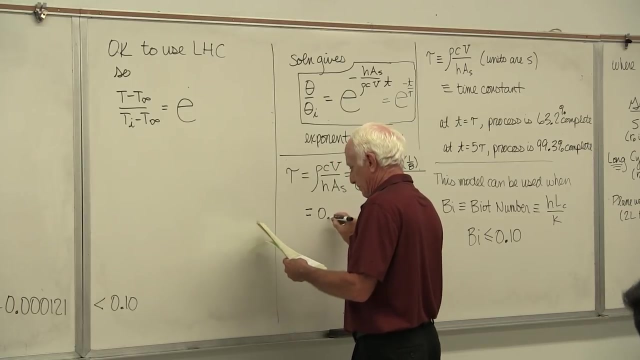 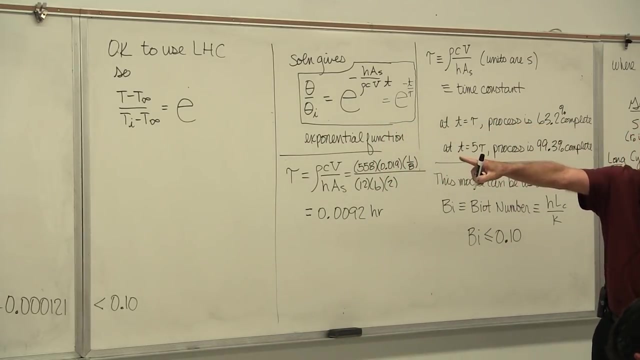 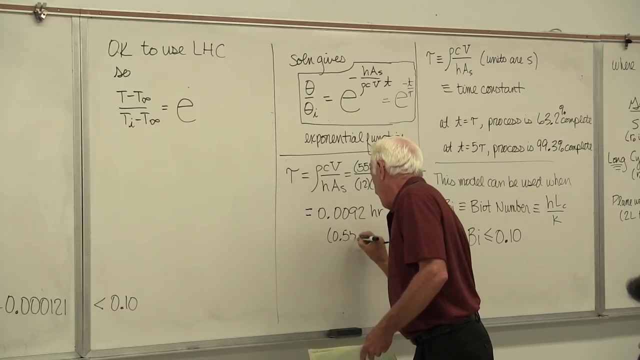 There it is: 1 eighth divided by 12, divided by 6.. H2. Time constant: 0.0092 hours. The answer comes out to be hours, because hours is on the properties over there in the equation, Which is a little more than half a minute. 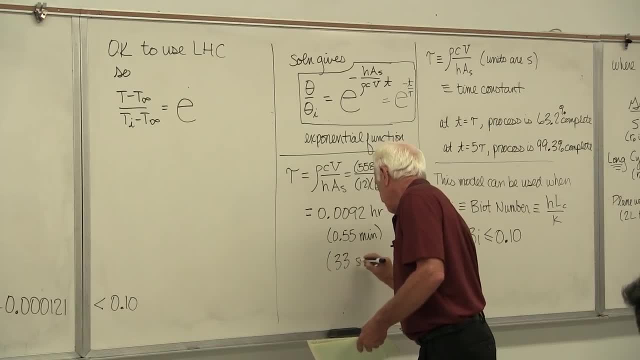 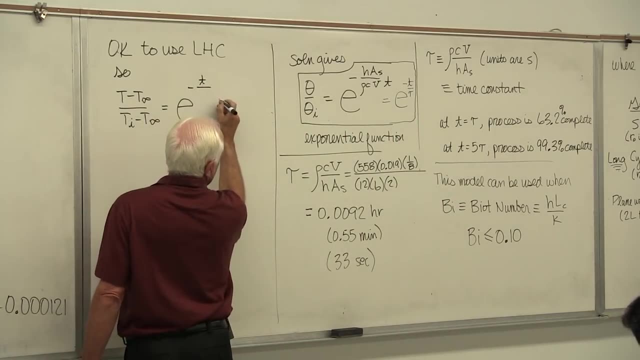 Which is about 33 seconds. So there's the time constant That goes up here, Minus T. We'll put it in hours Minus- I'm sorry- minutes, 0.55.. T is in minutes. Temperature is in degrees Fahrenheit. 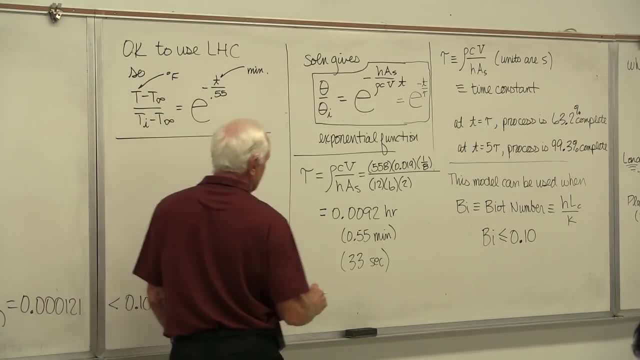 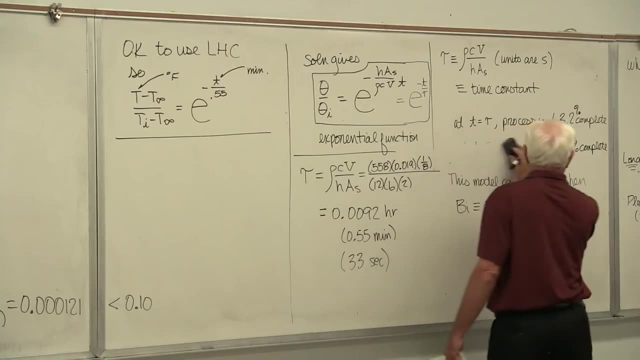 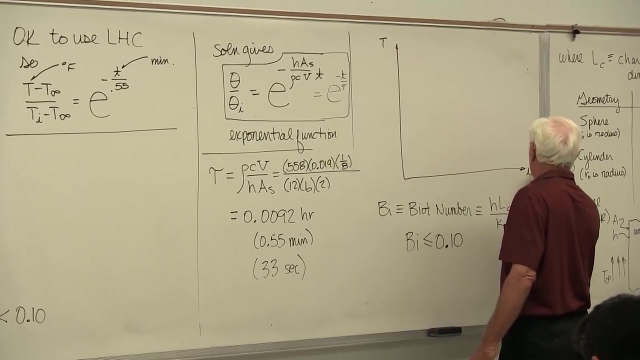 Okay, Now we're going to plot it. I need some space for that, So I'm going to plot it here. Okay, We're going to plot temperature versus time, And I'll do this for I think if I did it for five minutes. 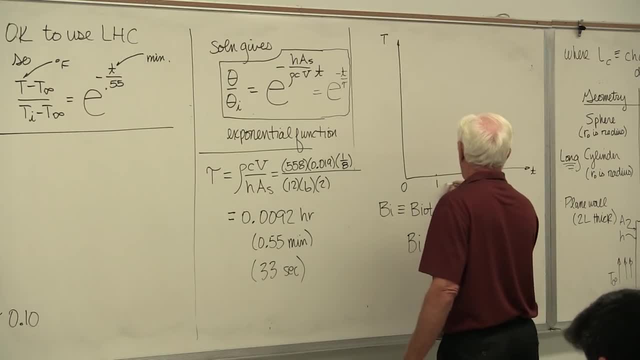 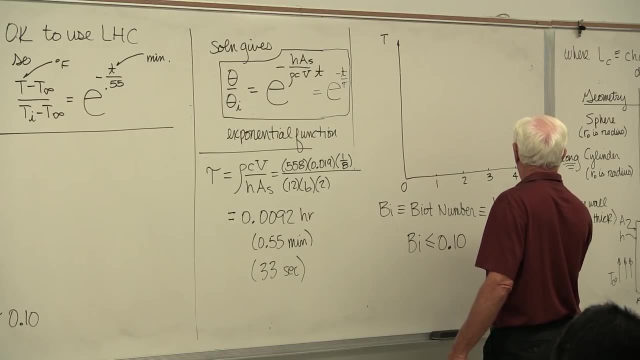 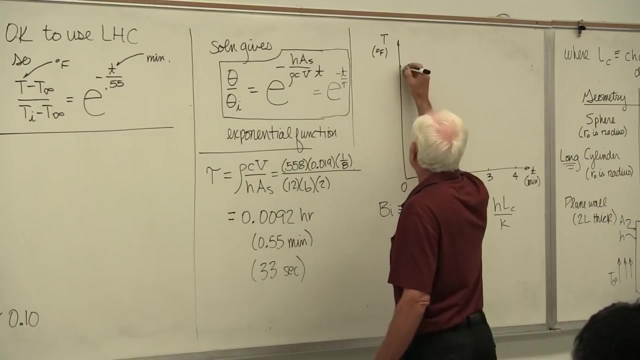 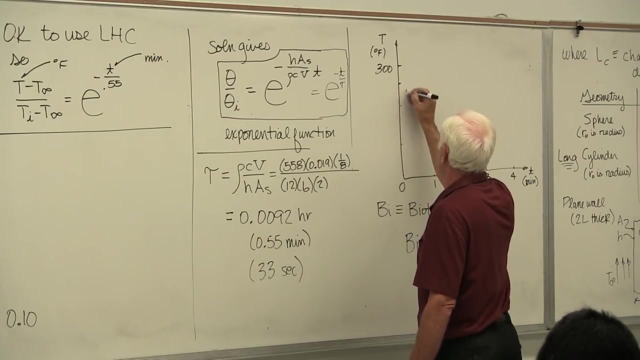 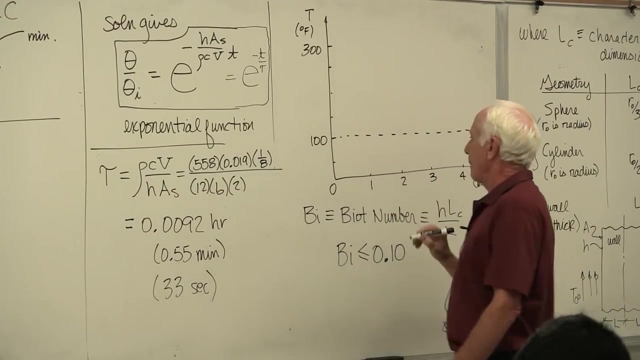 Four minutes: One, Two, Three, Four, Five. And we start out. it said at 300 T initial, And here is 100, 200,, 250,, 150,, 50.. So here is 100, the air temperature. 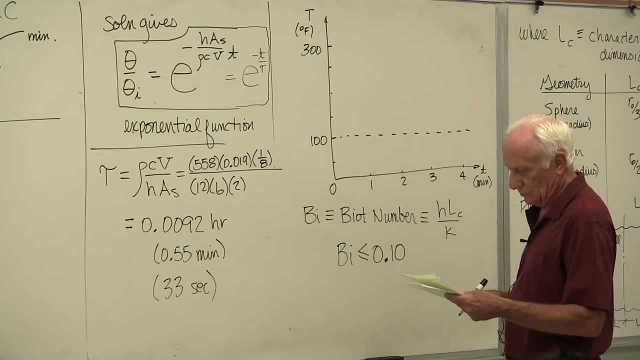 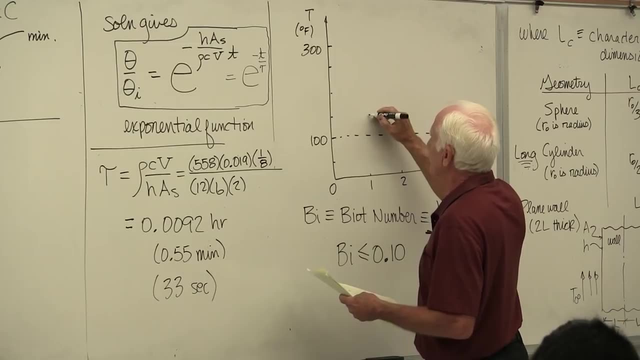 If I plot it, let's see where I get here. After one minute, I'm at about 130.. One minute, I'm at about 130.. There's 150,. 130 is right there. Two minutes, Boy, I'm right down there. 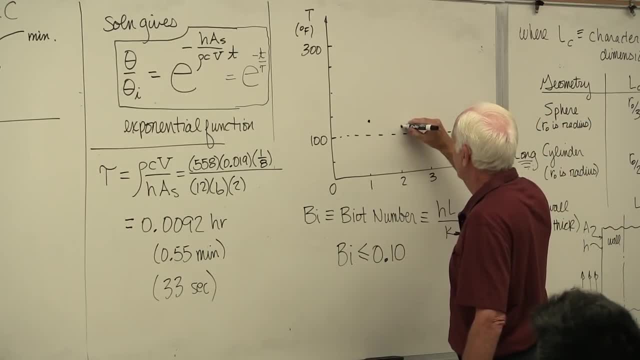 I'm at about 110.. 110 right there, So now I start out at 300.. So if I would plot that, it would look something like this: So there's the plot of how the temperature of the copper sphere varies with time. 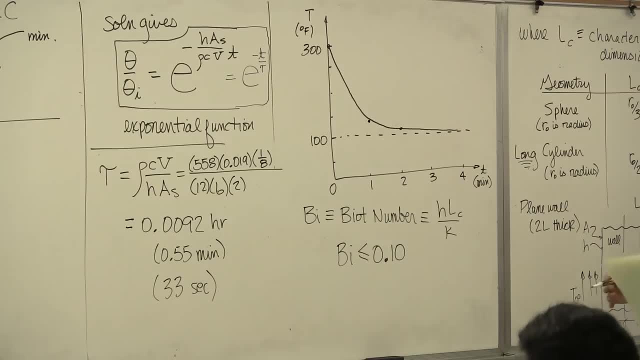 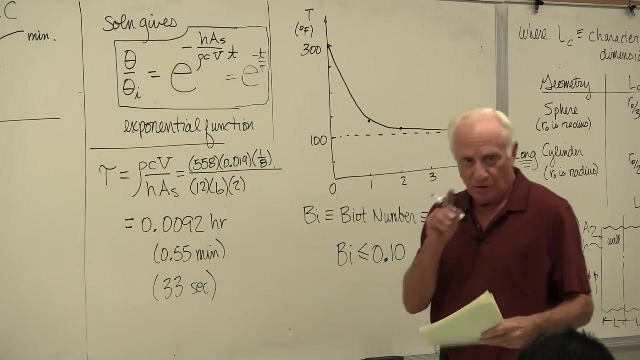 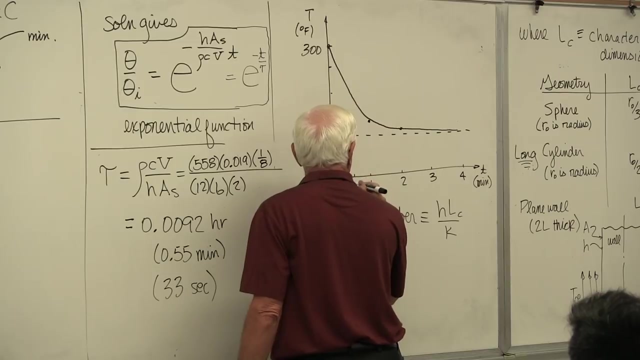 Okay, The temperature of the copper sphere varies with time. If you say what's the temperature of the copper sphere after one time constant, After time equal to one time constant, okay, 0.55 minutes, 0.55 minutes, what's the temperature? 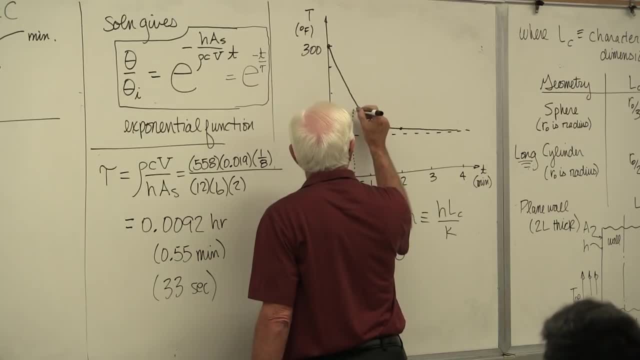 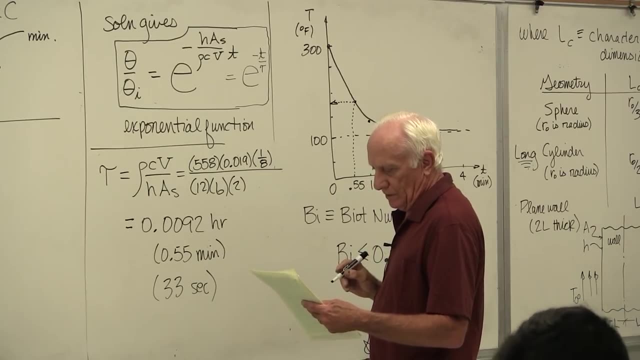 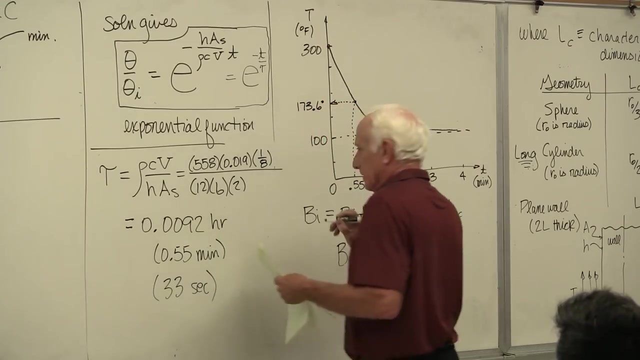 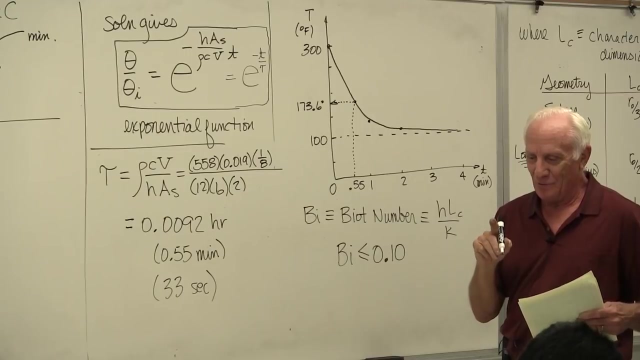 of the copper sphere. If you plug in the equation you would get an error 173.6.. Wait for five time constants. Five time constants. That's the integer rule of thumb. If you want to wait, wait five time constants five times 0.55.. 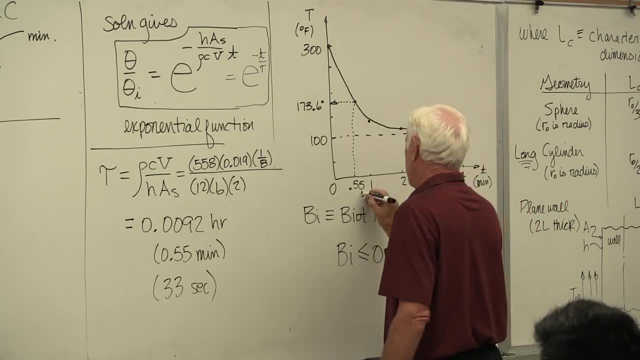 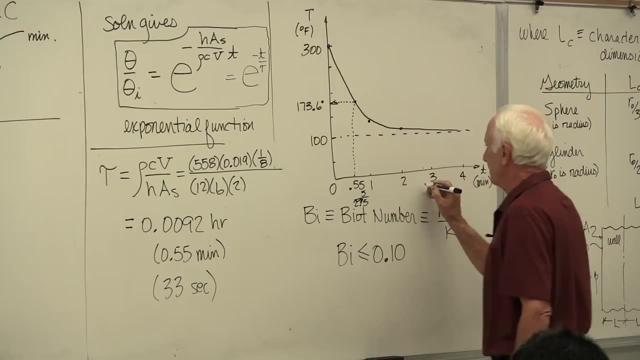 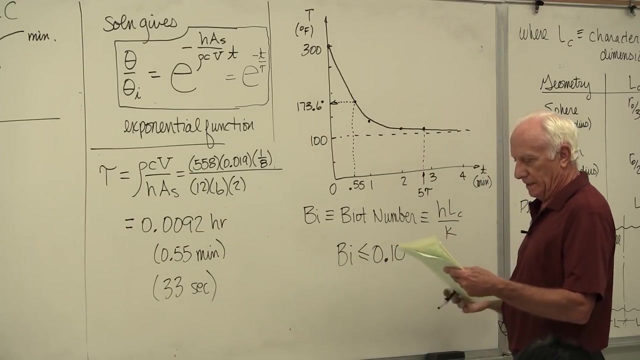 Here's five time constants. Okay, So five, 25,, 25,, 27,. all right, that's minutes, 2.75 minutes out here. This is a five time constants. The temperature at that particular point after five is 100, I'm actually didn't get that. 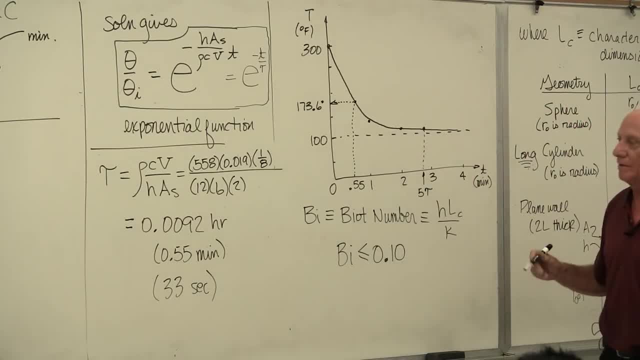 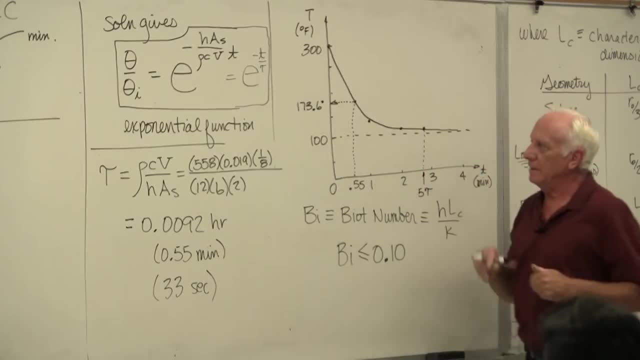 but you can get that It's very, very close. Well, I can tell you this: It's a 90,. what 99%? What's the difference here? 200, 99% And two degrees, it's about 102.. 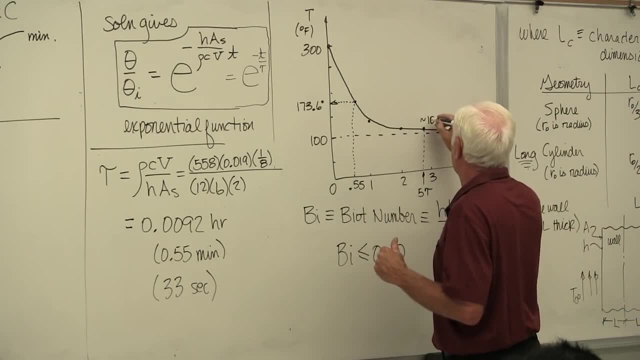 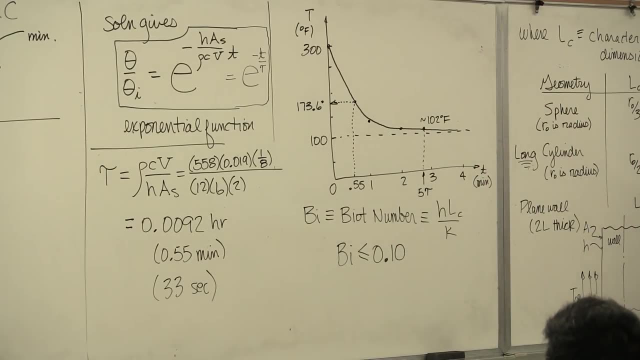 It's about 102.. That's really close to the air temperature. now, If I wait five time constants, I'm home. that copper sphere is almost at the air temperature. It's within two degrees of the air temperature. That's the rule of thumb for five time constants. 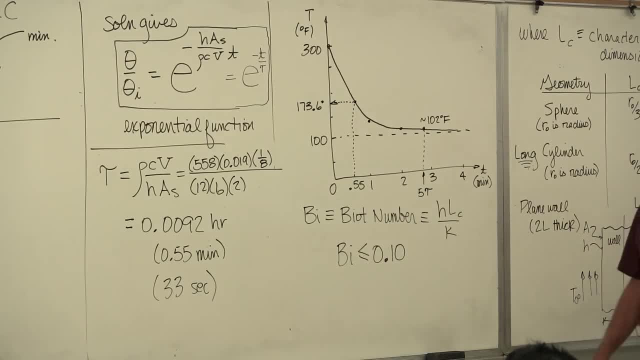 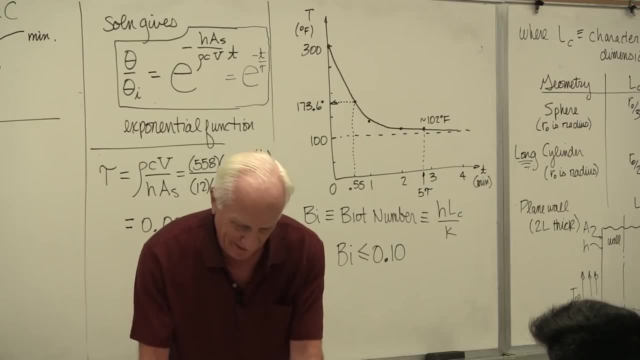 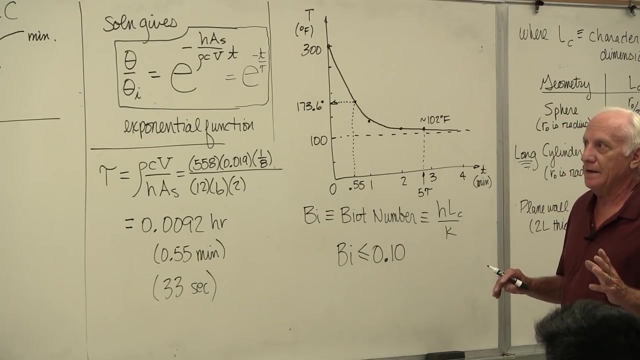 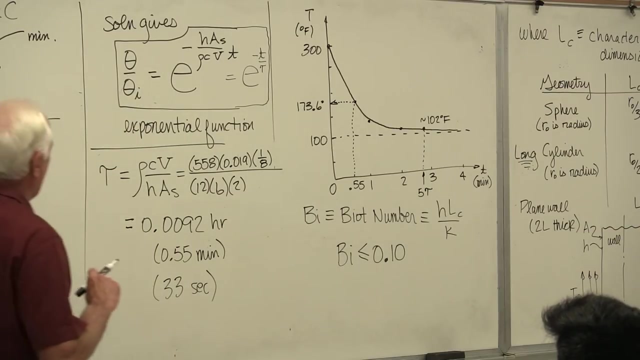 All right, Thank you. Okay, so there's the plot. If I change anything, the rules can change. Let's say I double the diameter now to a quarter inch. a quarter inch, a quarter inch. Double the diameter. Where's the diameter? 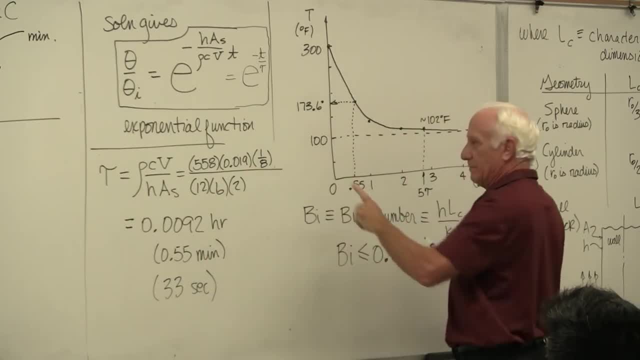 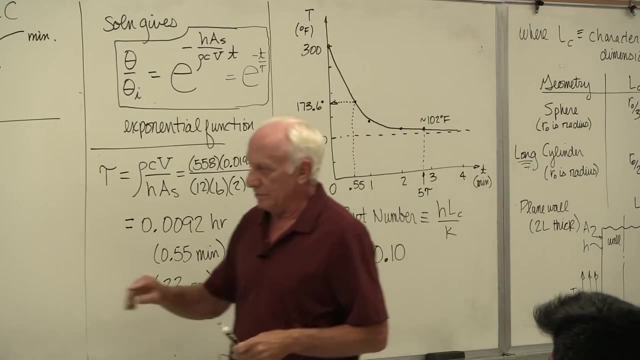 Right here, Where's the diameter on the BO number? Right here. Okay, Is the BO number still okay? Okay, double that number. Oh yeah, it's still okay. It's still okay. I can still use one heat capacity. 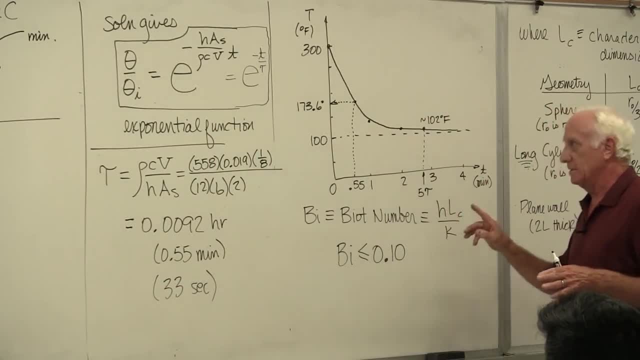 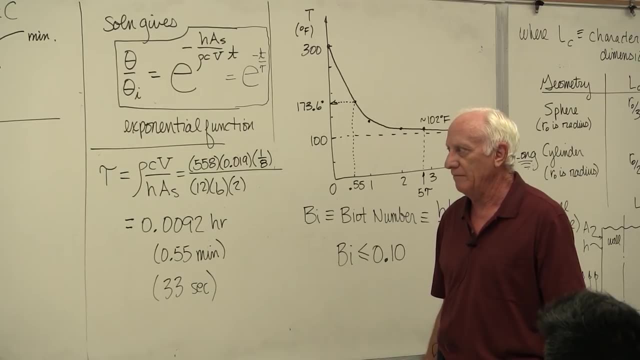 What do I change in that graph? What changes is I change tau. Double it Now tau 0.0184, 0.0184.. Don't forget: The bigger the tau value, the currier The curves go up. 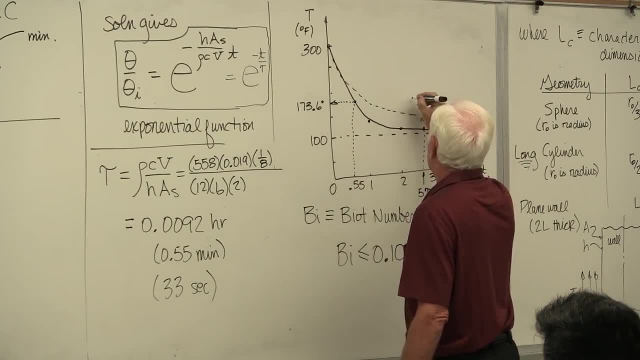 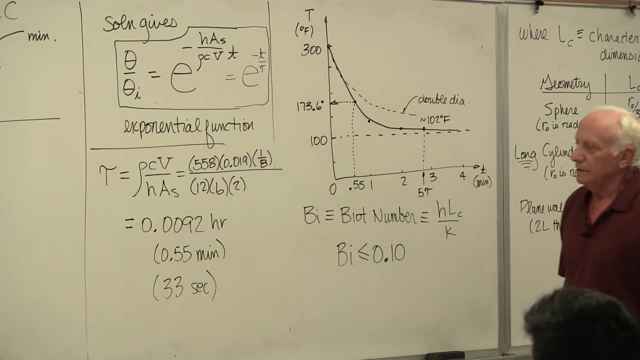 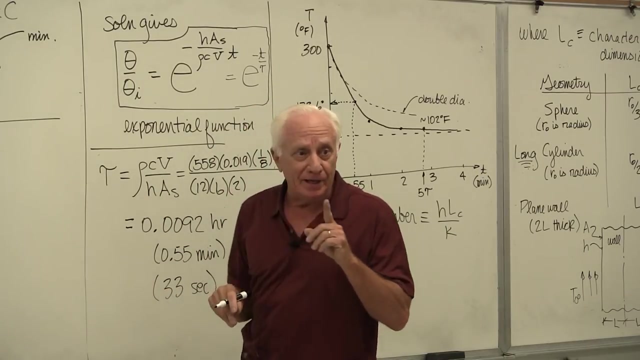 So the new curve now looks like this: Double, Double the diameter, Say well, okay, You know what I'm going to do. I'm going to double the H, I'm going to double H. Okay, Go ahead and double H. 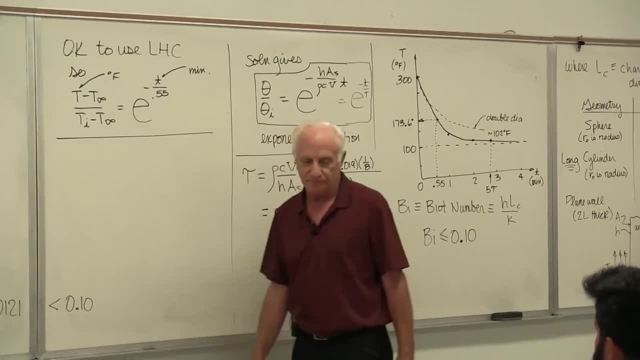 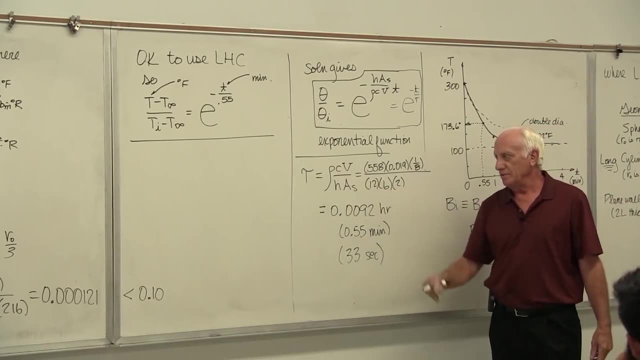 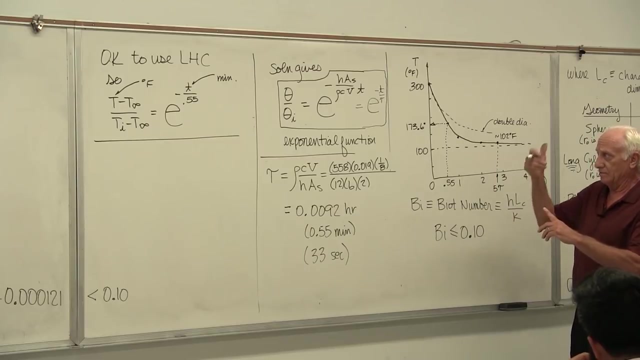 It's still way small. I can still use lumped heat capacity. I go over here. What changes I double H. If I increase the denominator, the portion becomes smaller. Tau is smaller. Remember the curves: Tau goes gets bigger, curves go up. 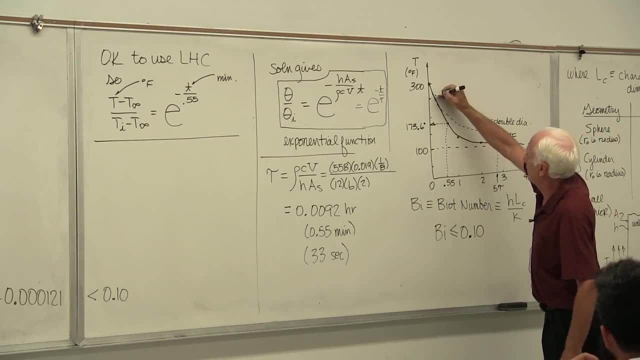 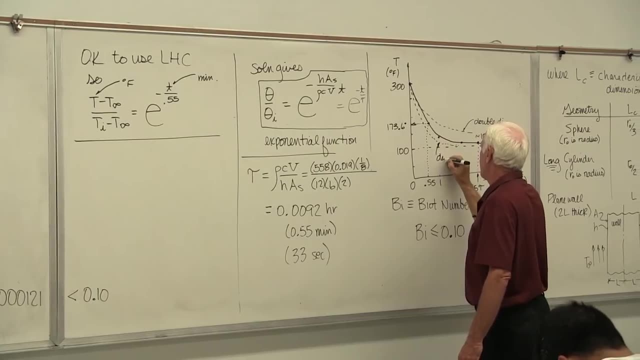 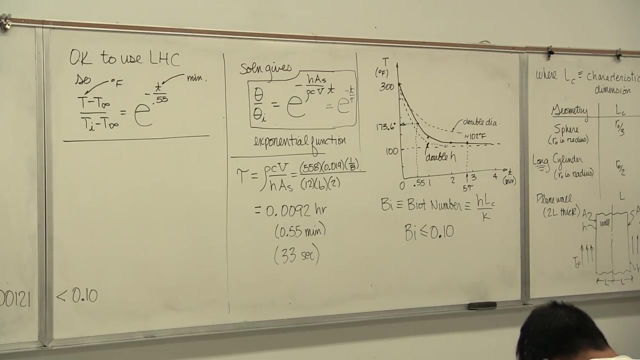 Tau gets smaller curves go down. So now my curve looks like this: This is double H. Of course it cools faster as you turn the fan on. Does that make common sense? Sure, it makes common sense. that way, If you make it more massive, sure it's going to cool slower. 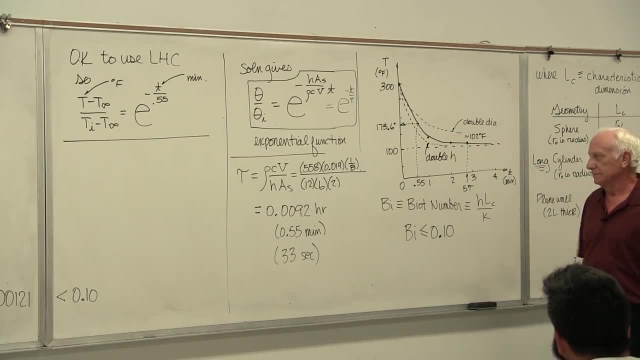 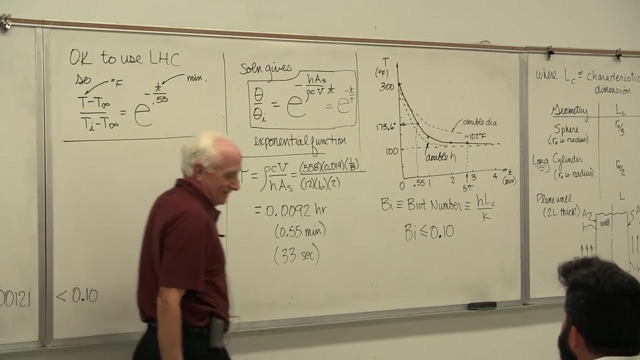 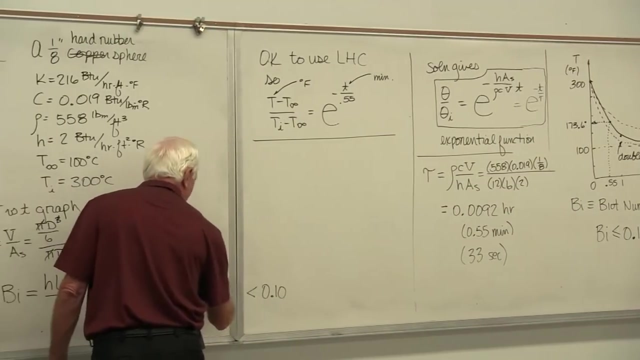 So these aren't surprises, They're somewhat common sense. Okay, Now I change the material. I go to the back of the book, Hard rubber. All right, When I do that, my VEO number .261.. Voila. 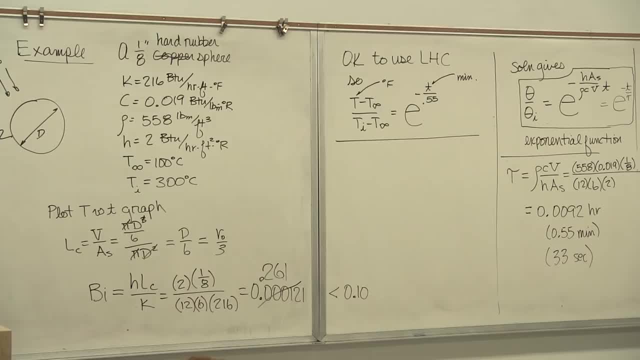 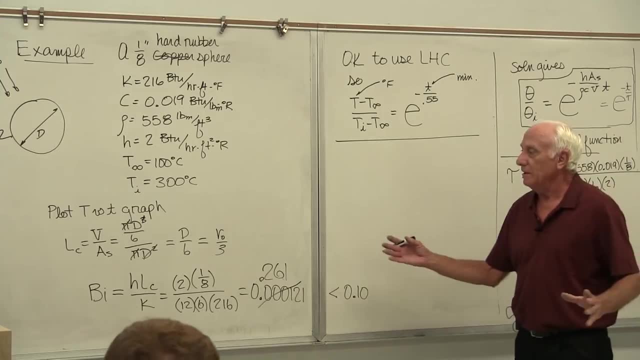 I cannot use lumped heat capacity now. I've got to use the more difficult approaches we're going to look at Friday. So any of those things could change. But H can change, K can change, I can change, C can change. 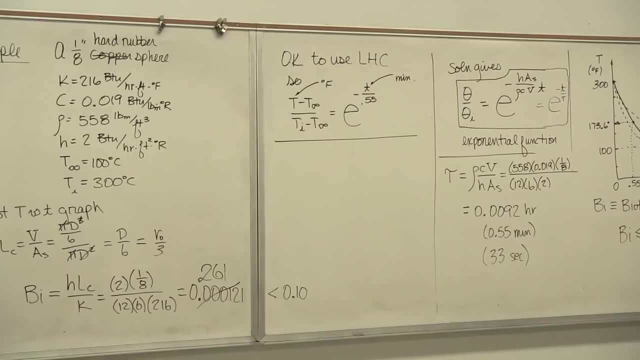 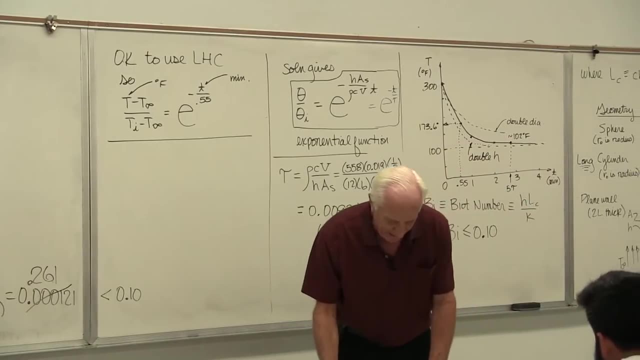 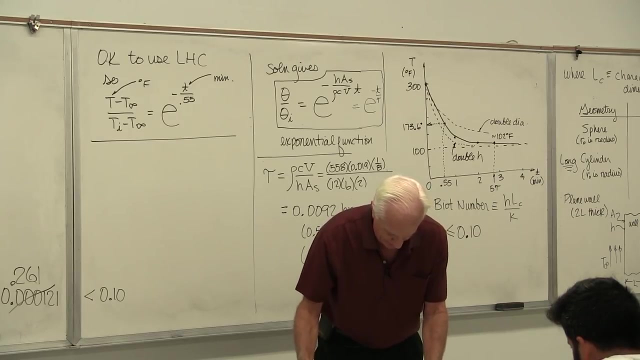 Rho can change, So everyone's different. There's different curves on here depending on what you put in those numbers right there. Now, if you want to find the heat transfer that's taking place in that time, we can do that. Let's see where our heat transfer there is. 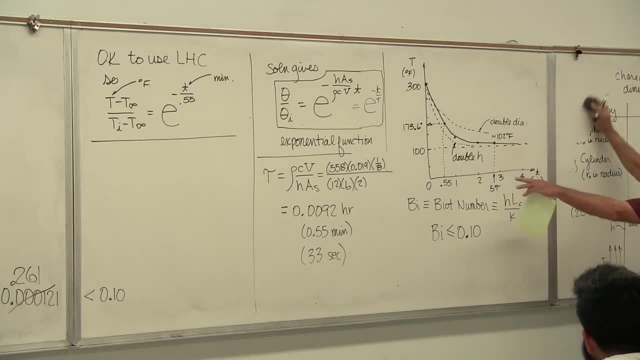 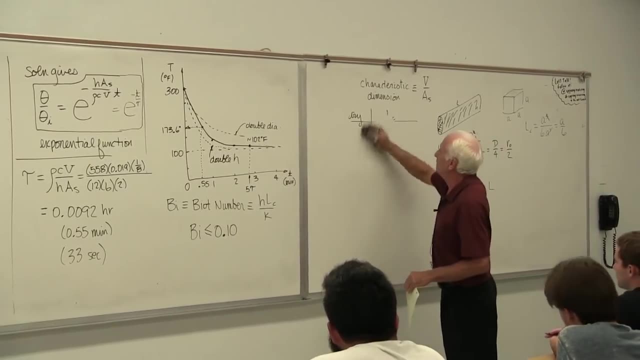 I'm going to put that over here, Because this gives us temperature. Don't forget, in heat transfer, we're interested in two things. We're interested in the heat rate, Q, and the temperature, T. Okay, So far, heat transfer. 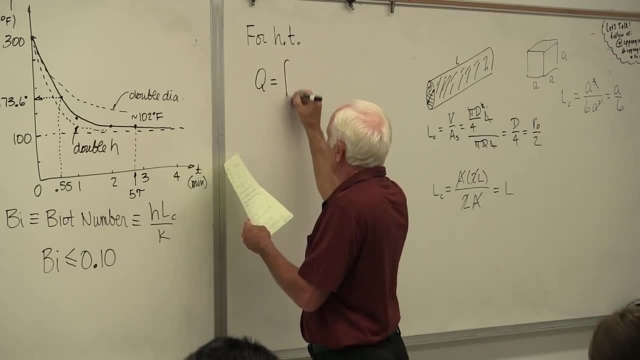 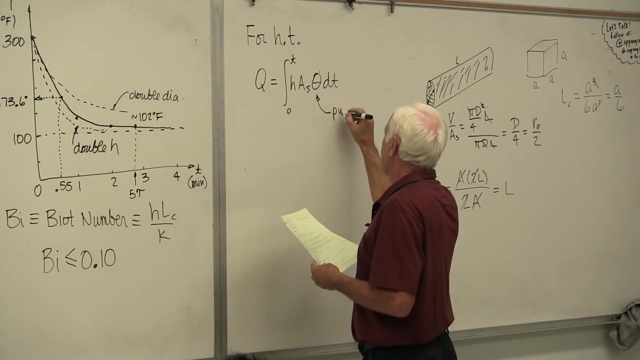 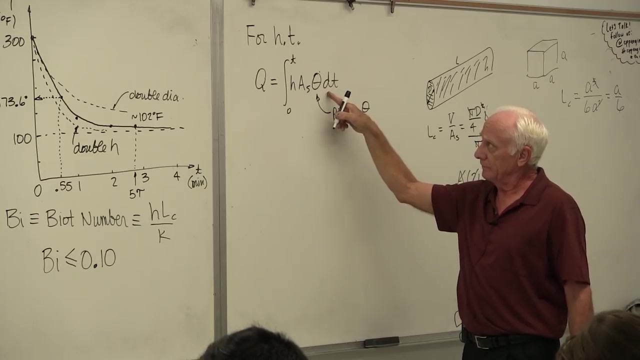 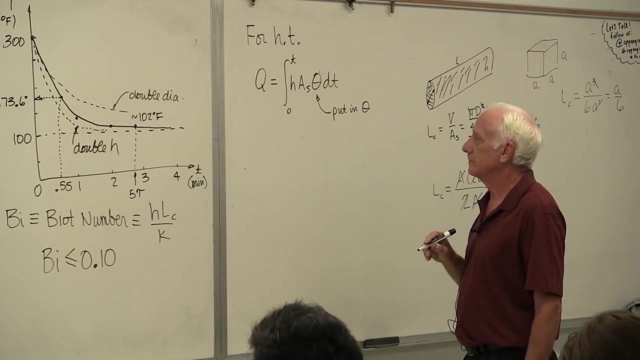 Q is equal to integral of zero to T. H A, S, theta times, dQ. This is convection, of course. H A T minus T, infinity. Integrate it over a time interval Zero to T. This guy right here is in watts. 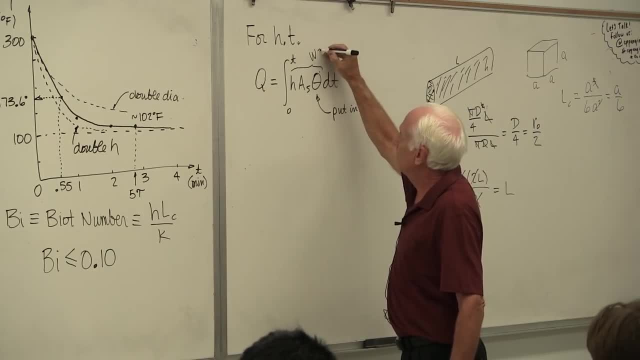 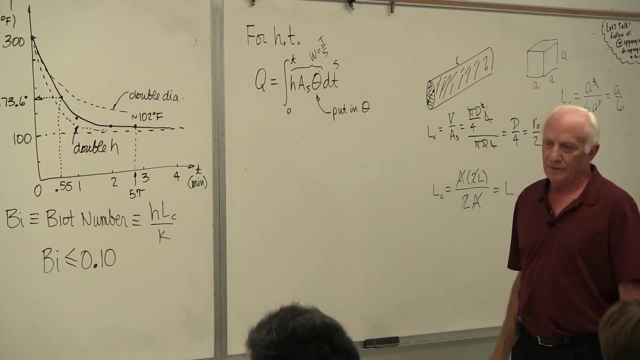 H, A, delta, T. What's a watt, A joule per second? Multiply that by time in seconds and what do you get? You get joules. That's why it's a capital Q. This is a lower case Q. 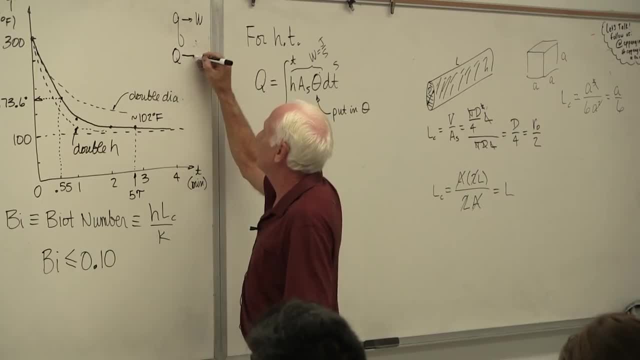 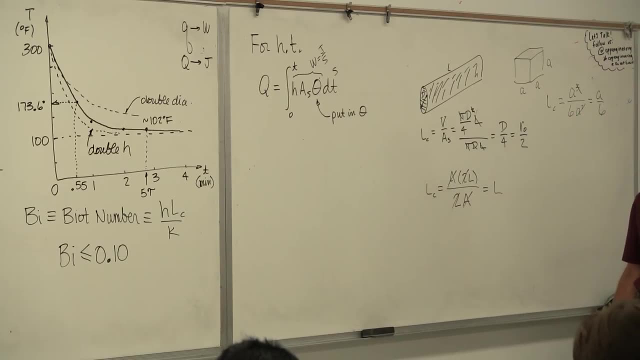 What's that in? That's in watts. This is a capital Q. What's that in? That's joules, Like a thermo Capital Q is in the thermo test And it's in BTU per hour or joules. 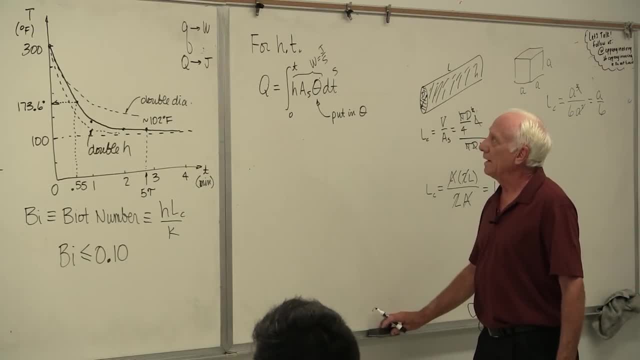 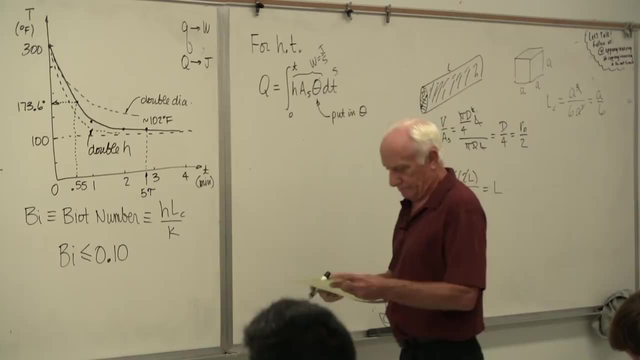 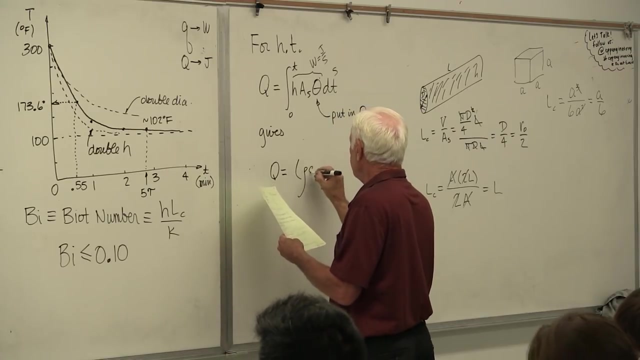 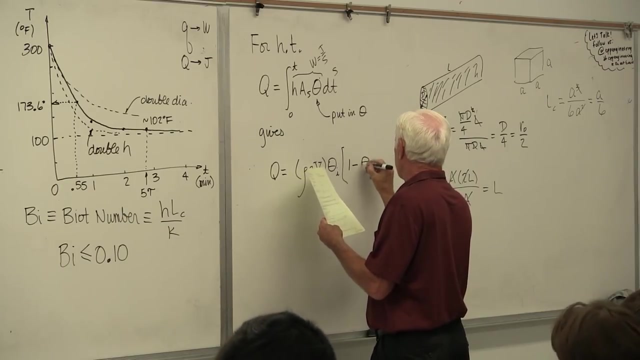 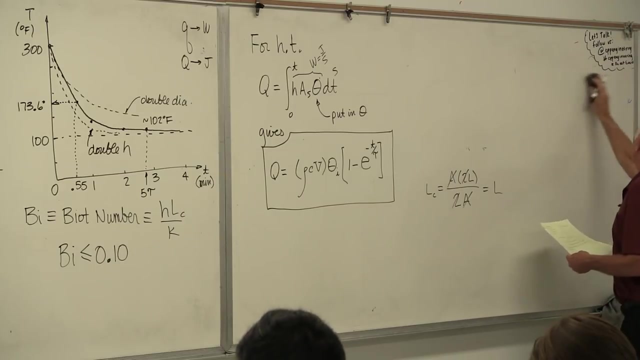 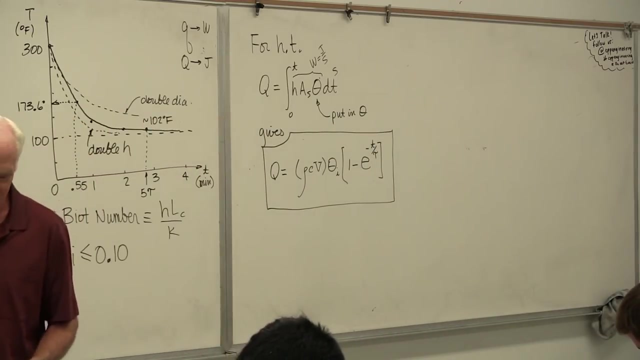 BTU. Okay, Put that guy in a box, Put him in here, Integrate it and you end up with Q. Okay, so now we have two box equations. One gives the temperature at any time And the other one gives the amount of heat. 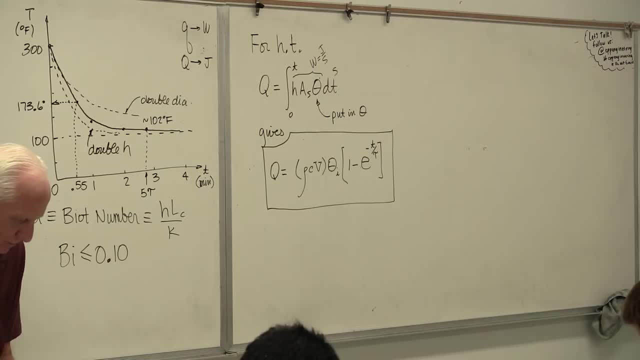 that's been transferred over that time in joules. In joules, Theta I is TI minus T, infinity. Okay, so we'll. I'm going to pass out this special computer bubble now, But we'll pick this up again on Friday. 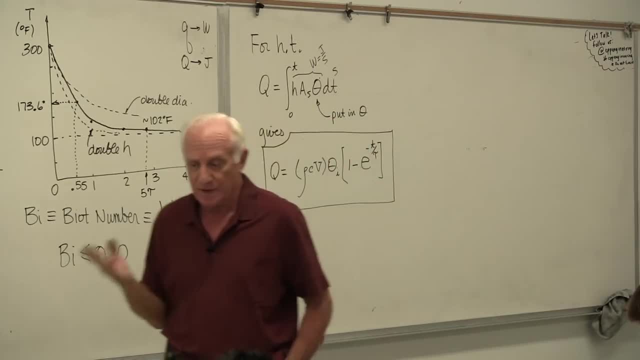 and we'll say what if the BO number is greater than 0.1? And we'll do it again on Friday If you came in late. I mentioned don't look at blackboard for homework due dates. I'm going to change it tonight. 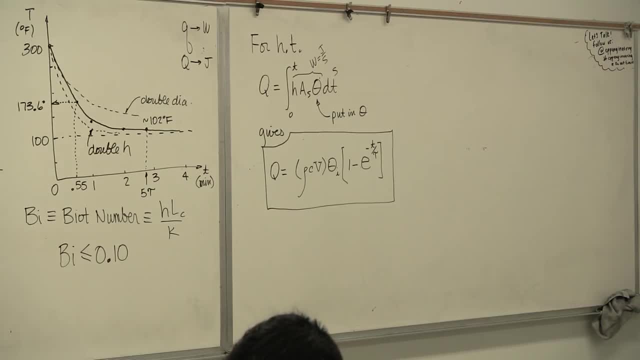 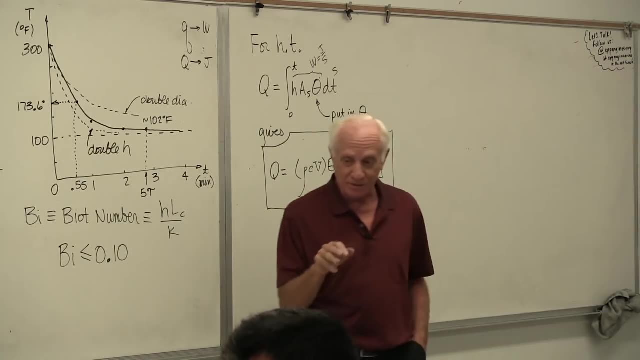 But just so you know, chapter 4 is due Monday. Special problem: computer problems are Wednesday. Next Friday. this Friday is chapter 5 homework, So three things due next week. Okay, so let's go through the computer problem. 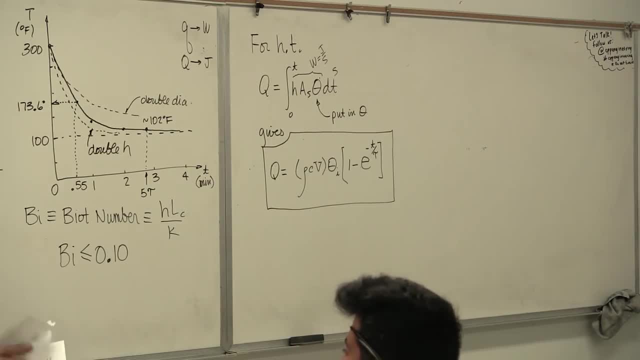 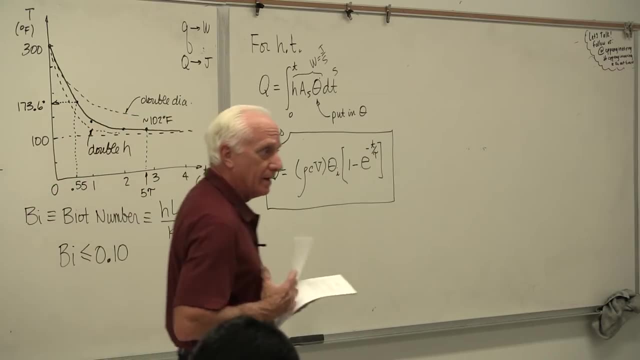 This is from chapter 4.. Okay, so over on June 10th you have to do I'm discussing the passes from one week to five months. How many years do you think you got on the computer to have? So these classes are going to break out on a Friday. 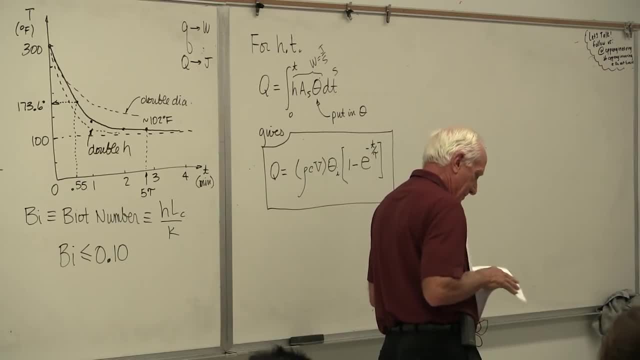 I'm going to go through them and I'm going to- or I'm going to- just wrap it up here and then hopefully you can come back and ask about something else on later Tuesday. So again, since you pay even less for the AC class, 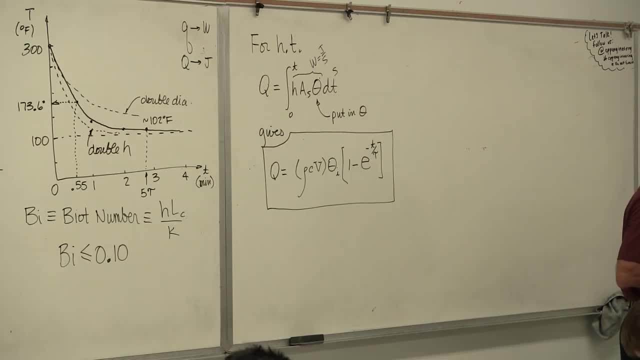 you have to make sure that we get to three weeks of� west end. All right, so the PAP size is five and 1차 and the 1var is 164.. So basically, when you pull this, you're going to go straight up. 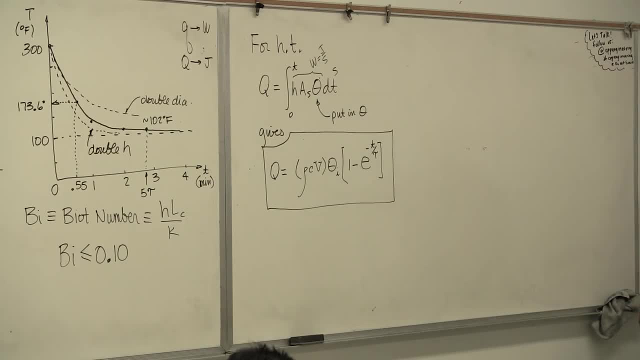 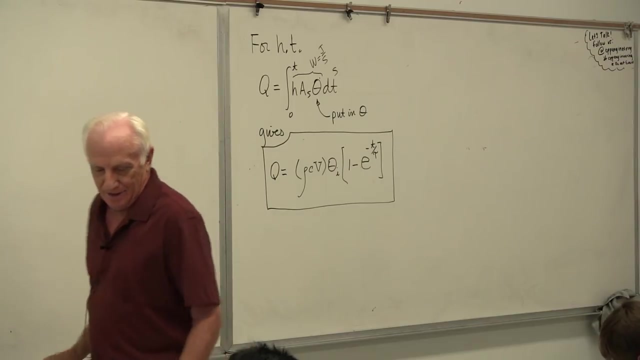 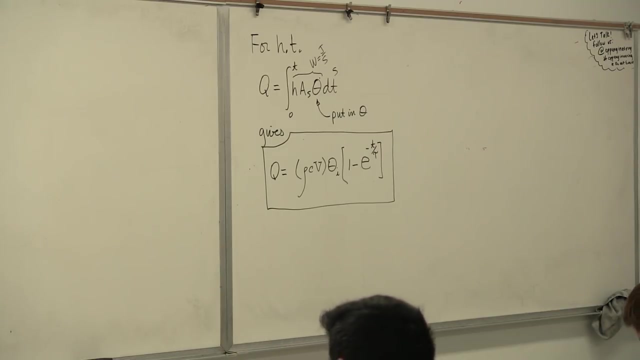 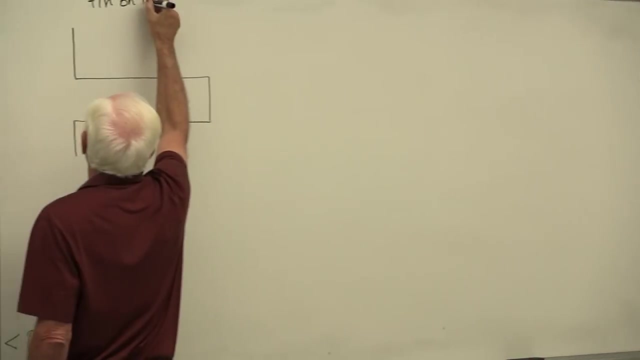 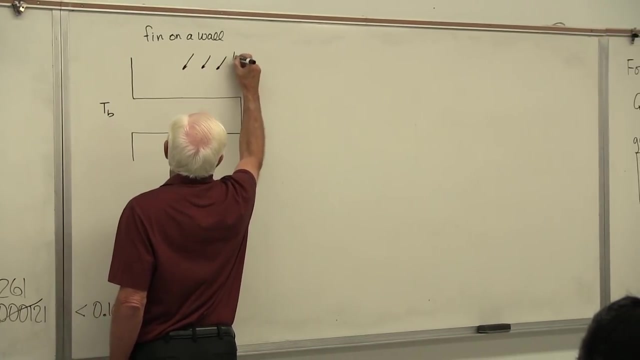 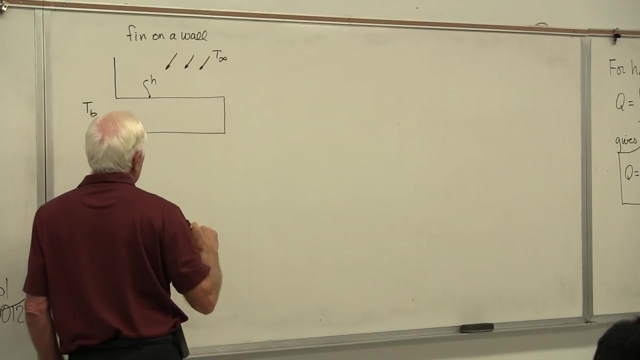 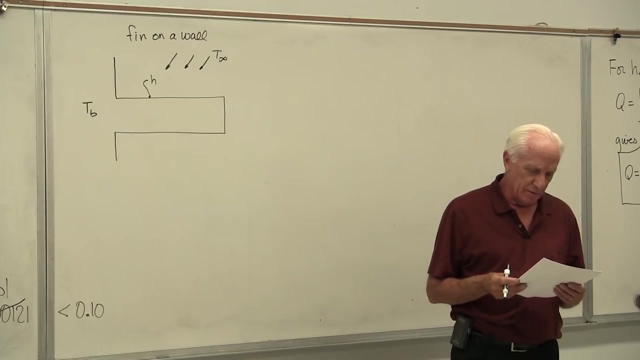 Okay. so the computer problem is we've got a fin attached to a wall, T, base T, infinity convection coefficient H on the surface and we know the temperature of the base of the wall. We know the temperature is air air stream, We know the convection. 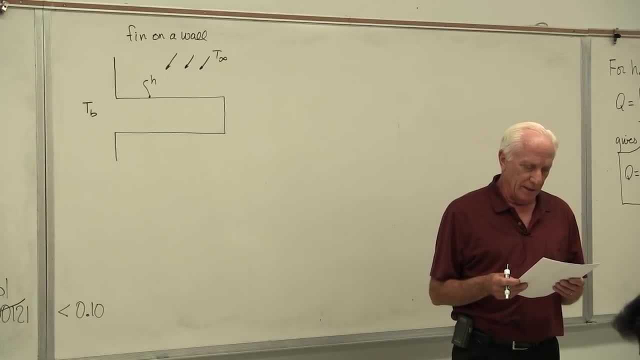 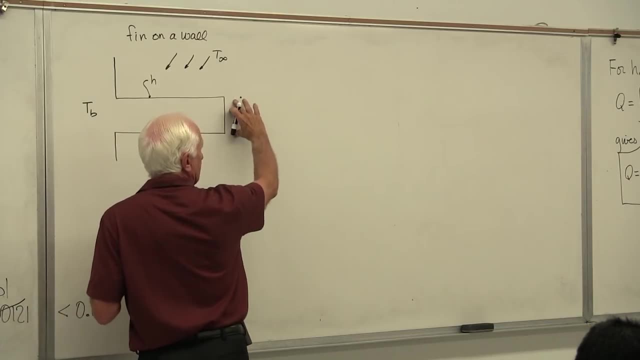 coefficient. We know the fin has a length of four centimeters and a thickness of two. So four centimeters. here's L coming out. The thickness here is two. Two is this dimension. four is that dimension We're supposed to model that? 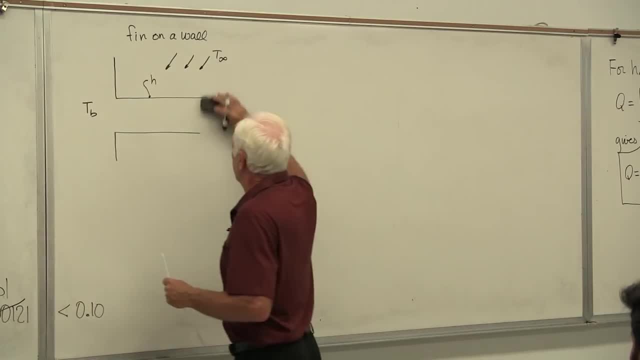 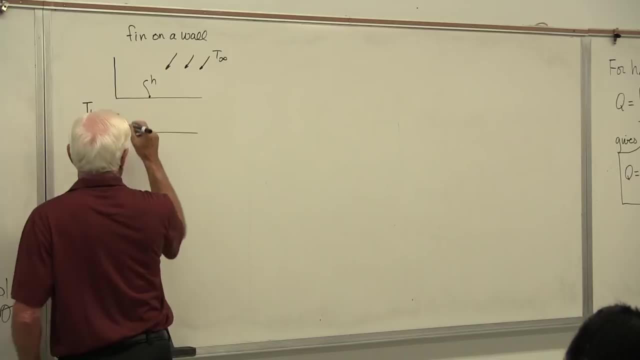 by a nose and heat conducting rods. So, all right, we're going to tell you what delta X and delta Y are. One centimeter, so it looks like this. So there's two, and this is four. One, two. 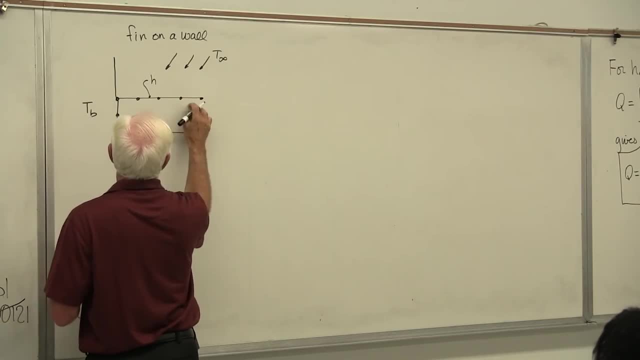 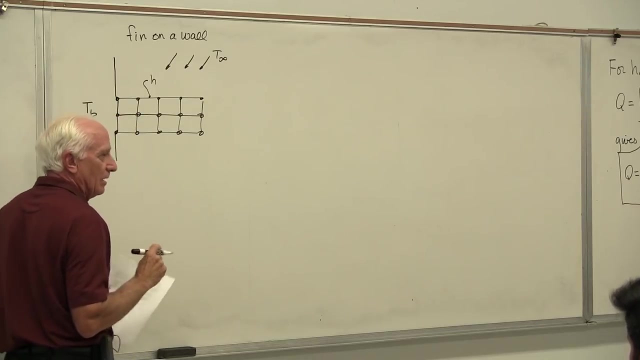 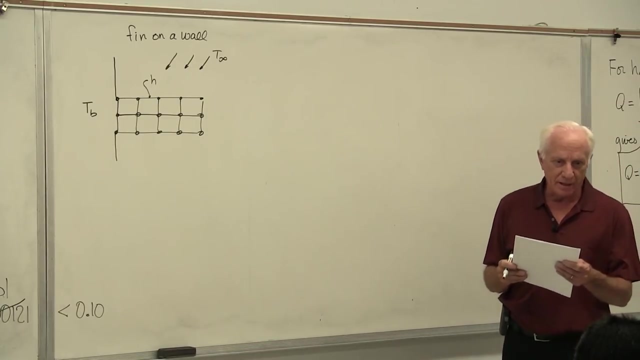 three, four, Four of one, two. So I'll draw the model for you here. Okay, Okay, Fifteen. So part A: find out how many nodes have an unknown temperature and write a nodal equation for each one of those nodes. 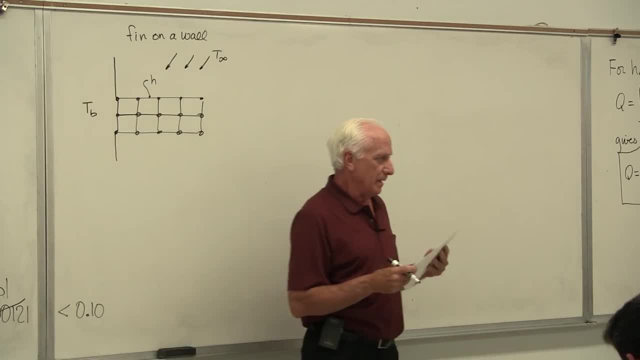 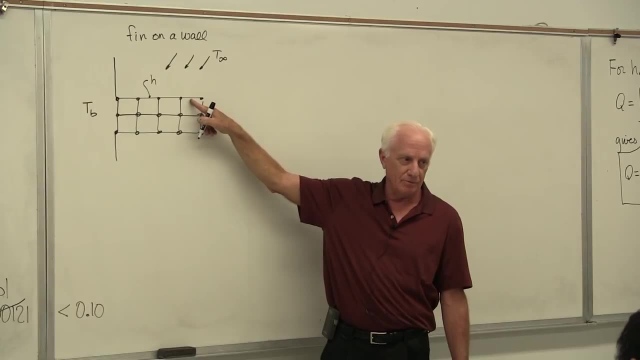 So you go to the table in chapter four. For instance, the node where my finger is right now, that's a node on a convection boundary, That's in the table, A node on a plane boundary. where my finger is, That's a node on a corner convection boundary. 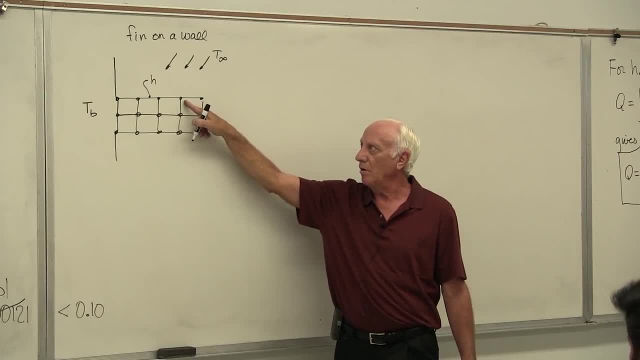 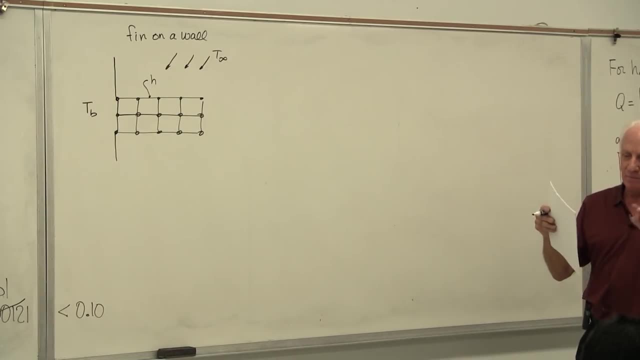 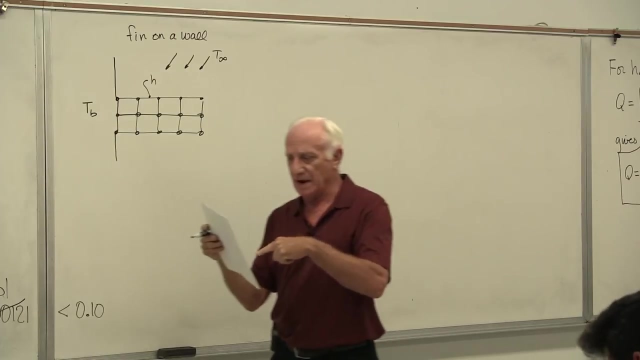 convection: boundary Corner: plain wall, plain wall. So look at that table, take out the right equation, put the numbers in and write it down, So you'll have all the equations under part A listed with numbers where you can find those will be a function of all the temperatures: T2, T3, T4, T5, so on and so forth. 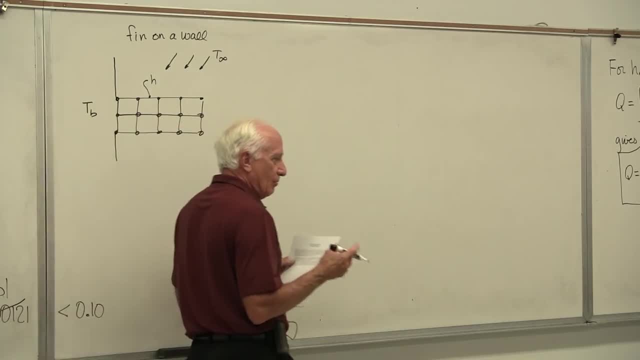 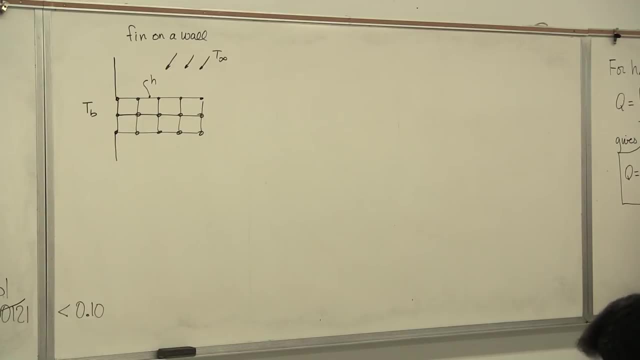 B: solve those equations for the unknown temperatures. We did this in class as a model. Use what I did in class as a model for how you work this problem. I'll make something up If you've got nine unknown temperatures and there's numbers. if you've got nine unknown temperatures, there'll be nine equations for those temperatures. 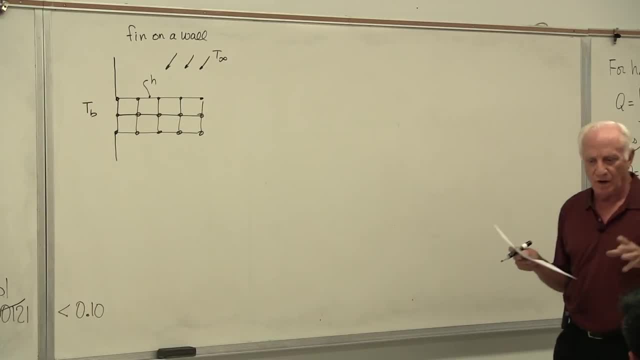 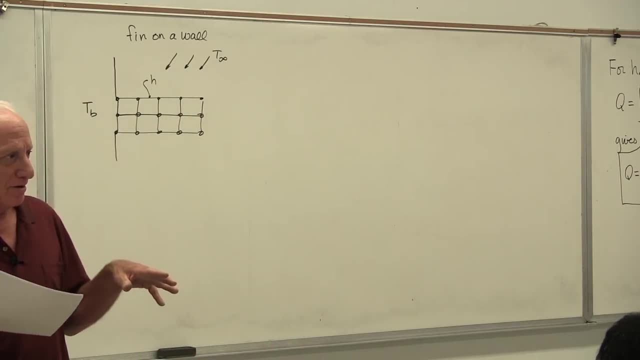 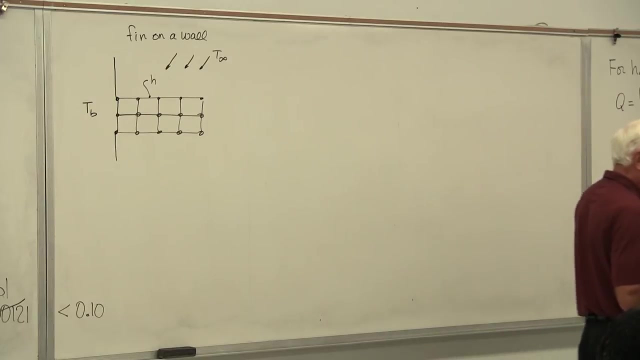 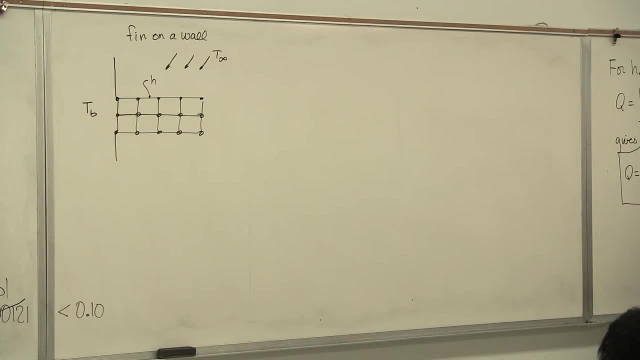 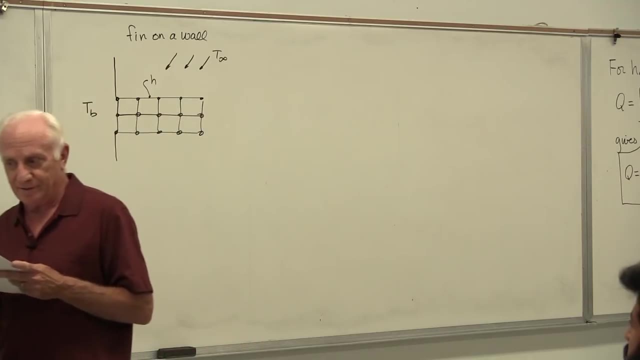 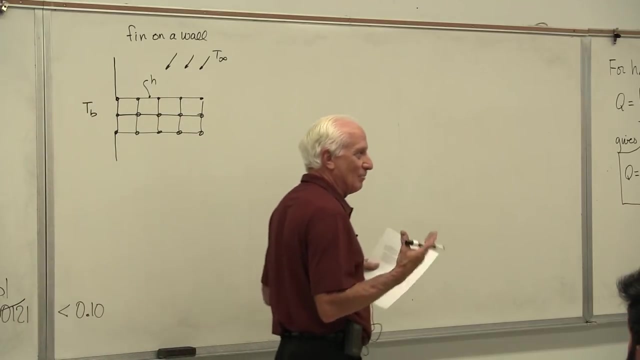 If you do it by Excel and MATLAB, attach it to your problem. the hard copy print out. the hard copy print out. If you do it by your TI, I'll see you in my office in the next two weeks after you've turned in and you'll show me on the TI. 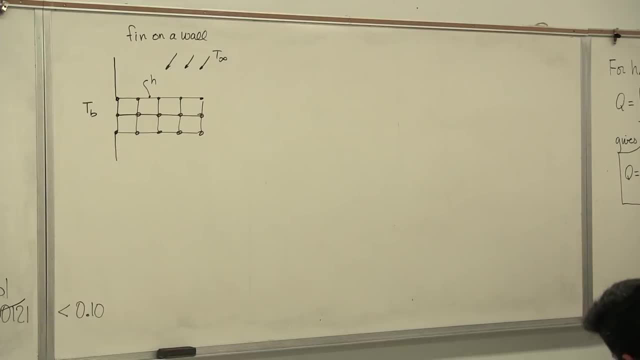 what you did. You might want to save those equations. if you do solve them, Save it because you'll need to bring them by my office for your TI. and you punch this stuff in. I'd look at it and see if that's what you got in the paper. If you do it by Excel or Matlab, a 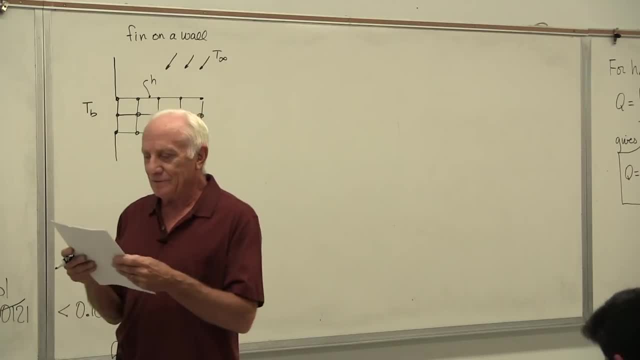 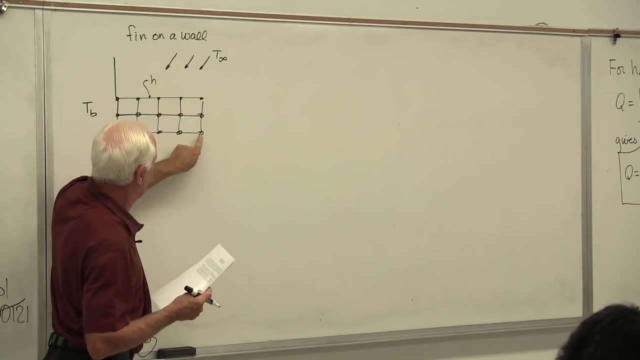 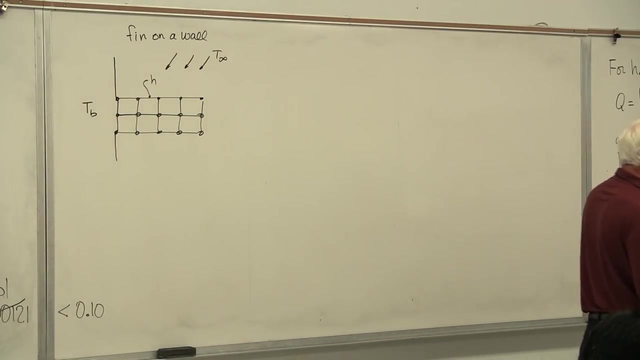 hard copy attached to it is fine. After you've done that, you find what the tip temperature is, the average. See, there's three, One, two, three. Here's the thin tip. Three temperatures averaged in part C. Compare that to table 3-4 in your textbook, because table 3-4 is 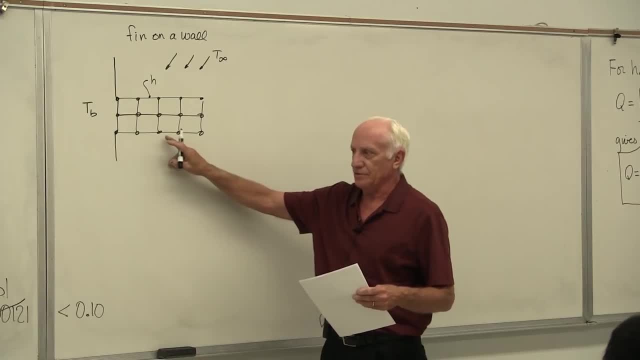 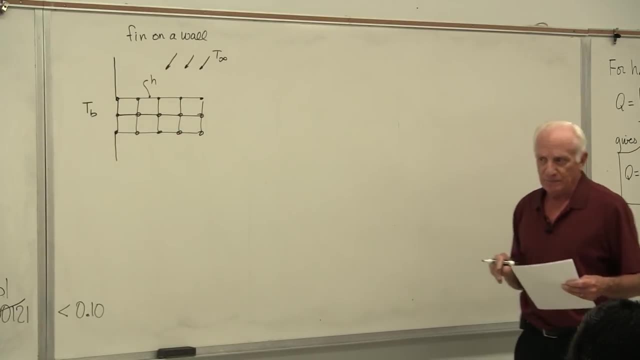 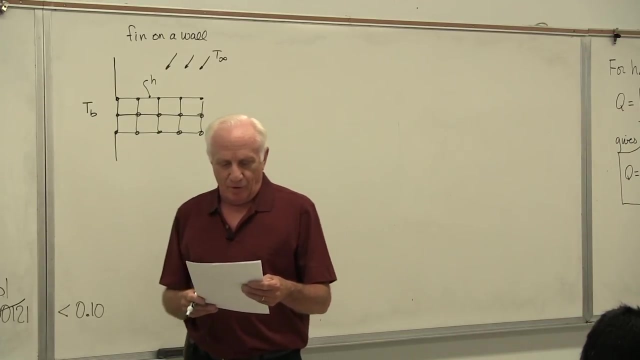 chapter 3 and chapter 3 is one-dimensional heat transfer. Temperature's only a function of X In this problem. in chapter 4, it's a 2D problem. Temperature's a function of X and Y. Okay, Part D. Find the heat transfer from the fin and compare that to chapter. 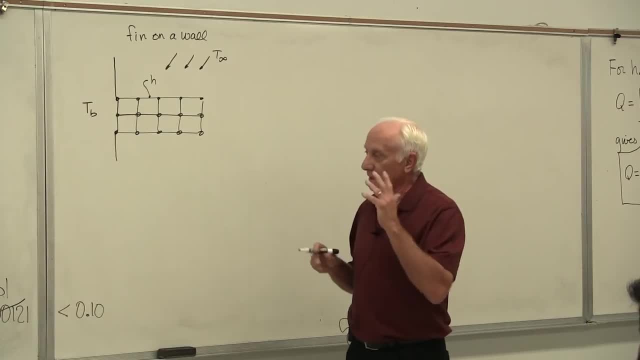 3. Chapter 3 results in one-dimensional heat transfer. Okay, How do you find- now? we've already found the temperatures over here- How do you find the heat transfer? Okay, To find the heat transfer, let me see your class notes from that, What we did in class in chapter. 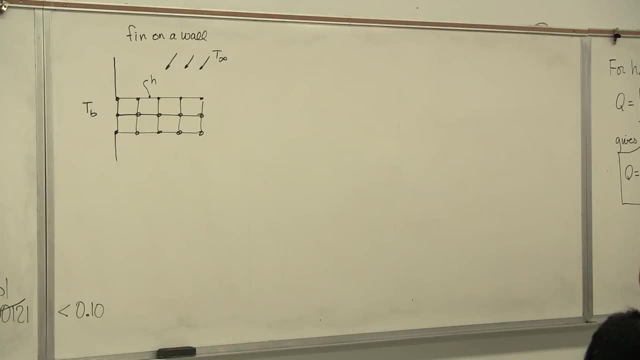 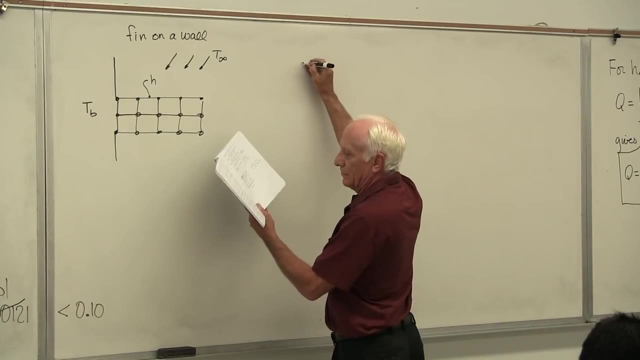 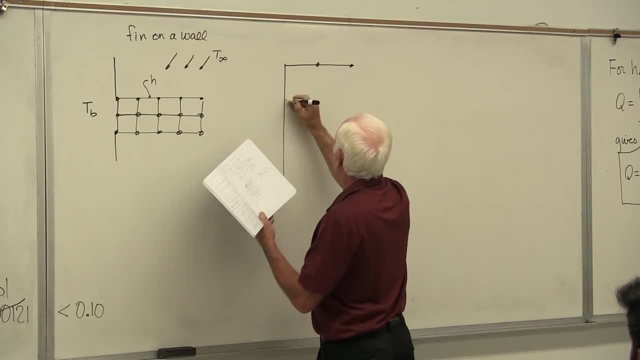 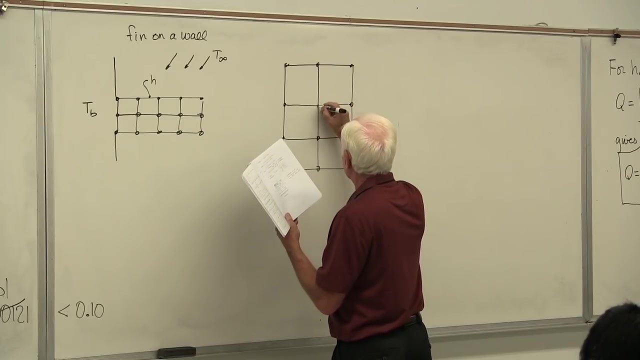 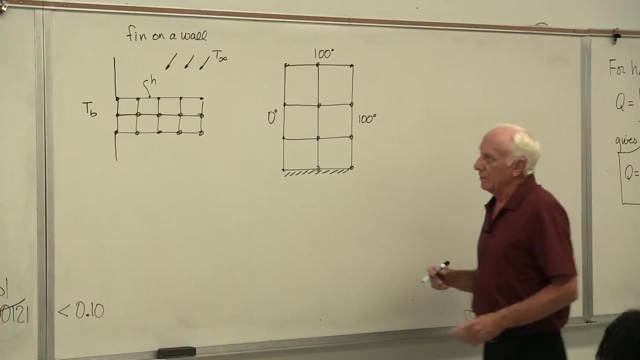 Okay, It looked like this: This side was adiabatic, perfectly insulated. This side was at 0 degrees. This side was at 100 degrees. This side was at 100 degrees. Okay, if somebody now we didn't do this at that time, if somebody we did, we did solve. 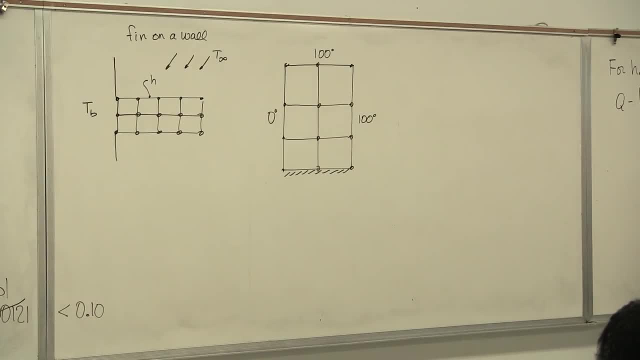 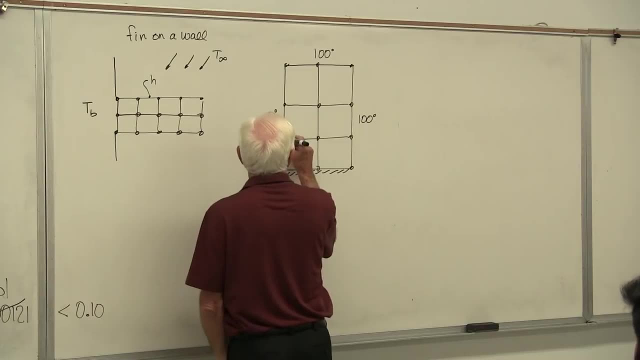 for the unknown temperature. there were three of them. okay, if you've been asked to find the heat transfer, here's one way you would do it. okay to find the heat transfer. number one is I'm going to find out how much heat is conducted into the zero degree face from. 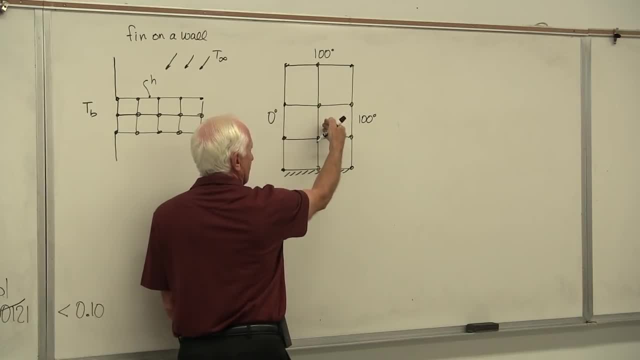 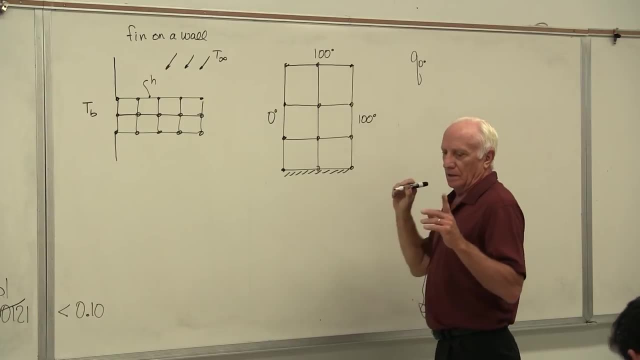 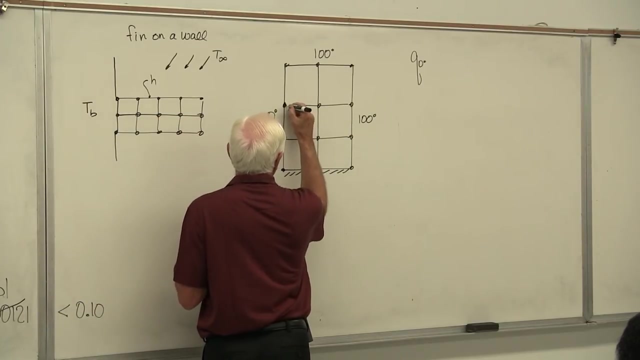 the inside. inside's hot. this is cold. heat's conducted from the inside to the zero degree face, Q, going out the zero degree face. look at the heat conducting rods that connect the surface to the interior are at different temperatures. temperature here: temperature. 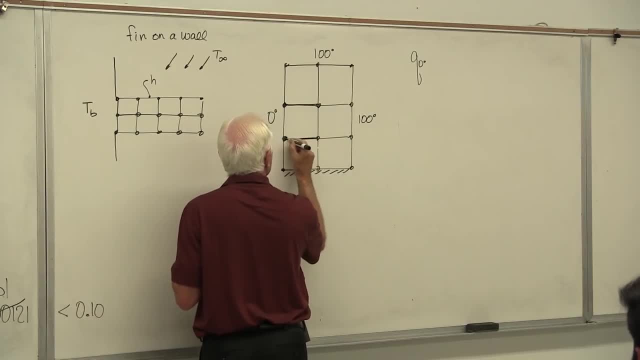 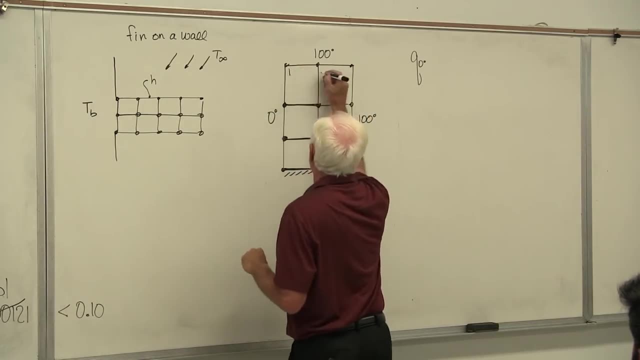 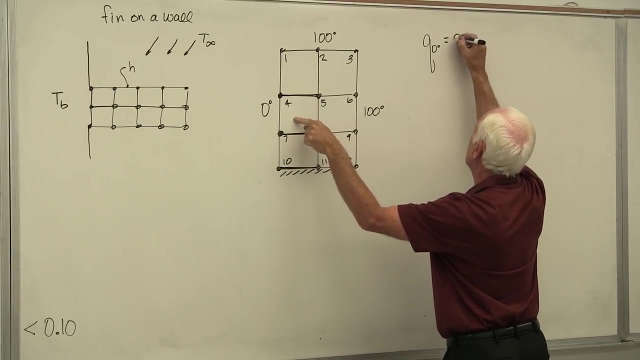 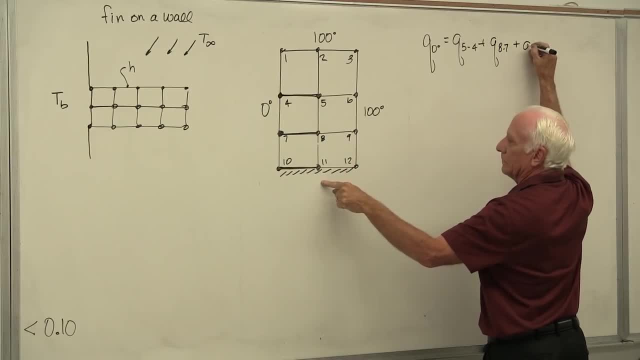 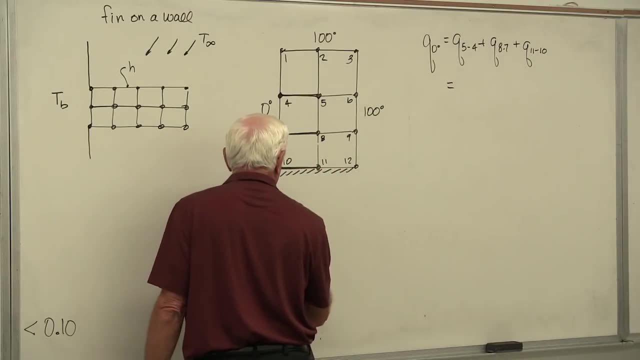 10,. use Fourier's law: Q equal KA, delta T, K, K is equal to three. so that's four, two, two, three, four, five, six, seven, eight, nine, 10,, 11 to 12.. 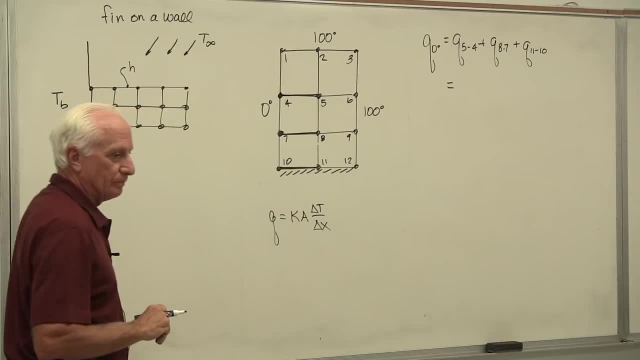 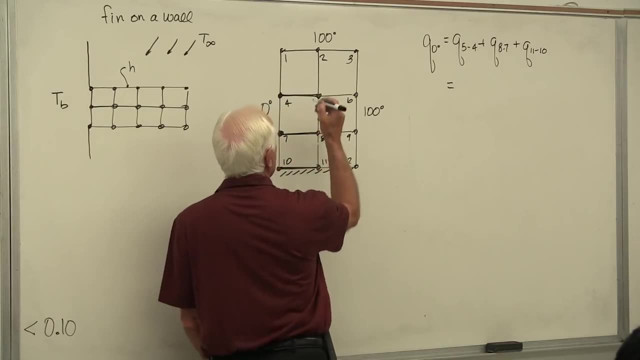 over delta X. It's a simple model. Okay, I'm going to go from 5 to 4.. If I do it by these finite elements, then this is the heat that goes from 5 to 4.. It's in this region, right here. 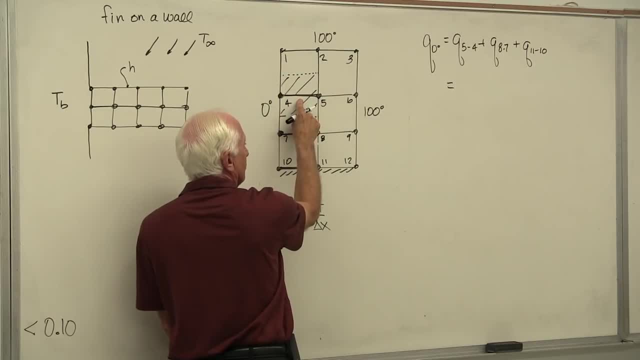 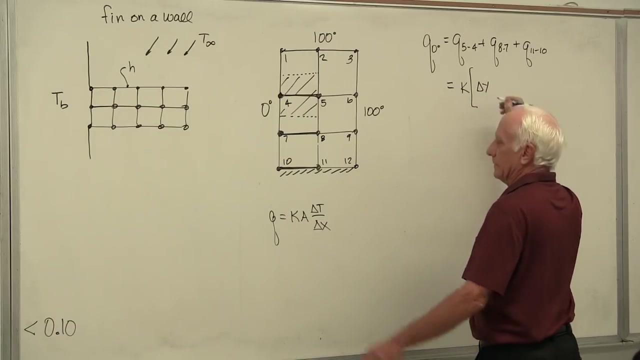 5 to 4, it goes out like that. That's the heat conducting rod replacing the actual material. What's the area the heat goes through My hand? delta Y times 1.. Okay, here it is. Here is delta Y times 1.. 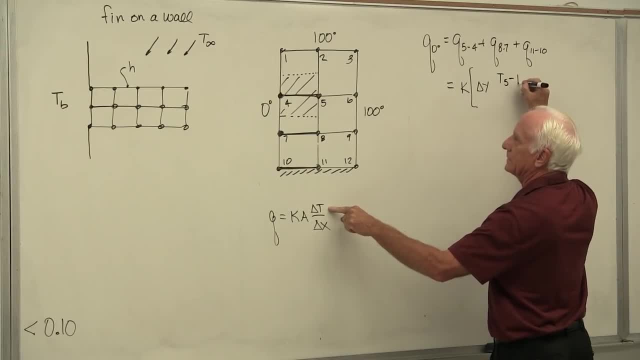 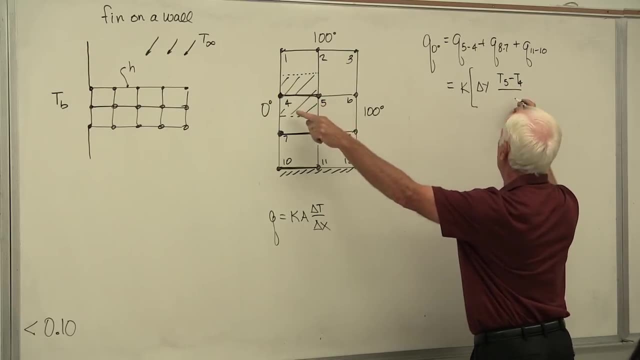 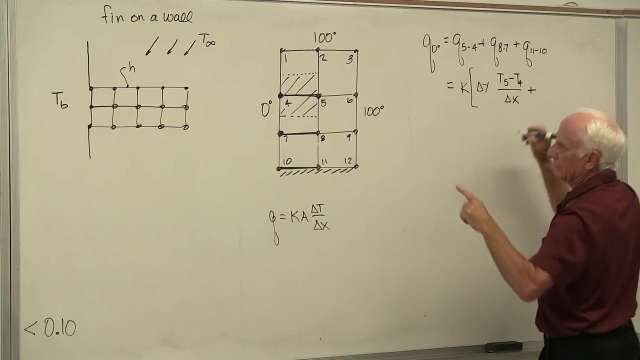 Temperature difference: hot minus cold, T5 minus T4. Divided by how far I moved, How far I moved from 5 to 4, delta X, The heat from 8 to 7.. I'll draw the picture again. 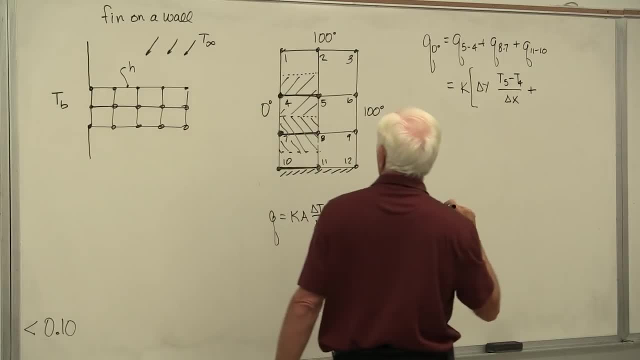 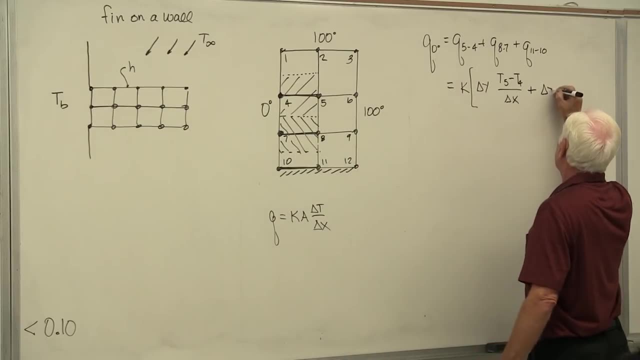 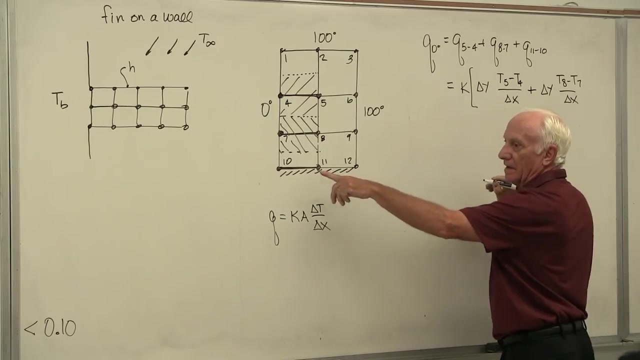 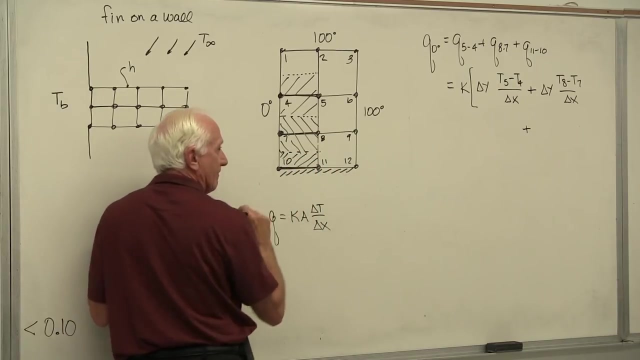 The area: delta Y times: 1. Temperature difference: 8 minus 7. Distance: I moved delta X plus 11 to 10, be careful, The area now is only half an area. Delta Y over: 2. Half an area. 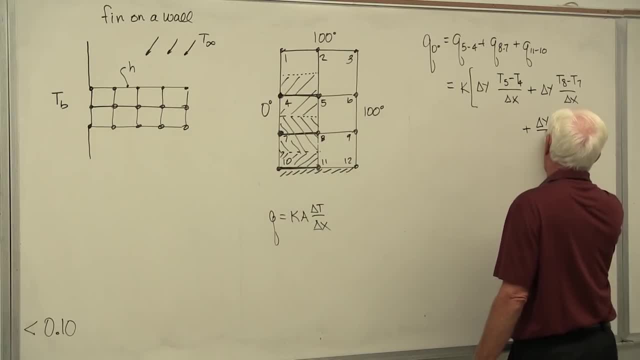 Delta Y over 2.. Hot temperature- T11.. Cold temperature- T10.. Distance: I moved delta X: Rectangular square grid Square grid. delta Y equal delta X. Gone gone, gone gone, I've got it. 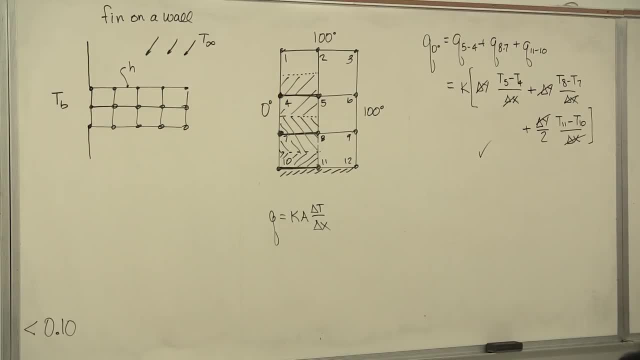 I've solved all the temperatures. in the previous problem, part C, I solved the temperatures. There they are Now. that's one way to do it. Of course, you can also do it this way. Here's the grid again. Here's the adiabatic wall. 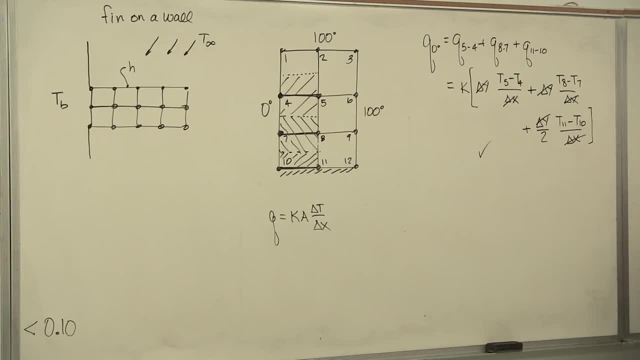 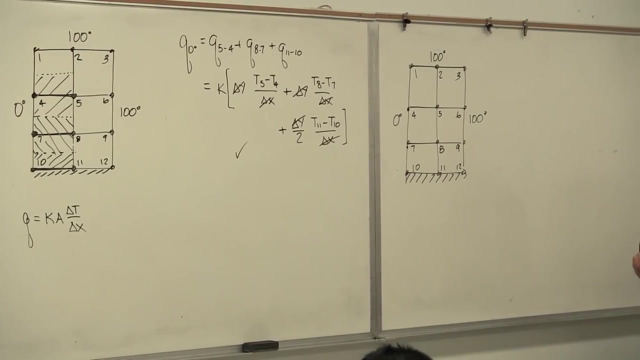 Here's the 0 degrees. 100 degrees. 100 degrees: That same heat transfer that goes out. the 0 degree face should equal the heat transfer that comes in the 100 degree face. Conservation of energy, chapter 1. Any storage. 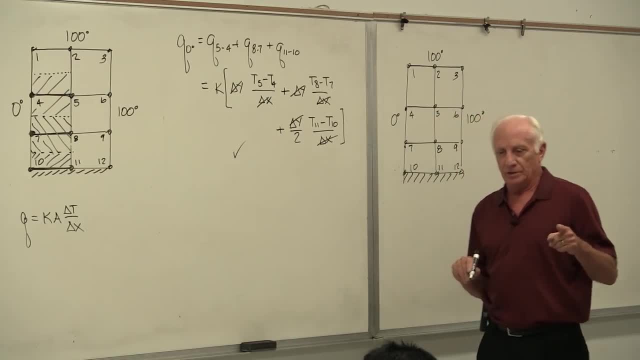 No, Any generation. No Conclusion: Q dot N E dot N E dot N E dot N. So all the heat that comes in from the 100 degree face should go out the left-hand side. We just found out an estimate of how much goes out the left-hand side. 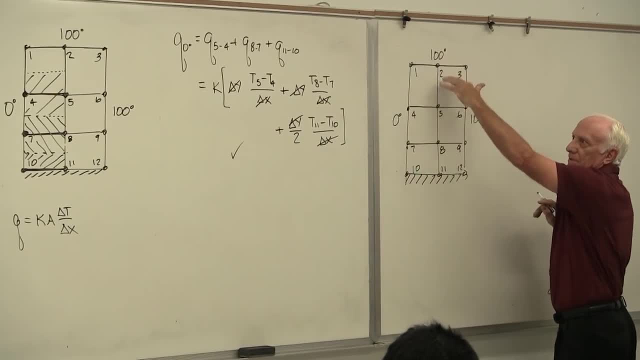 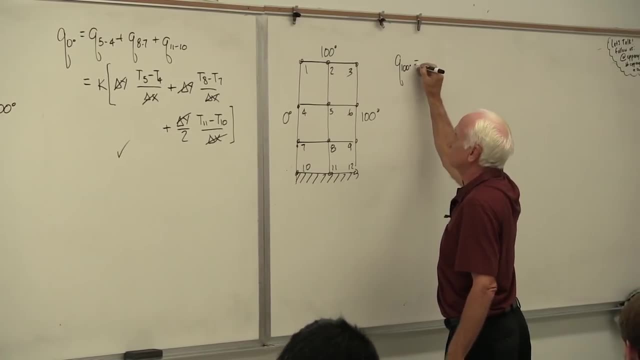 Now let's find out how much heat goes from the top into it and the right-hand side into it. Q into the body from the 100 degree face. Look at the heat conducting rods. Connect them together here from the 100 inside there. 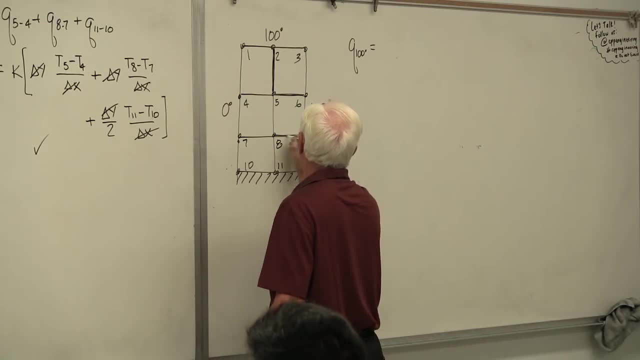 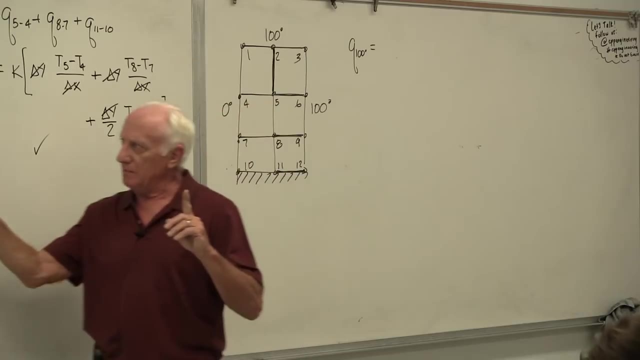 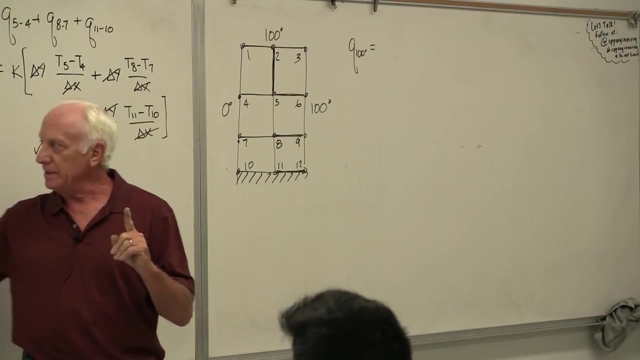 From the 100 inside. There's another one, Here's another one, Here's another one down here. By the way, don't think, because that's an adiabatic wall, that no heat flows from 11 to 10. Because I'll tell you that temperature there is 100.. 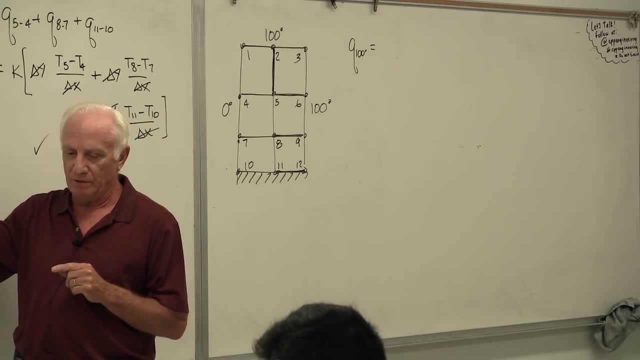 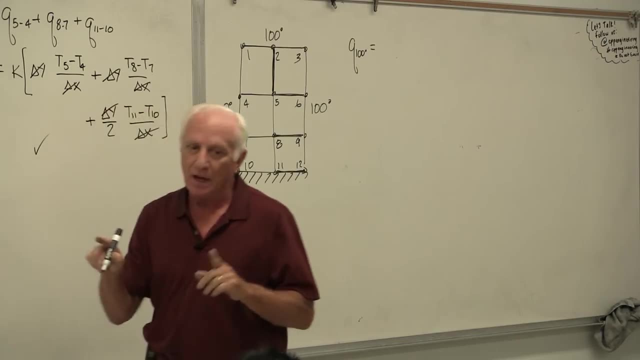 That temperature there is 0.. That temperature there is 51.6.. Definitely there's heat transfer from 51.6 to 0.. Oh yeah, There's heat transfer. There's no heat transfer normal to that direction. No. 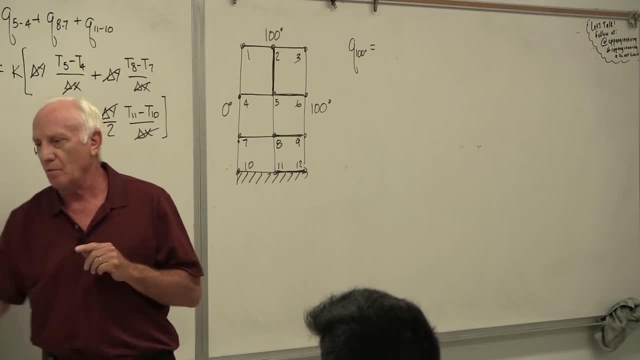 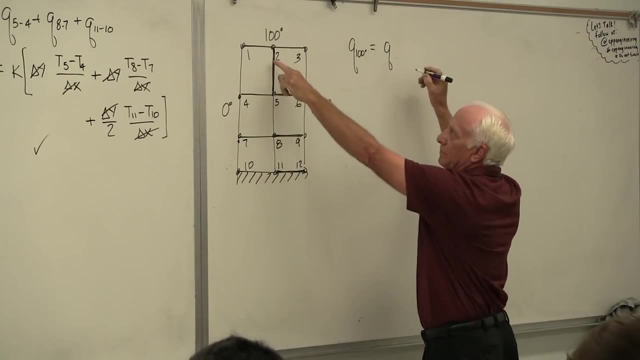 He's not transferred down that way, but he's transferred along the wall. Okay, Same as before. Q: hot temperature- T2,. cold temperature- T5.. 2 to 5.. 6 to 5.. 9 to 8.. 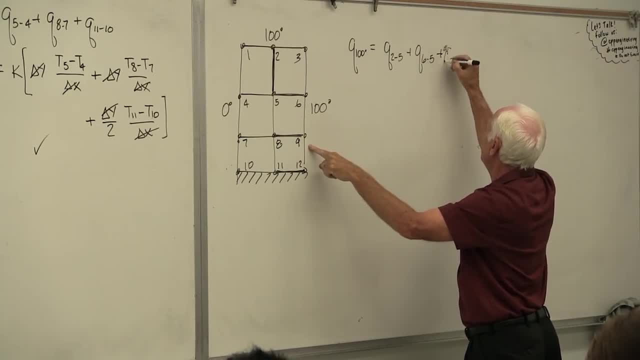 A cube: 5 to 6.. 6. 10 to 10.. 1 to 10.. 1 to 10.. 1 to 10.. 4 to 10.. 9 to 10.. 9 to 10.. 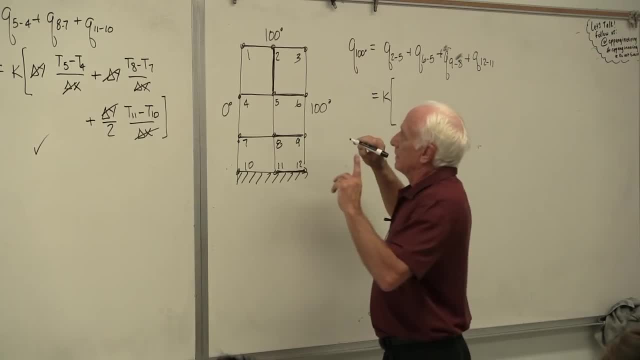 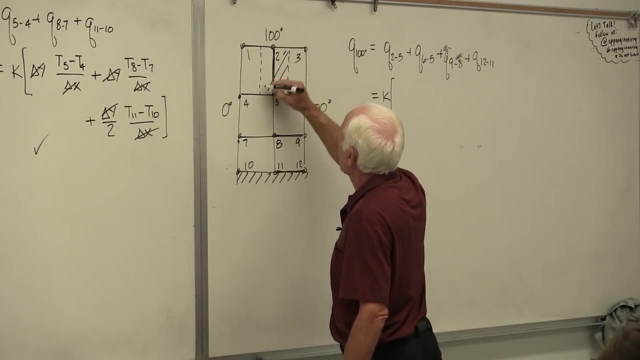 10 to 10.. 11 to 11.. 1 to 11.. Okay, Let's Okay. The heat conducting rod from 2 to 5 replaces what material? It replaces this material? What's the cross-sectional area? heat goes through. 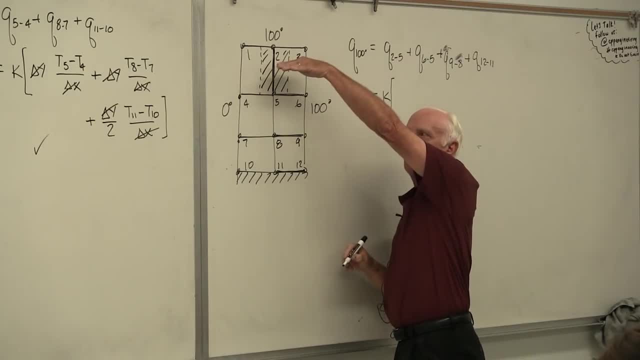 My hand. delta x times 1.. What's the cross central area if heat goes through? Delta x times 1.. What's the cross central area? That's my hand. delta x times 1.. What's the temperature difference: Hot to cold? 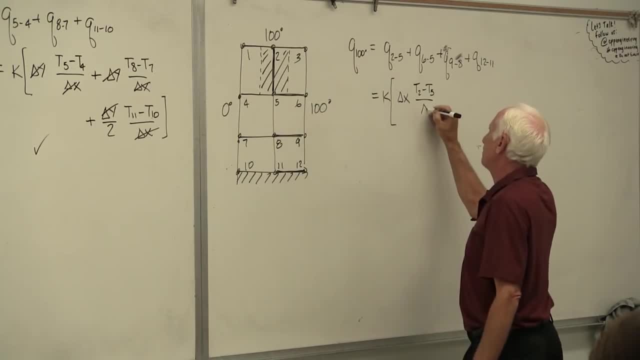 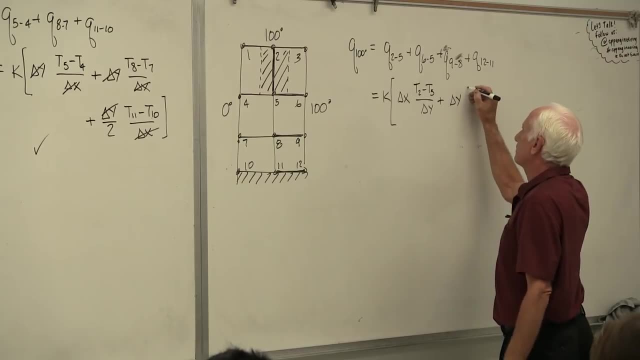 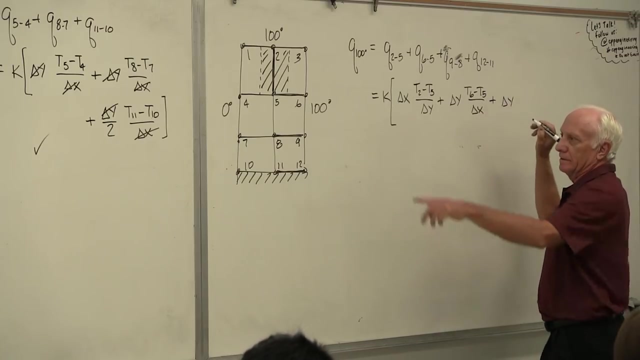 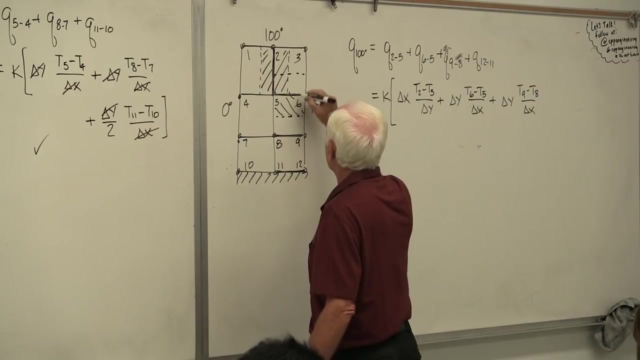 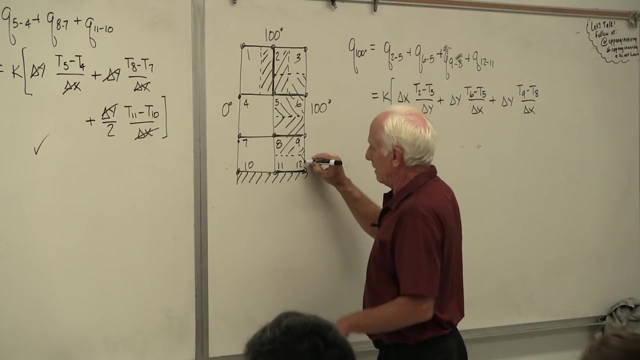 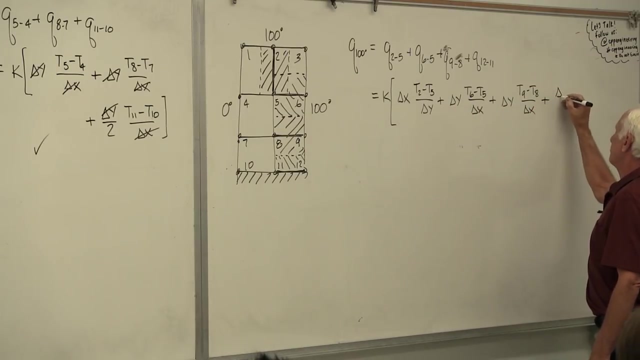 Divided by how far did the heat move? Delta Y Keep going. Six to five. Keep going. Nine to eight, Keep going. But watch out, because now the area is half again. Half delta Y over two. Keep going. Simplify it. 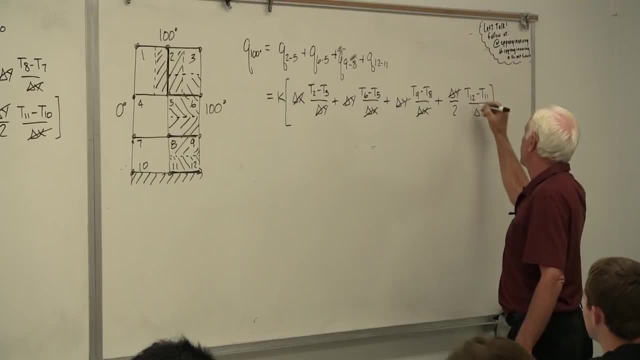 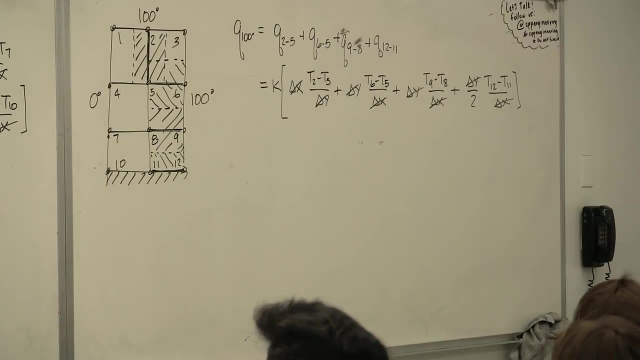 Square grid. You know the temperature. You've solved it already. Put the temperatures in. That's an estimate of how much heat goes out, comes in from the 100 degree face. Theoretically they should be the same. Conservation of energy. 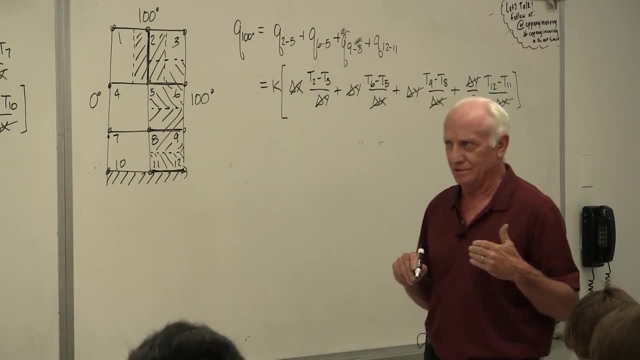 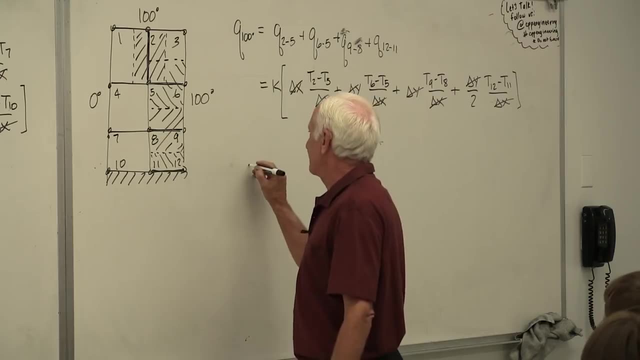 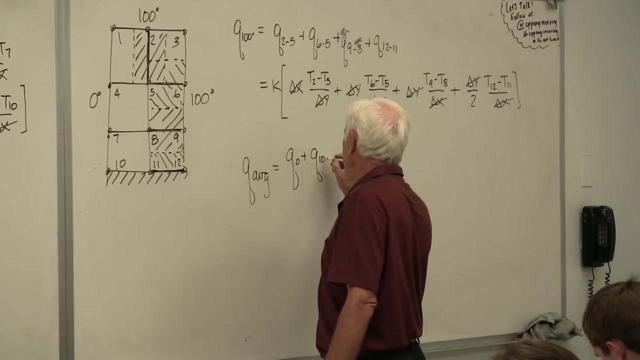 But they're not, of course, because this is a really coarse grid model. This is a really coarse grid model. Those two numbers won't match up, So one way to do it then is to take Q average, Q zero plus Q 100, divided by two. 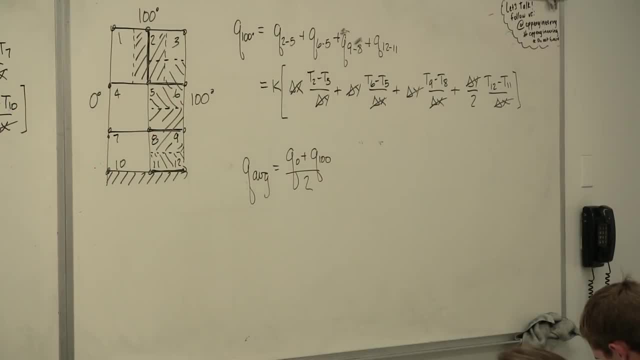 That would be a typical way to handle that. Okay, You say, well, can we make it better? Well, of course you can. Let's have the grid size. Have grid size Delta X. now is half Half O delta X. 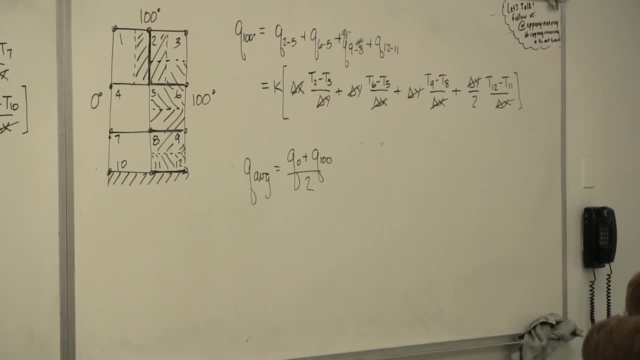 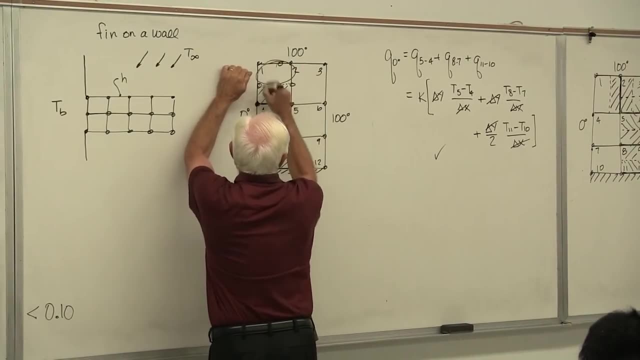 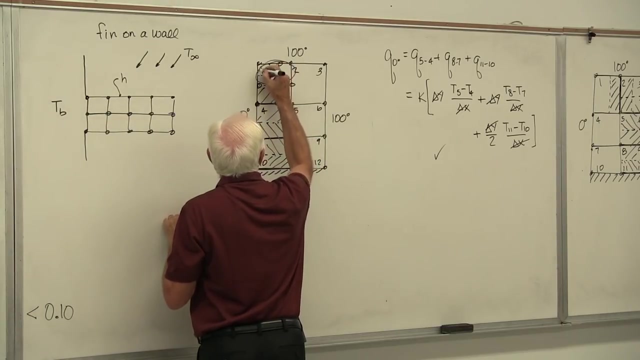 Delta Y is half O delta Y. So now you've got nodes here, here, here, here, here, here, Up here, you're ignoring this whole area. You're ignoring it If you make it half grid size now. you're ignoring that little piece. 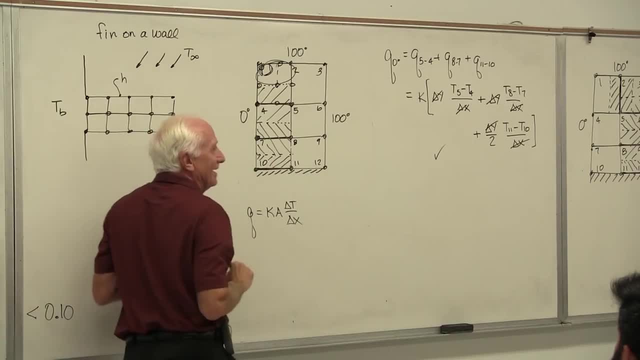 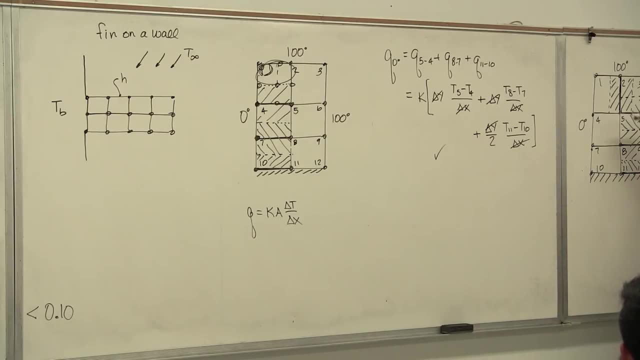 Have it again. You're ignoring a little piece up here. As you make the grid size finer and finer, you're going to eliminate that gray area Over here. where's the gray area? Did I account for this from 100 here? 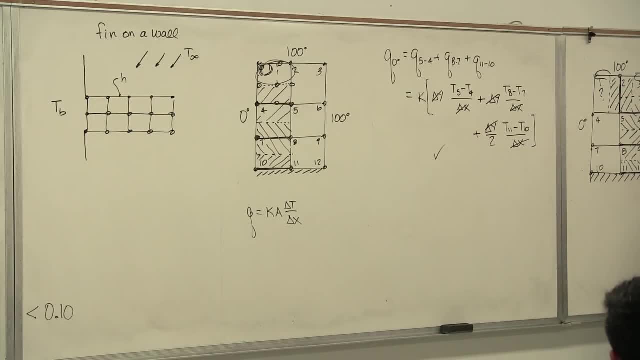 No, Did I account for this? 100 degrees here? No, As I make the grid size smaller, finer and finer, this piece up here gets smaller and smaller until it's almost negligible. Then this will approach this In the limit, as the grid size approaches infinitely small. 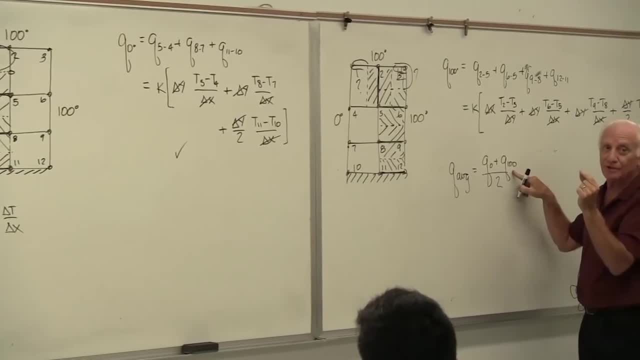 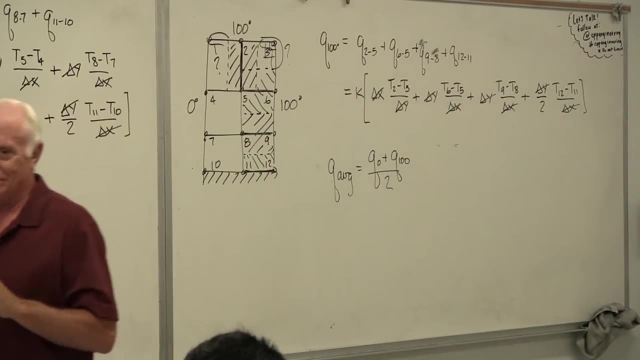 it's not that complicated: Delta X equal to 0,, delta Y equal to 0, you got it. Then you're going to find out, if you wait long enough, that they will be the same. But you know that's too much time. 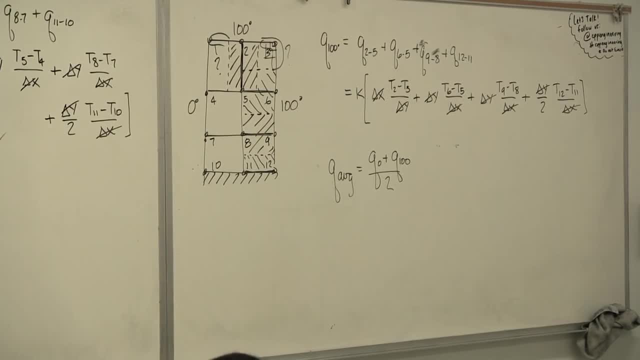 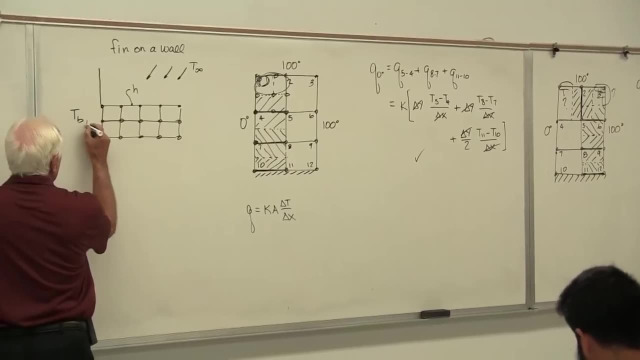 So, anyway, that's what you're going to do in part B of your problem here. okay, I'll tell you what it is here. If you've got a fin, the heat that comes in here by conduction through the base, all the heat that comes. 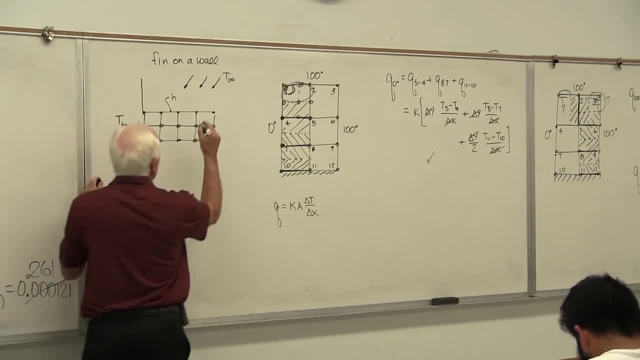 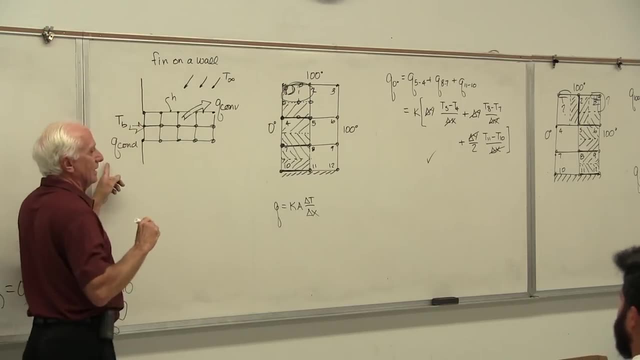 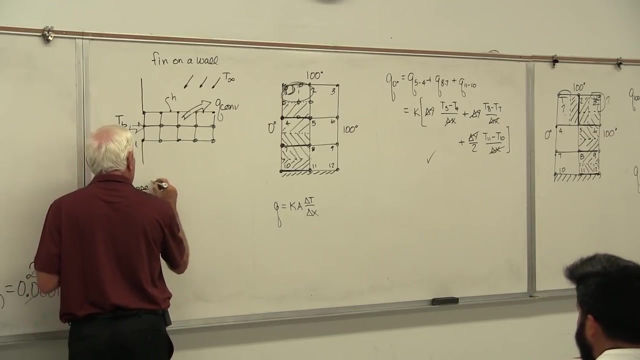 into the base by conduction, goes into the fin. all that heat is carried out by convection. All the heat that comes through the base is carried out by convection. So you're going to find first of all Q, base equal. 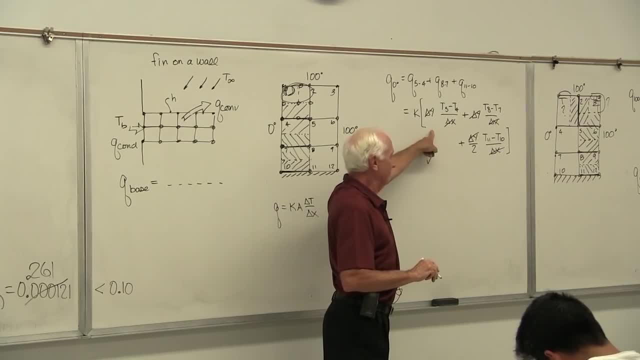 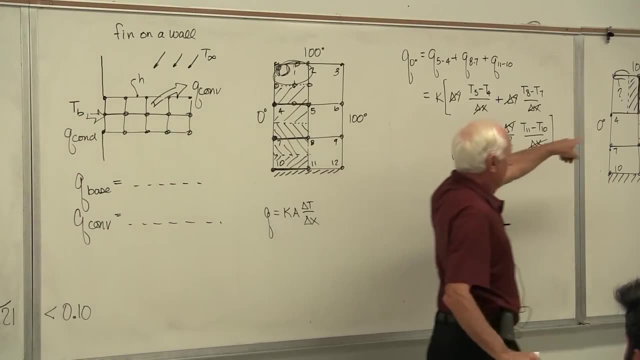 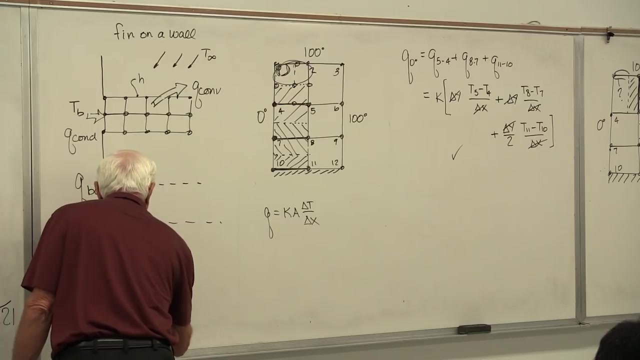 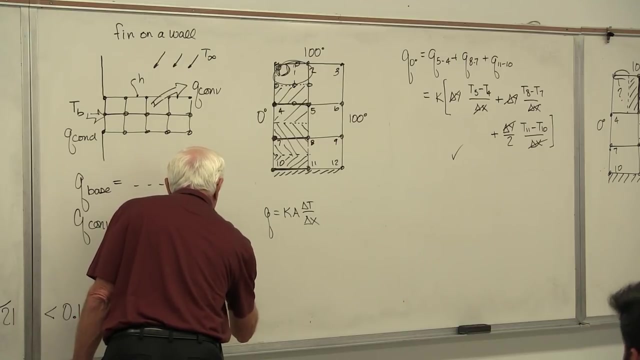 you're going to find out Q convection- I like that, Okay- And then you're going to average them because they won't be equal, because the grid size is not very fine. So if you want to find out how much heat goes in the base,